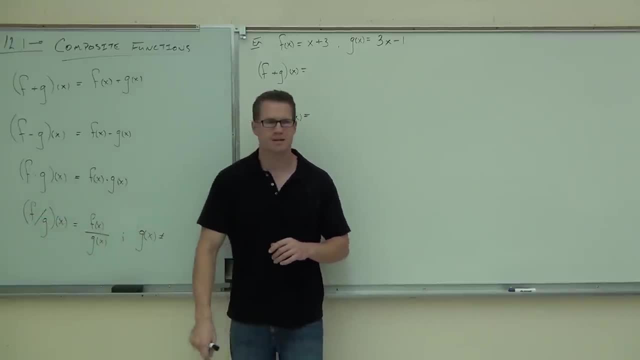 by g of x. By the way, I said one thing over here. I haven't completed this statement. What can't g of x be equal to? Why You can't ever divide by zero. So the only thing that g of x can't be equal to is zero. Are you with me on that? You can't have a fraction. 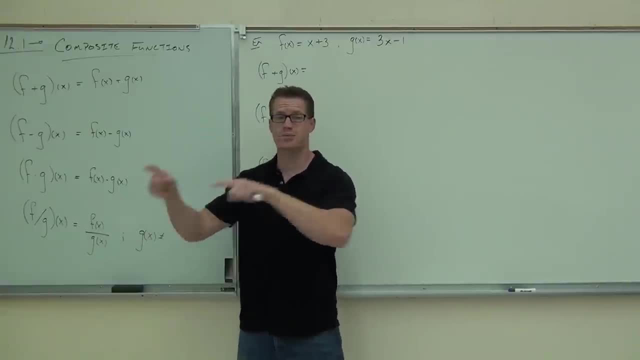 over zero. That doesn't make sense. So this is going to go back to our domain problems. Do you remember those domain issues from like a long time ago? We'd say: the denominator can't be equal to zero. We set it not equal to zero and we solve it. Do you remember? 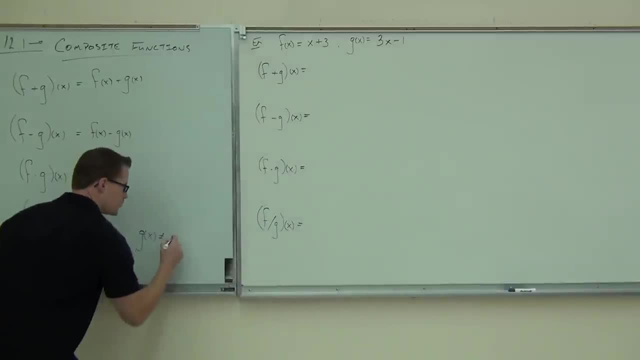 that It's not a hard thing. It's just one other thing we've got to deal with for this one particular issue right here. So g of x can't be equal to zero. Now I've got a simple example. Let's see if we can. 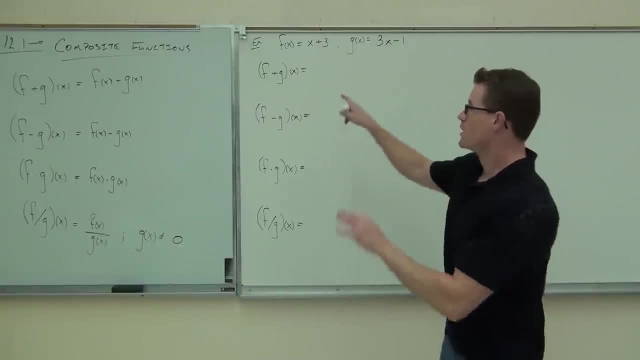 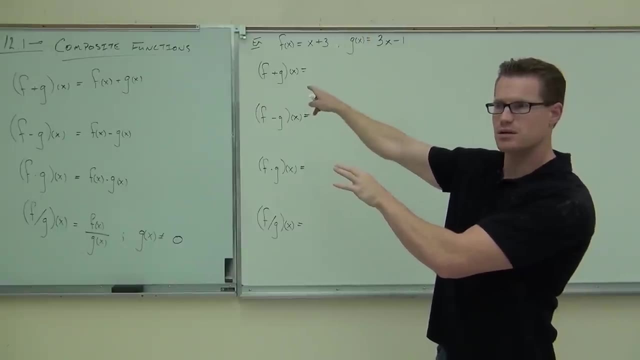 go through that example and figure this stuff out. So, firstly, we're going to try to do all four of these operations with those two functions, f of x and g of x. What is f of x, please? x plus g of x. 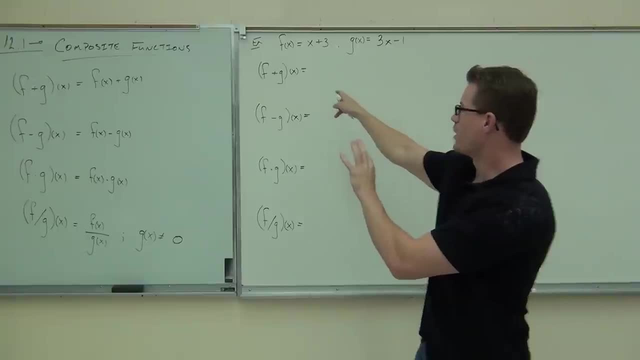 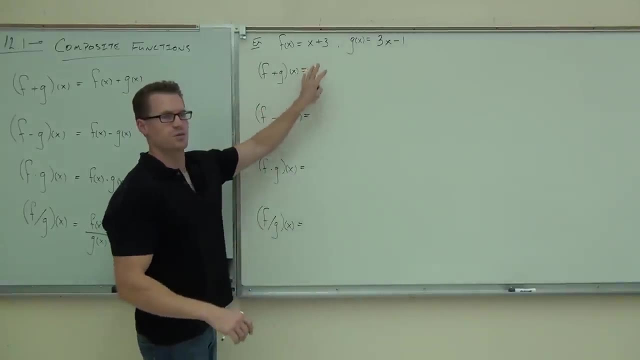 Good, What's g of x, g of x, g of x? Great, And I want f plus g of x. So this just says: refer back to your functions, add them together. f plus g of x would be this one. I'm going to see if you can figure out. 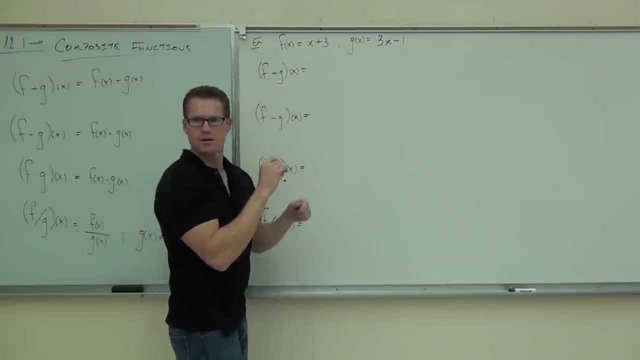 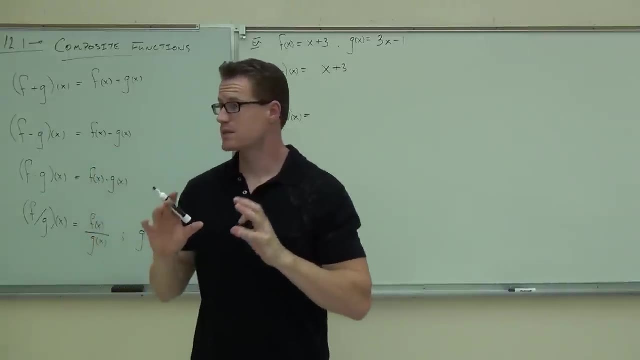 the rest of them. But f plus g of x would be what's the first function then? x plus g of x. So I'm going to write x plus 3.. I'm going to write it in parentheses because it's a function itself. OK, It's saying: this is where it came from. I've got x plus 3 as f of x. 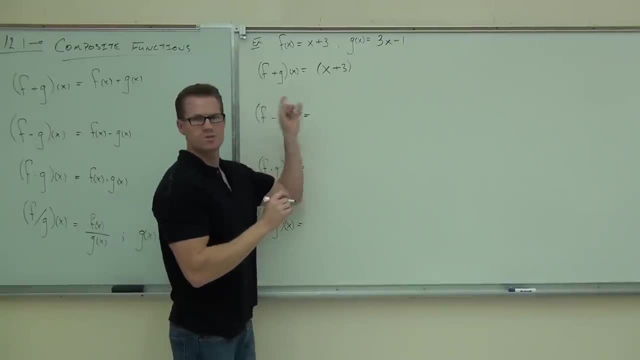 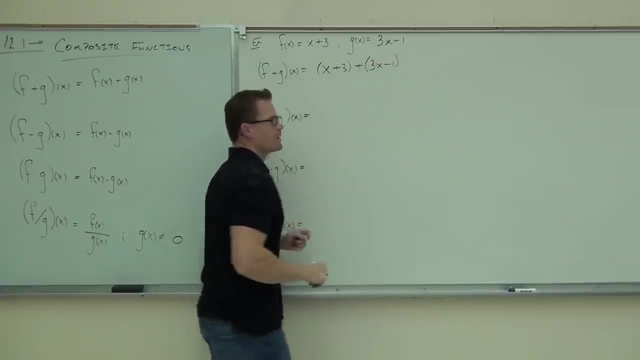 Are you with me on that? And then, what operation am I doing? Addition, subtraction, multiplication, division, Addition, Addition. I'm adding. what function? 3x minus 1.. Raise your hand if you see where those things come from. Good. So f plus g of x says hey. 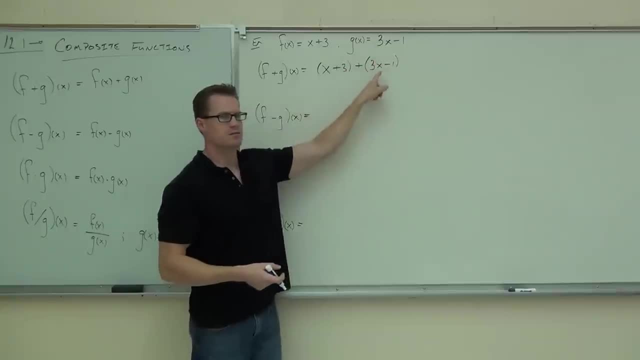 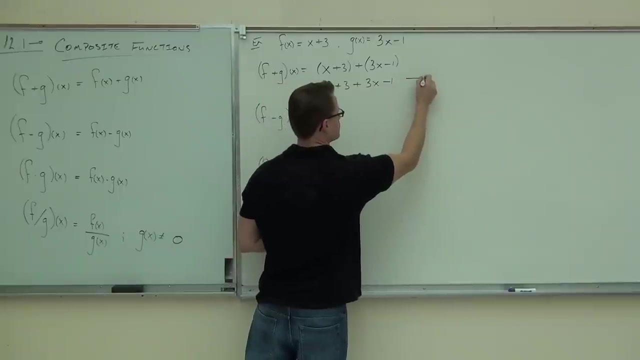 take f of x, add g of x. I can combine some like terms. It's addition. Do I need to change any signs? So essentially I can just drop the parentheses, combine like terms And that's going to give me what's x plus 3 plus 3x minus 1?? Do the combining like terms? 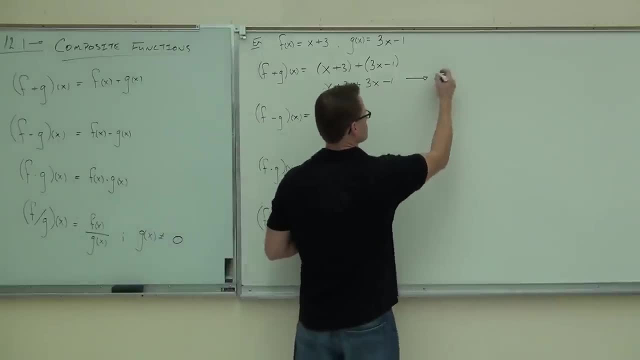 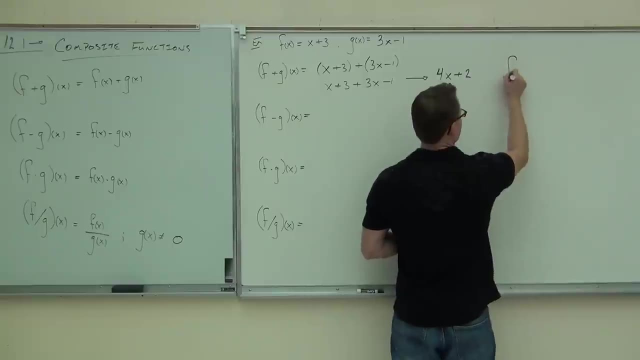 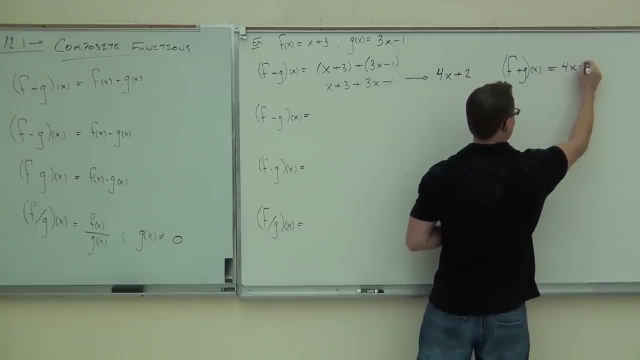 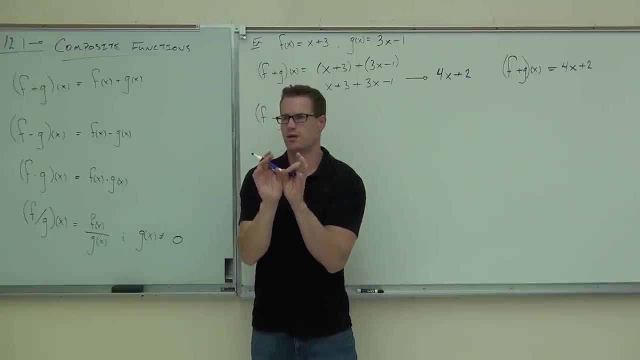 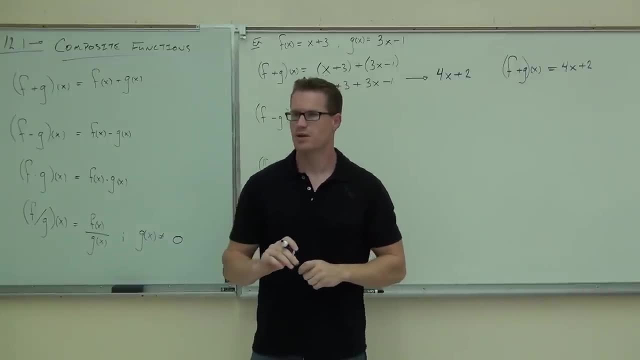 That's the function you get when you add those two functions together. nod your head if you're OK with that. You don't need to simplify it. G of X. First thing, is it important to put the F first in this case? 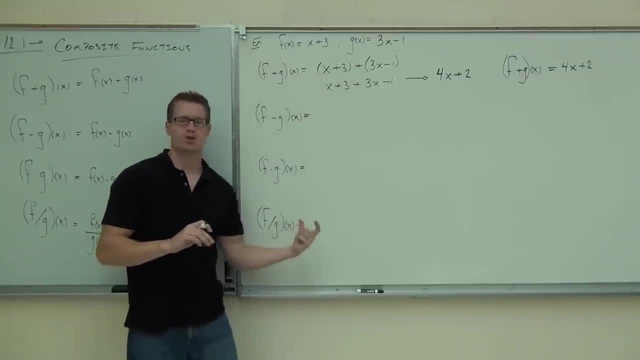 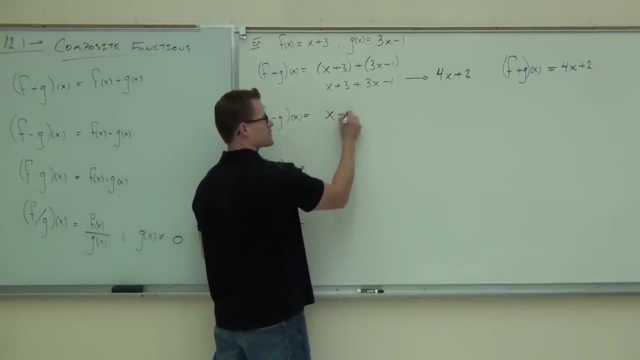 Yeah, addition really doesn't care right, Because it's commutative, But subtraction and division are not commutative, So it depends on what comes first. So what has to absolutely come first? Yeah, because that's our F, I'm going to put it in parentheses. You're going to see why the parentheses are. 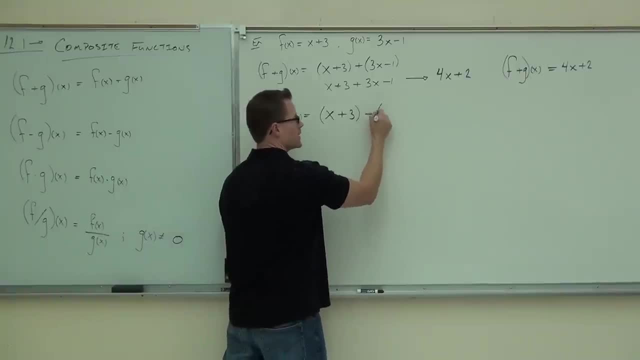 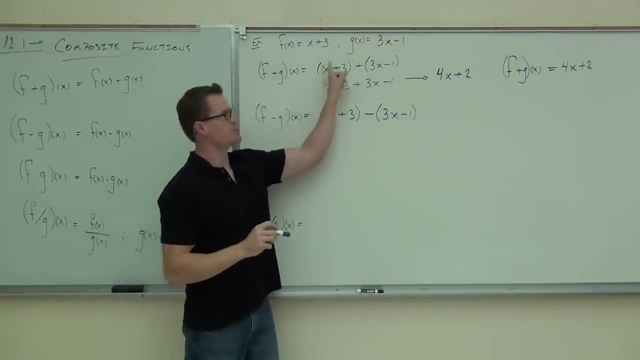 important And what's going to come next, Minus what? Hey, by the way, look over here at the board- Am I supposed to distribute these? No, When do you distribute? Yeah, not addition, subtraction. We don't want to distribute those, We don't want to FOIL those is what I mean. Now, what's? 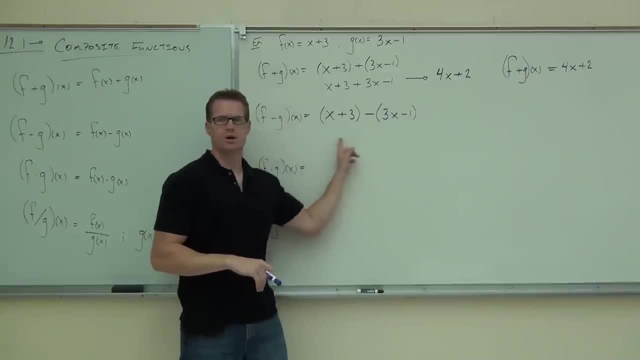 going to happen with this expression here? What do I need to do to this to get rid of those parentheses? Yeah, we're going to multiply that negative inside, So the X plus 3 stays the same. However, what am I going to get? 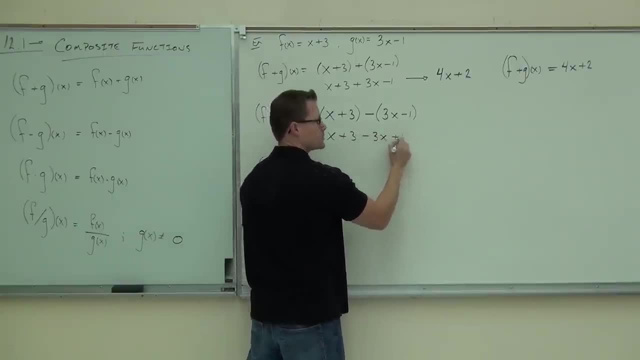 next: Ah, plus 1.. Do you see where the plus 1 is coming from? You all see where it's coming from. That's important to have those parentheses, right? Because if you don't have those parentheses, if you didn't have these up here, you'd have a minus 1 still. 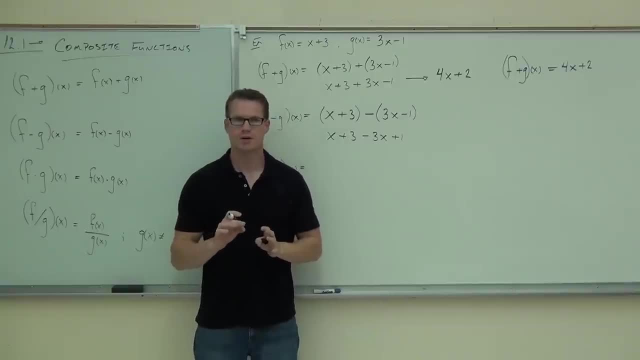 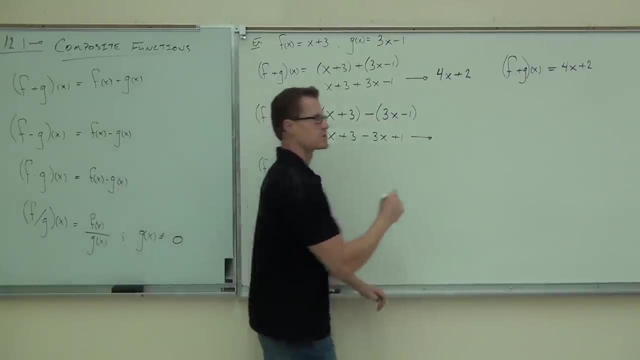 and that's going to give you a different constant at the end of your expression. You okay, so far with this. Okay, so when we combine these, do your combine like terms? what are you going to get when you combine like terms: 2X, 4X? 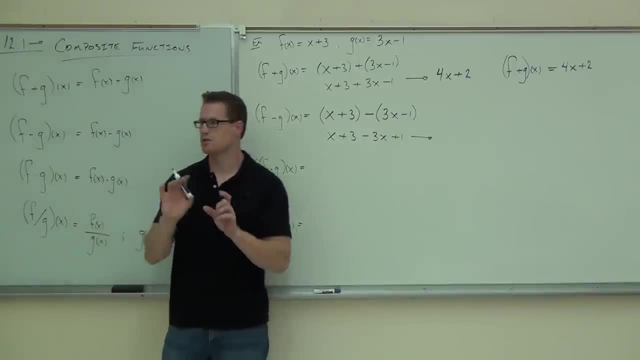 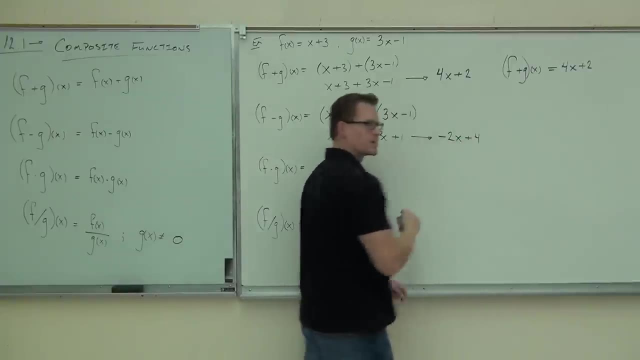 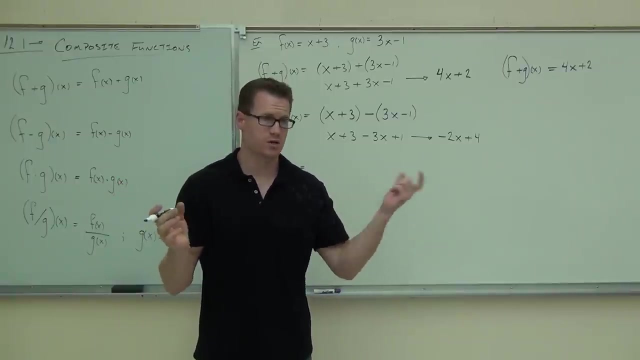 Negative 2X. What are you going to do with the sign Negative 2X and what was that one Plus 4.. So the key on these things: you've already added functions together. You just did them without calling them functions. You've already done this. combine like terms. You've already. 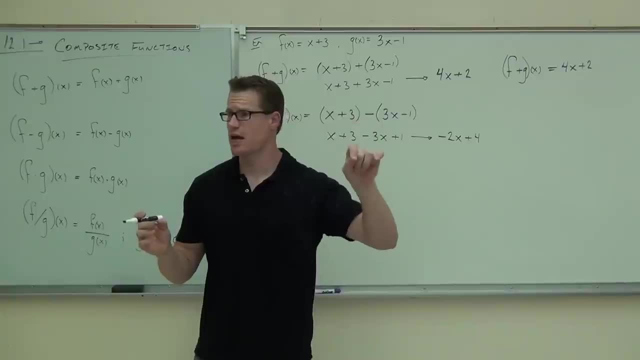 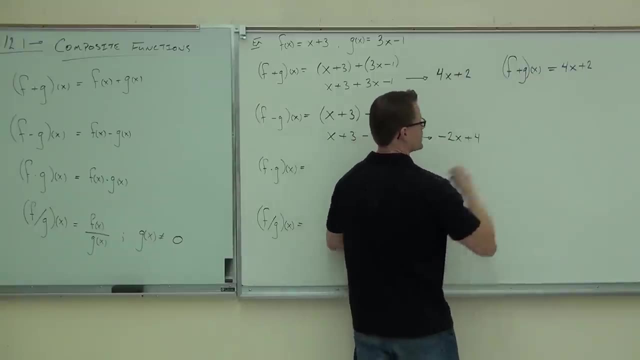 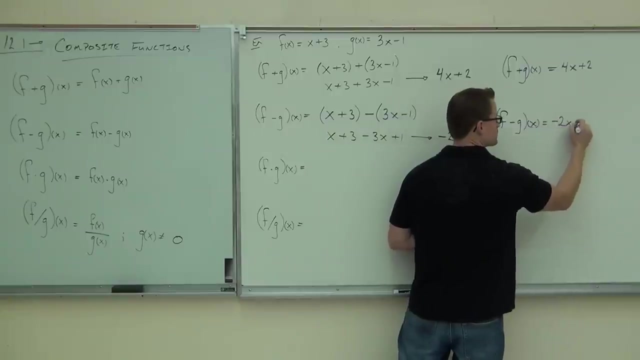 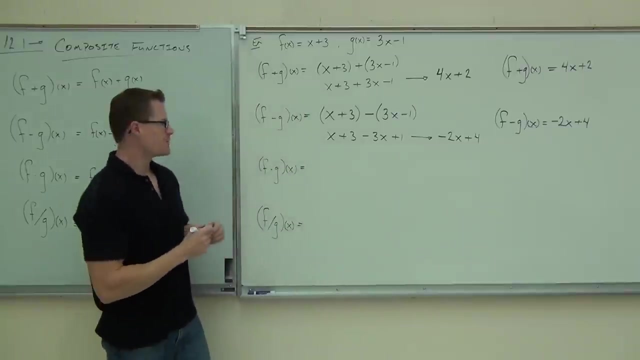 subtracted them. It's called combine like terms. You just have to make sure about your signs, right, Make sure your signs are correct. So we say F minus G of X, in this case is negative, 2X plus 4.. Let's see what F times G of X does. We have F times G of X. It says: take your. 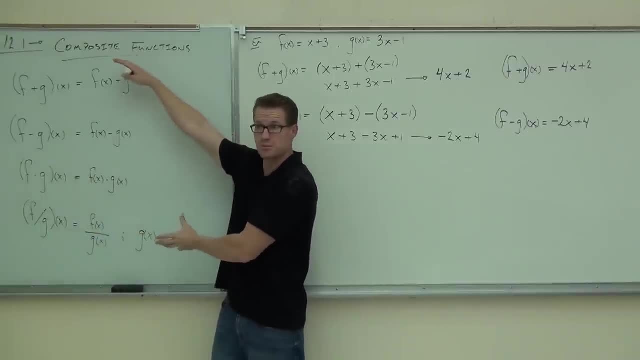 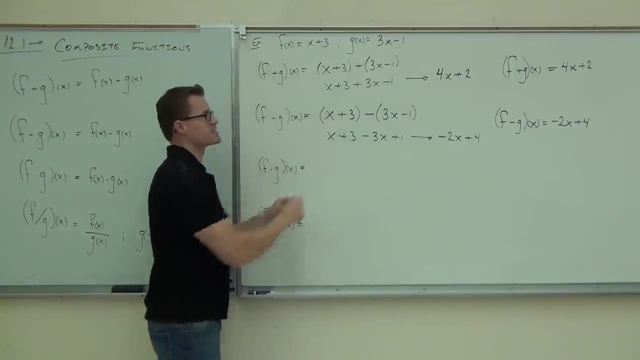 F of X, multiply it by your G of X. That's what these rules say. This is all it says. It's a pretty simple idea. It says: add your functions, subtract your functions, multiply your functions and divide your functions. That's really it. We're just practicing that over here. So we've already. 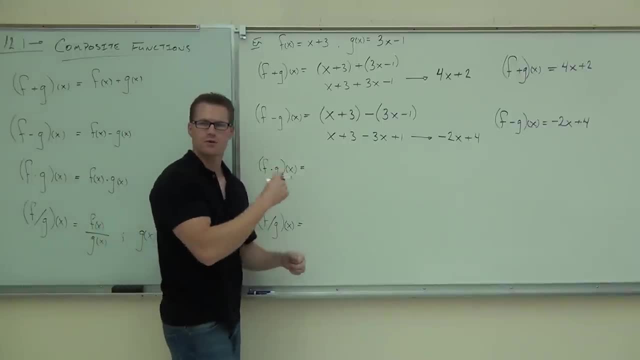 added, we've subtracted. Now let's see if we can multiply our functions. What's the first function we're going to have here? X plus 3.. Okay, that's in parentheses. And what am I doing? Multiply, Okay, and what am I going to multiply by? 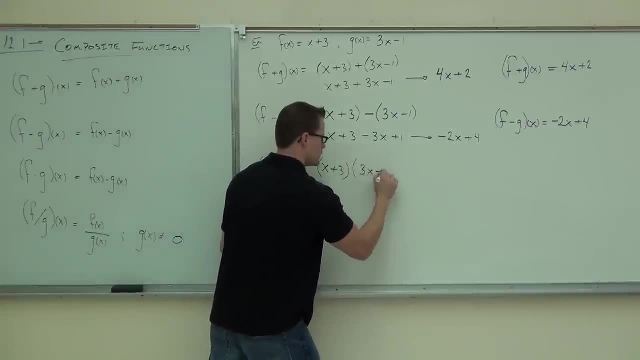 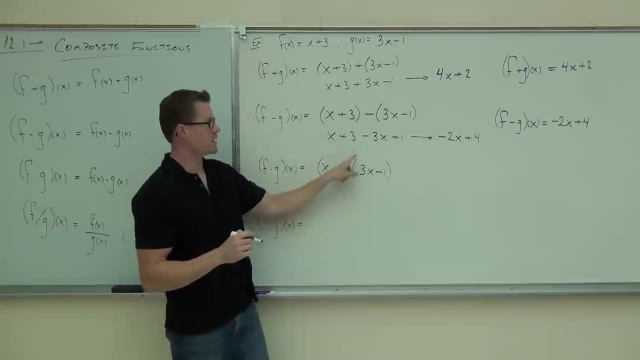 3X minus 2.. Good Now, of course, when I don't have an operation in between them. so it looks similar to these, except the operation is different. This is plus, this is minus, and there's nothing That. 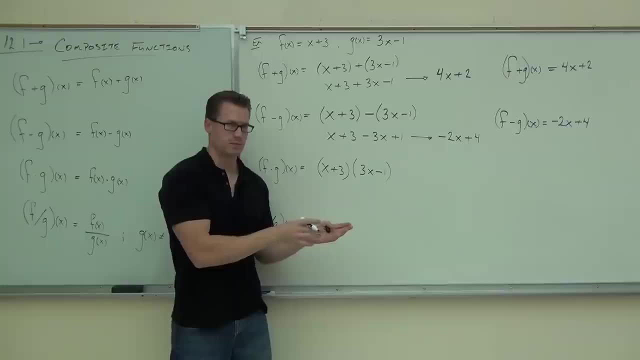 means we're multiplying. How do I get rid of those parentheses when I'm multiplying? Here's where I distribute. So if we were to distribute, can you tell me the first thing that I'm going to get, please? 3. Good, I like the X squared. Awesome, Keep going. 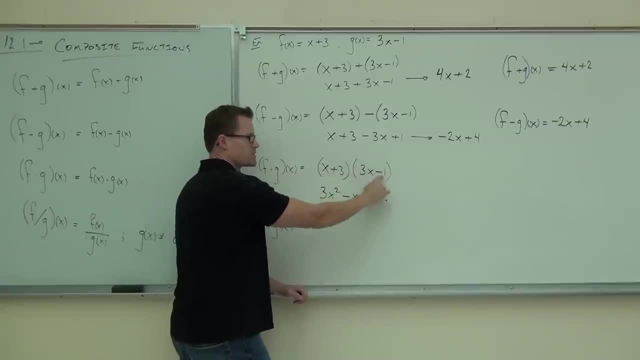 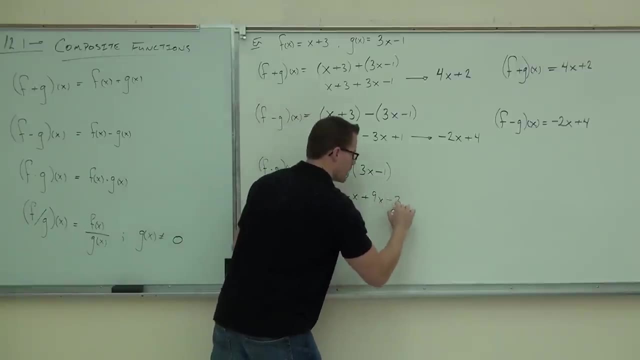 Minus X. Minus X because we're doing X times negative. 1. We're getting minus X. And then what? Plus minus X? Good, We got 3 times 3X, and then Minus 3.. Ah, minus 3.. Once we combine some like terms, we'll get 3X squared. I know that. What's the next thing we'll get? 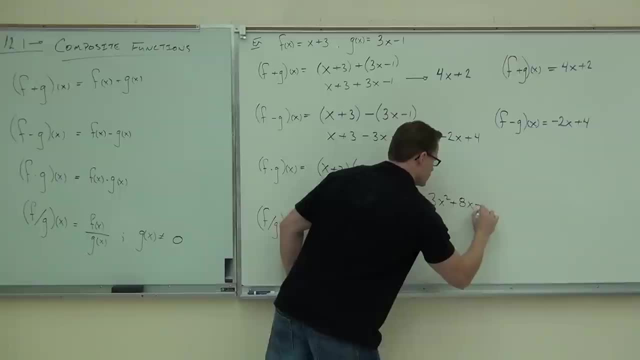 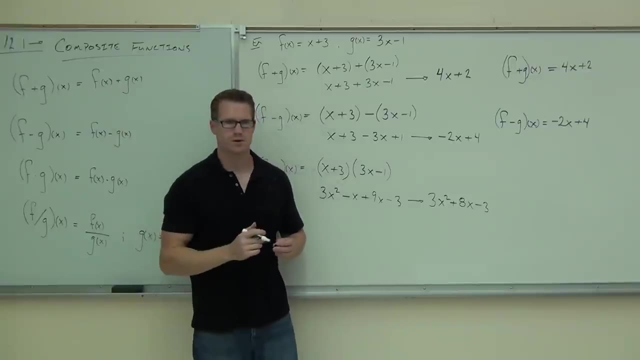 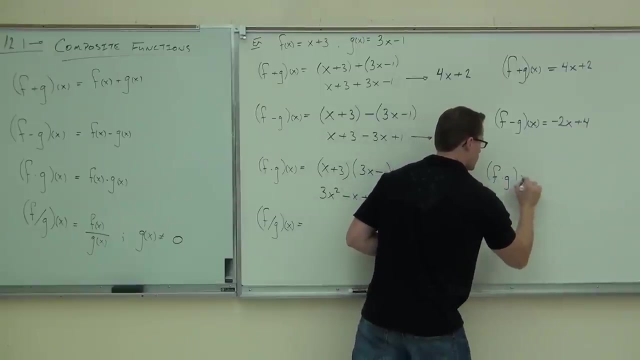 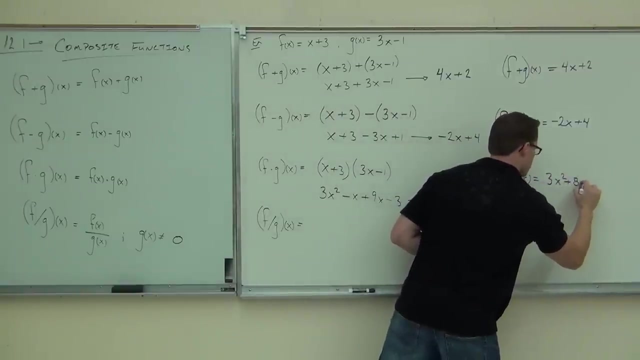 Plus 3 times minus 2.. Cool, That's as far as I can go. I don't need you to factor. All we're doing right here is doing these operations with these two functions. So we'd say, in this case, that F times G of X is well that expression that we just created. 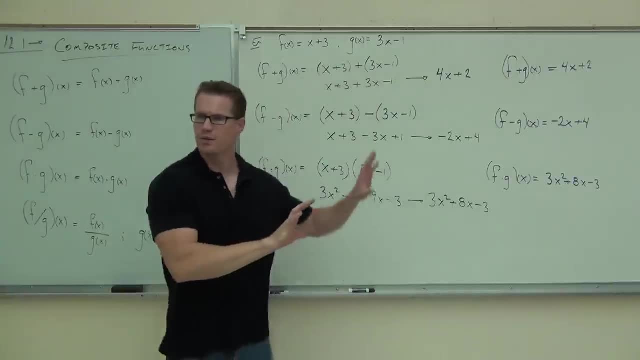 And let's do the last one. The last one is F over G of X. By the way, are you okay with these three examples so far? I don't know if you are Okay so far. you've done all this right. You've done all this before. 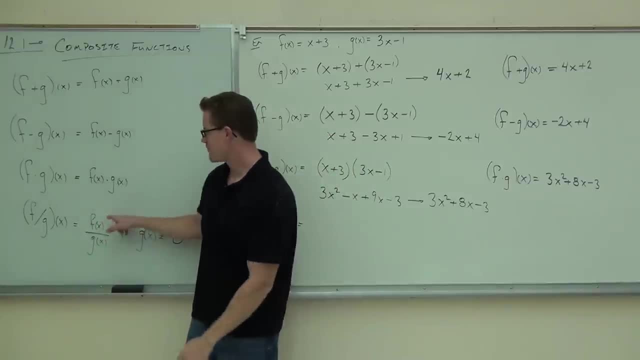 F over G of X, F over G of X says you're just going to take F of X, put it on top of G of X. That's it. So in this one this might be the easiest one for you to do. 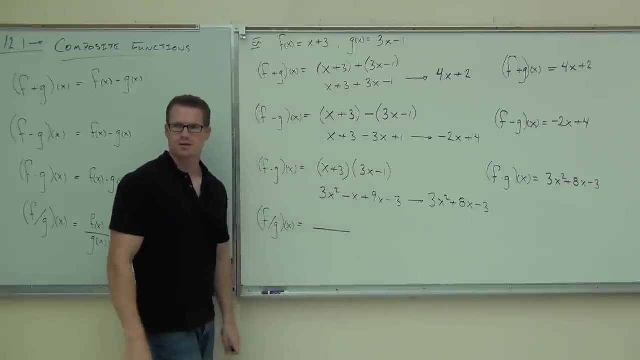 What's going to go on the numerator, F of X or G of X, F of X. Is it important to put that one on the numerator? It really is, It really is. So we're going to have X plus 3.. On the denominator, we'll have G of X, 3X minus 1.. Hey, can I cross out the X's? 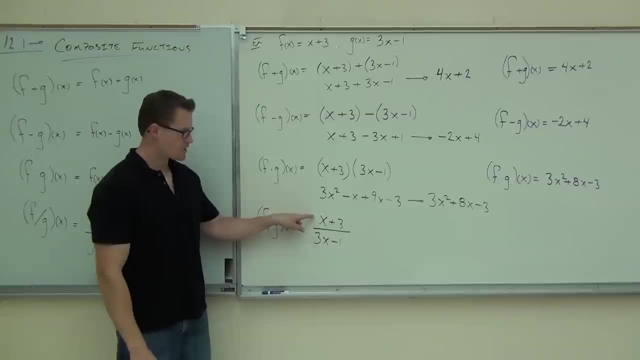 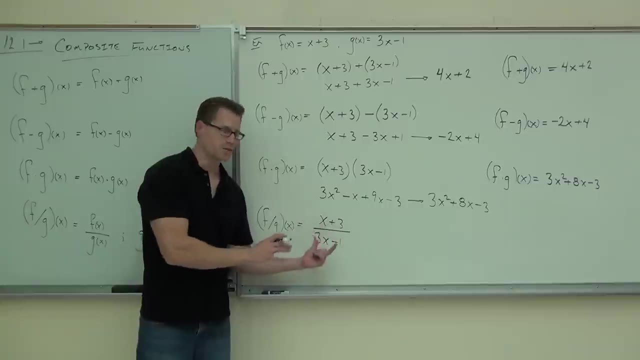 No, Can I cross out the 3's? No, Even if there were 3 here, Even if there were 3 here, could I cross out the 3's? No? No, because they're all connected by addition and subtraction, right. So unless you can factor these, which you can't, you can't factor either one of those. then you're essentially done. 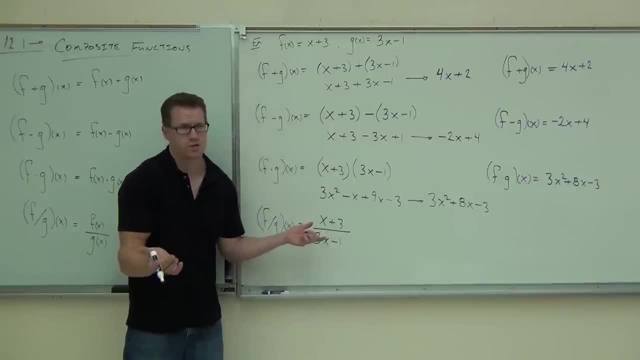 You can't do anything with that. This is the expression. It's a rational function. Now, the only other thing that you've got to do, you've got to give me the domain. So, right now, this is it. This is F over G of X. It's already listed for you. No work at all. right, That's kind of cool. 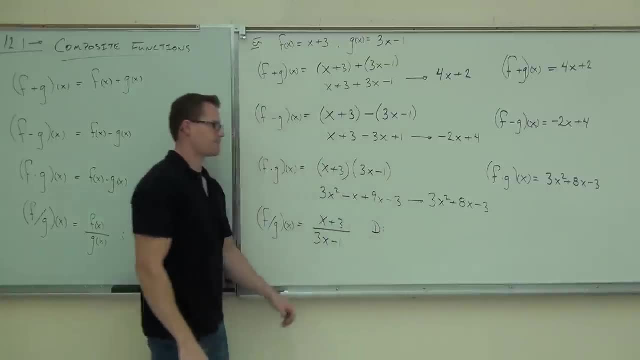 But you do have to state the domain. And here's how you state the domain, if you don't remember this. The domain says: can the numerator be equal to 0?? A numerator? Yes, Absolutely. The top of a fraction, no problem. How about the bottom of a fraction? 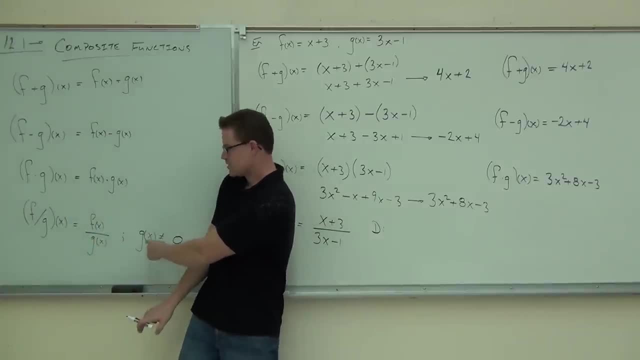 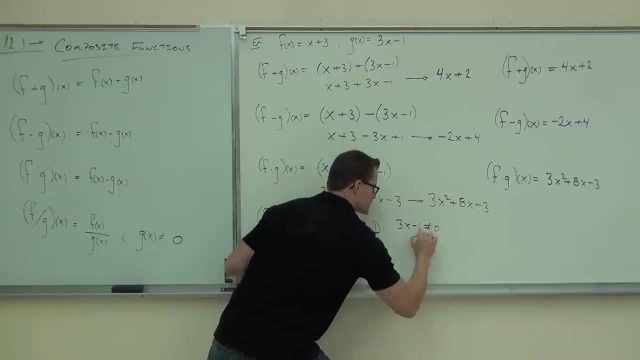 No. And so what the domain said? this is what this says right here: G of X can't equal 0. It says that you're going to set your denominator not equal to 0.. Do you remember doing that? No, We'd say, oh, look here. 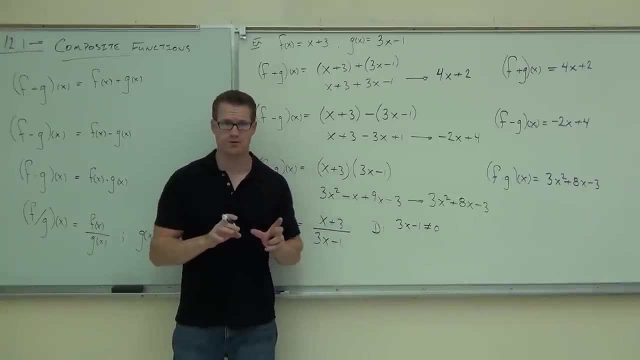 Set it not equal to 0. Because that's the one thing we cannot have it equal to. You follow me, And then you solve it like any other equation. How would you solve that one? Add 1, and then you would do what. 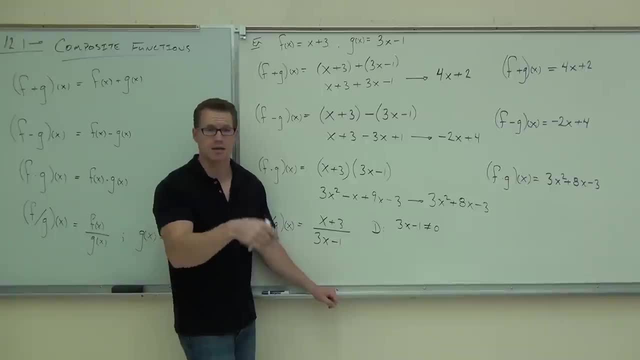 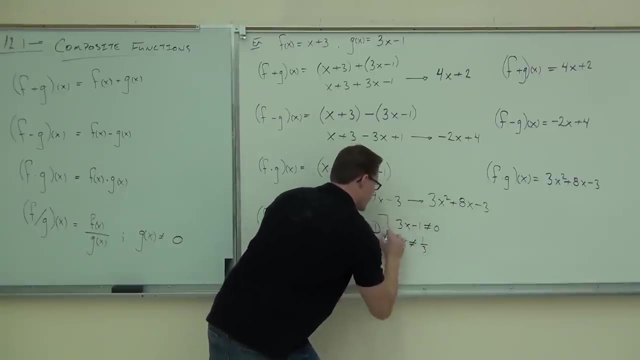 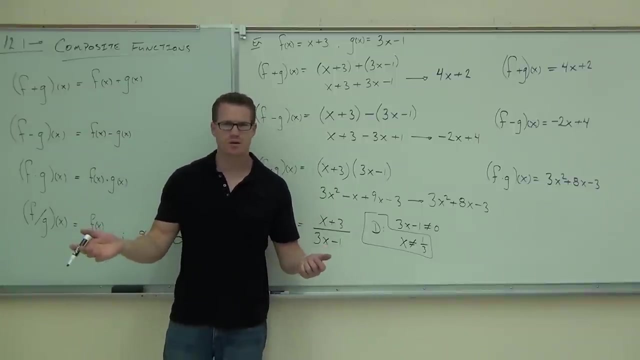 So we're going to get X equals, or actually X is not equal to 1 third. That right, there is your domain. It says X will be all real numbers, except except which number: 1 third. Why can't we have think about it? 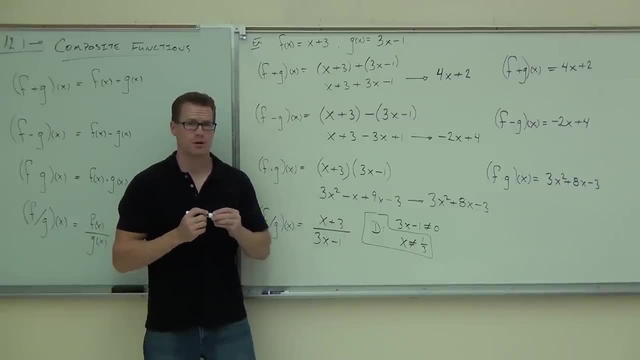 Why can't we have 1 third here? It's going to turn that 3 into a 1.. So 1 minus 1 equals 0.. Ah, So the only number in the world that if I plug in here that makes it bad is if I plug. 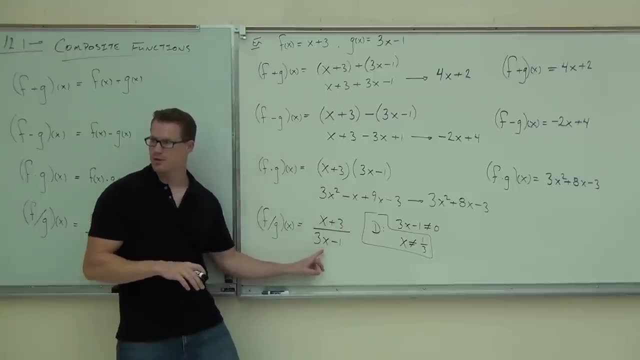 in 1. third, Are you with me? Anything else is going to work. 0 is going to work because I have 0 minus 1.. It's negative 1. It's fine, But negative 3 would work because I have 0 up here but not down here. 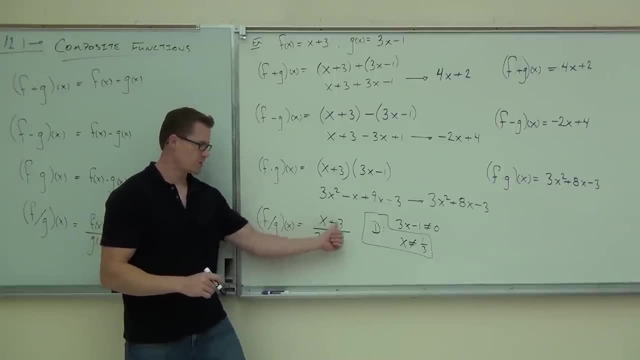 That's fine. But if I plug in 1 third, I get 3 times 1 third, That's 1.. Minus 1 would be 0. And I can't have 0 in the bottom of a fraction. That's why we have that listed right there. 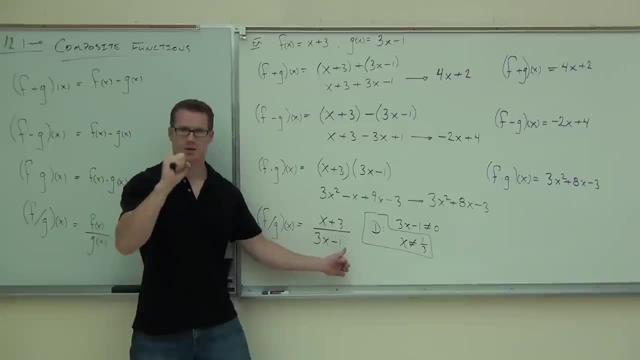 So that's what we're going to do. Would you raise your hand, if you feel OK? on addition, subtraction, multiplication and division of functions: Good, Good, Hey. that's half our lesson, right there, That's the first half. 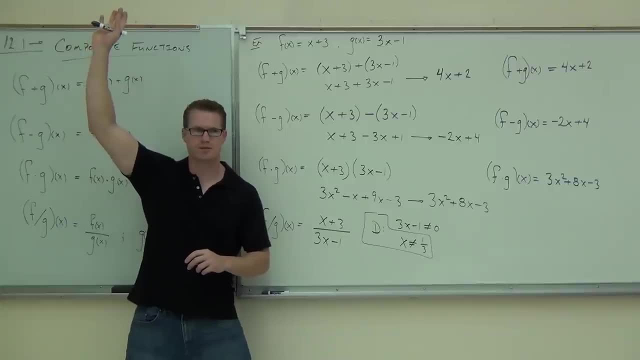 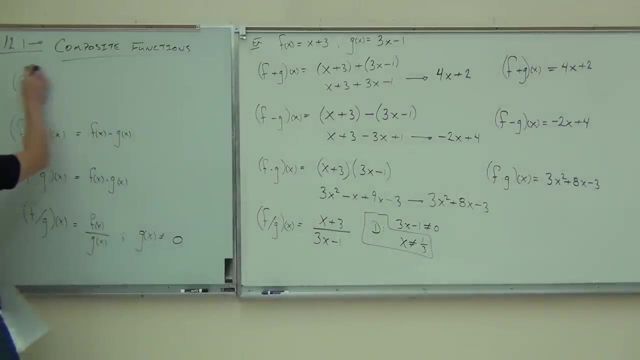 Now the second half. By the way, I told you these were going to be quick. right, These are quick sections. The second half of this section says There's one other thing we can do besides adding, subtracting, multiplying or subtracting. 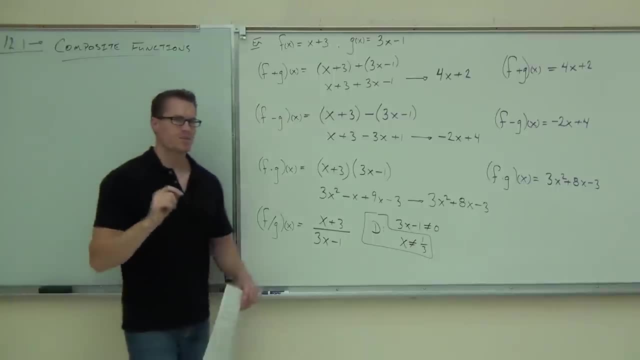 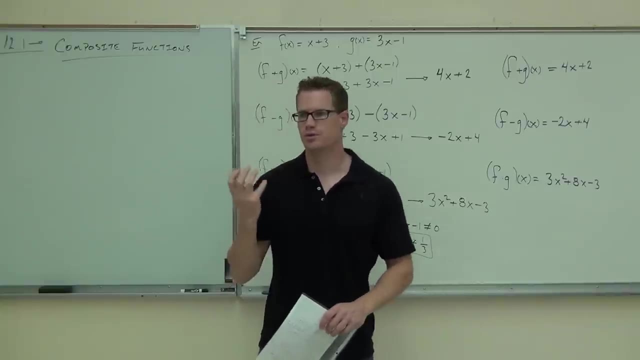 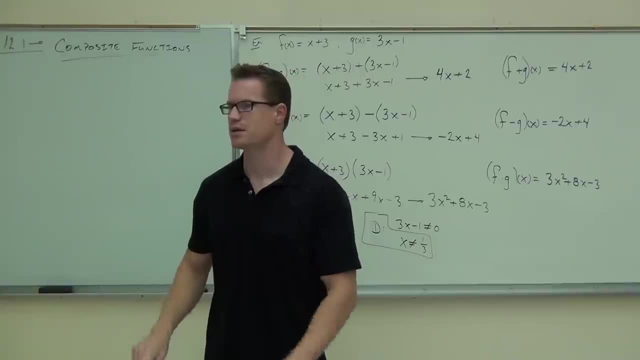 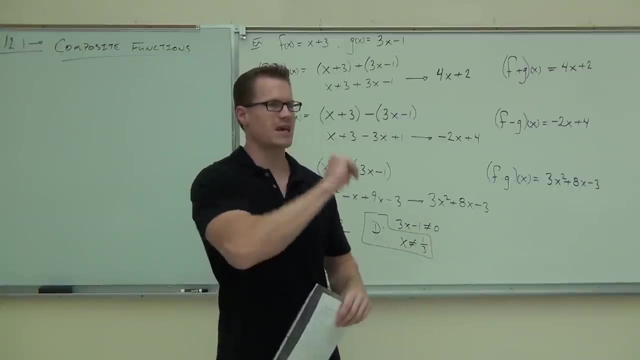 compose. you've composed things before. you've heard of people compose things. what? what's that mean? create or put together? you compose music, right? you make a composition paper. you're putting stuff together. that's what we're gonna do with our functions: we're gonna put them together. besides addition: 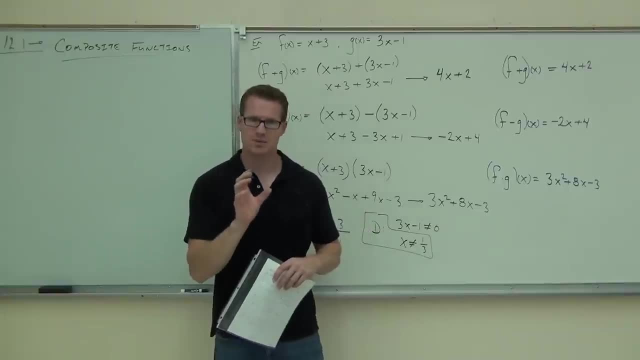 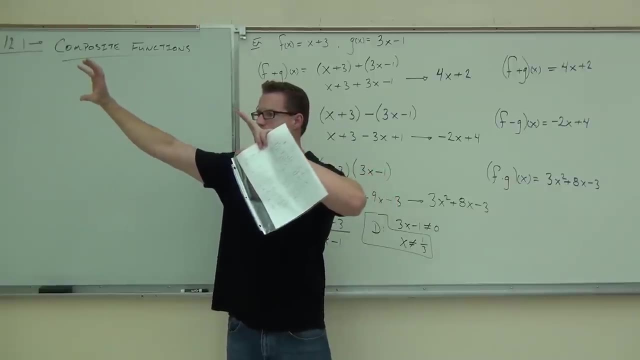 subtraction, multiplication, division. what we're gonna be doing is basically here's what composition does: takes one function and puts it inside another function. it says, oh, here's one function, I'm going to augment it by inserting another function into it. that's what composition does. so we're going to be: 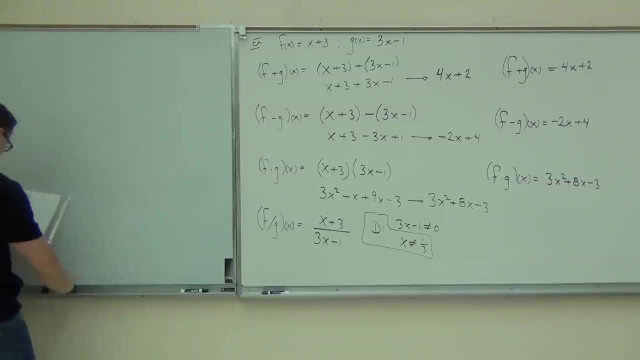 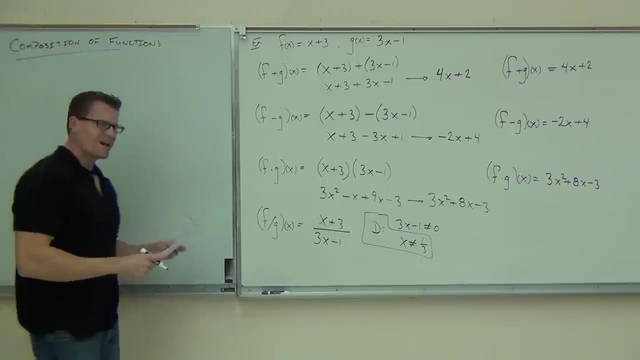 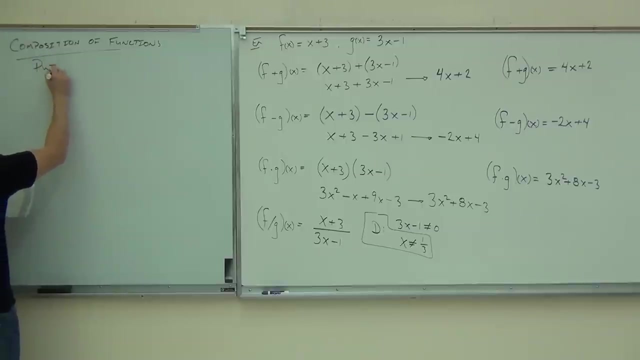 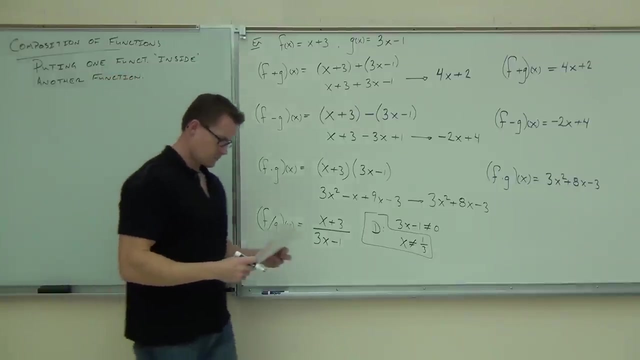 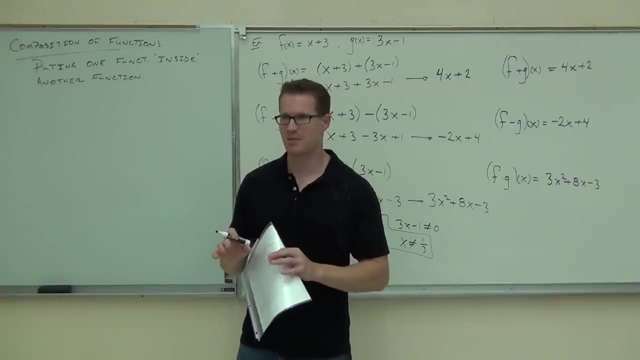 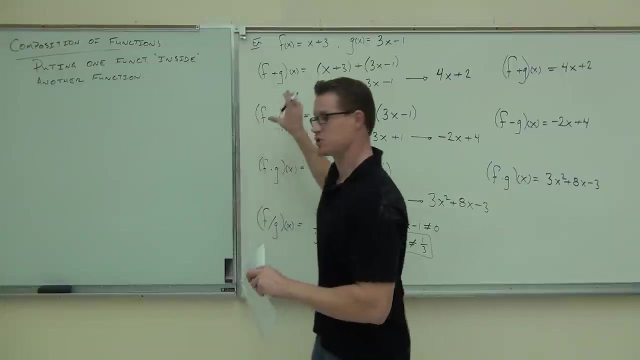 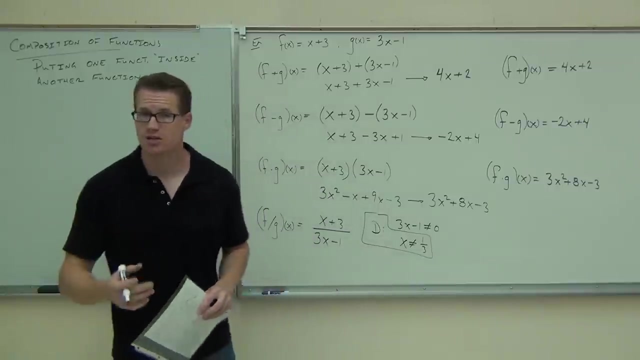 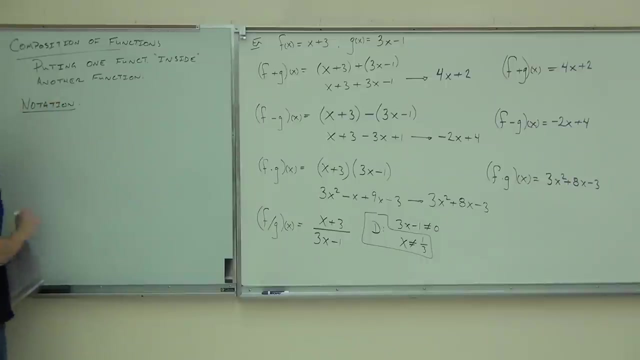 composing functions, composition of functions, and this does. I'll give you the English on this- this is putting one function inside another function. it sure is you. it will be appropriating夜 to happen. it's not I. it will be pretty hard, you know. I don't even know what he's talking. 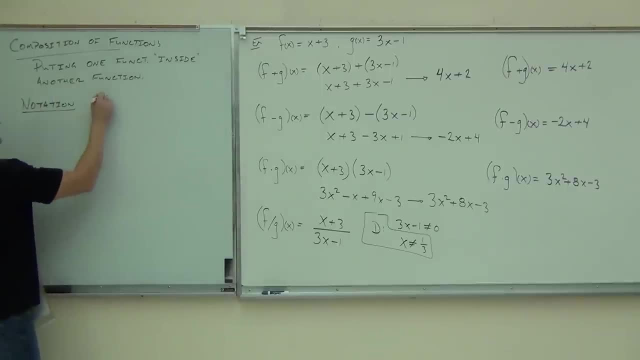 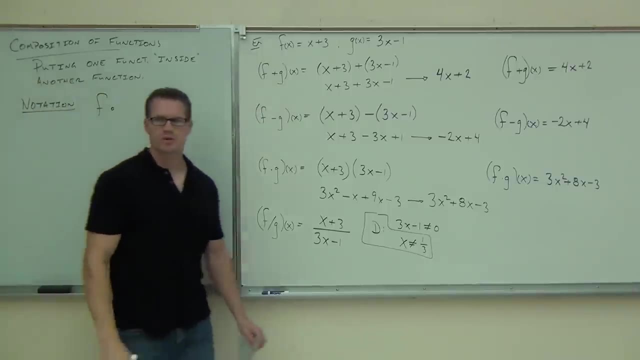 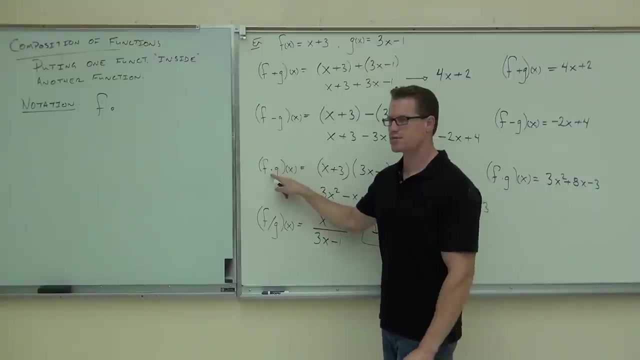 about here. here's what the notation looks like. here's what a composition of functions look like. you had the function made just like F Over here. difference between this and that. yeah, that's right. this does not mean multiplication. all right, this does. I know it's a little confusing, right here. 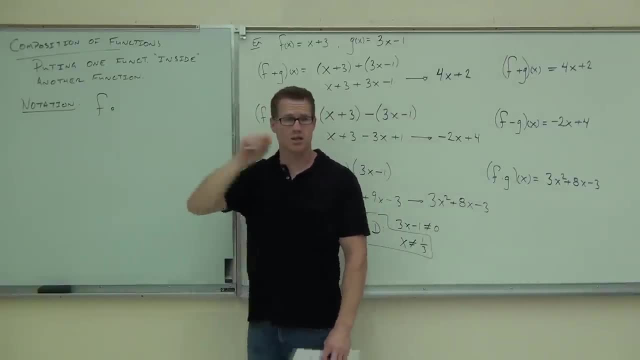 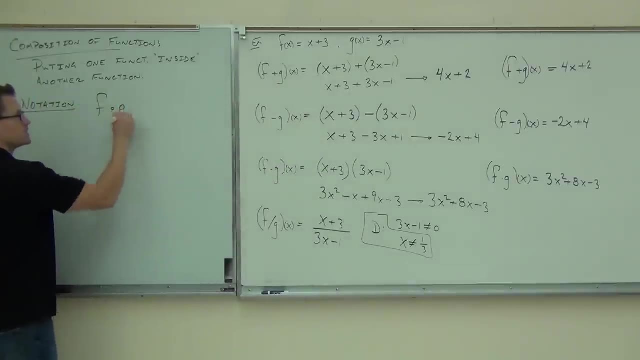 the little dot. we have an open circle. that doesn't mean multiplication. it's an open circle. it means of, oh, it's, it means a composition. this is f of G of X. so say this with me: this is f of G of X. that's what it says, and little note not. 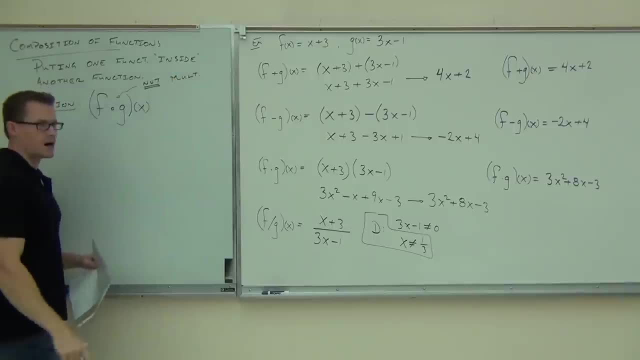 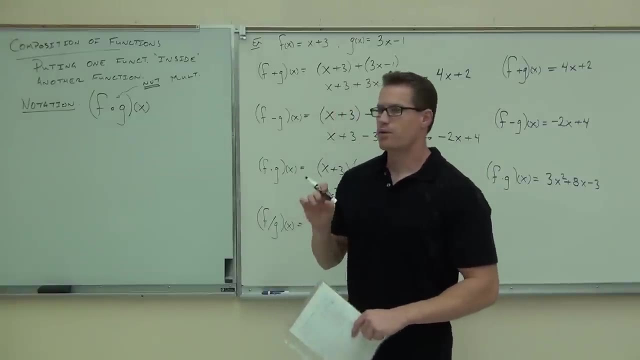 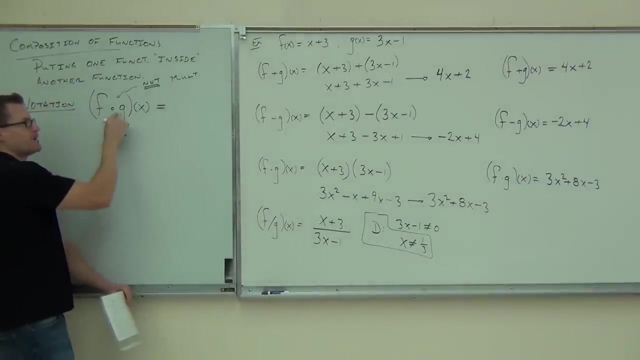 multiplication. that's not multiplication, it's a composition. now this is kind of kind of interesting, kind of nice for us. actually, you here's what this equals: f of G of X. guess what? that's the same thing as f of G of X. those are read the same way. look at this with me: this is f of G of X. 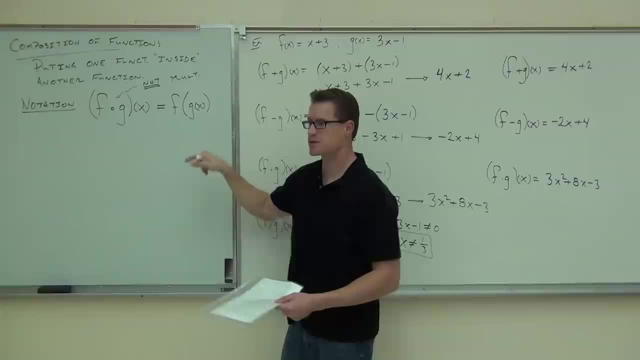 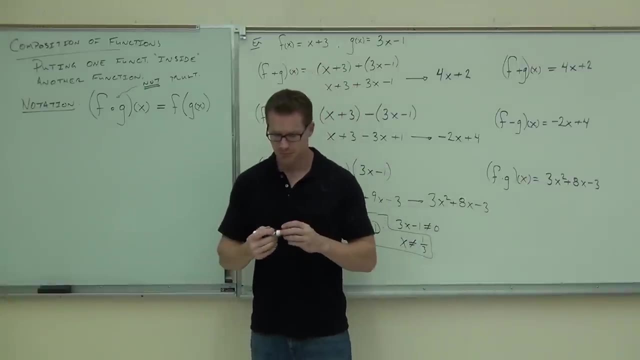 right, this is f of G, of X. those mean the same thing now. now what's it mean mathematically for you? what this says in English is this: it's gonna be a little bit confusing, but you're gonna see this in just a bit when we do an example. 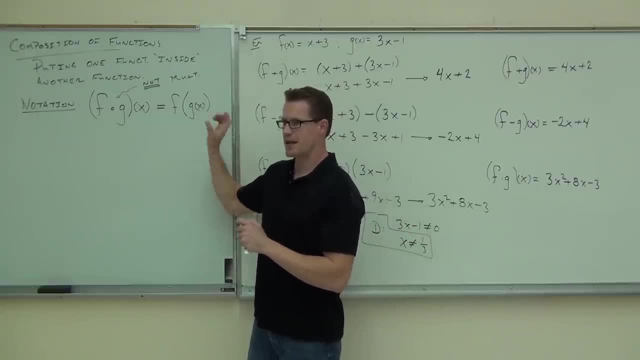 this says: everywhere you see an X variable in the function F, you're going to insert the entire function G of X. does that make sense to you? everywhere you see an X in the function F, you're going to insert the entire function G of X. you see, this means f of something right, some expression, what you're gonna. 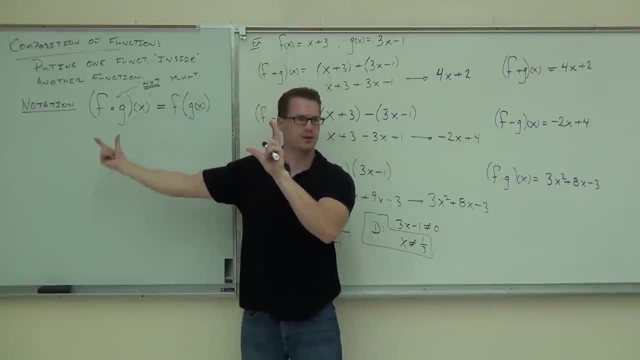 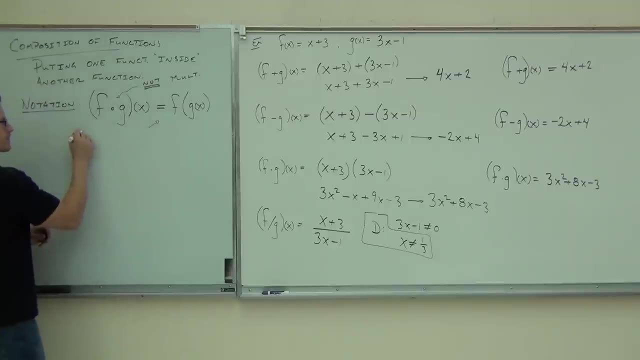 do is look at that function F, everywhere you see X, you're gonna put the entire thing G of X. that's what that means. so in English, everyone, everywhere I can say it in English, we'll see. it is Friday, right. what do I do on Fridays? drink on Fridays. I'm just kidding. 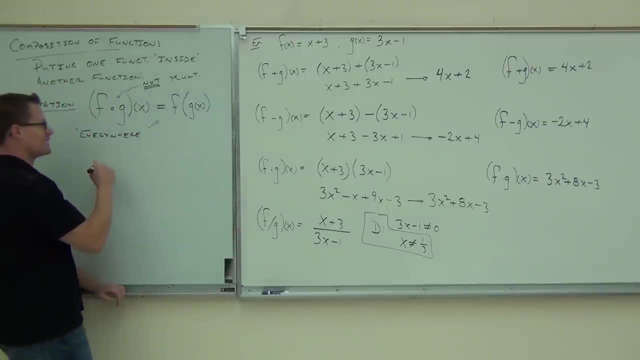 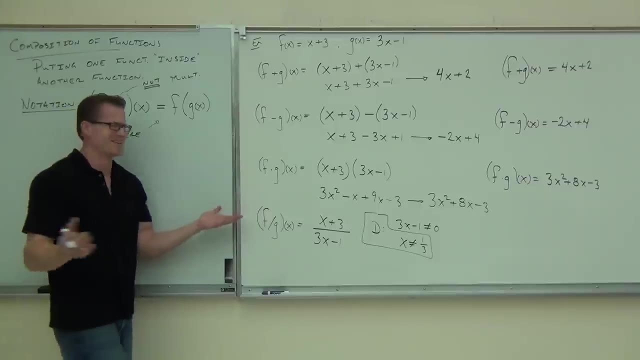 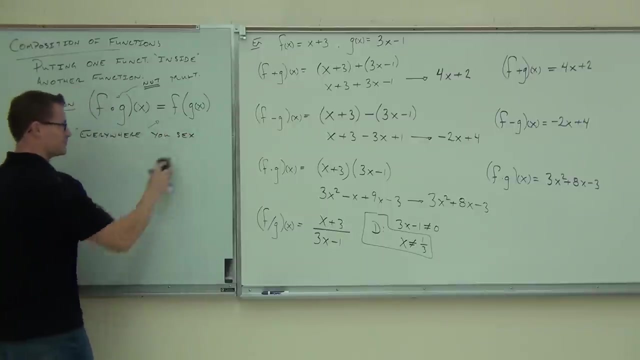 I'm only joking with that. I don't even really drink. so now, this is a celebration. you know you have like champagne at weddings or something. Friday's a celebration. come on joking. everywhere You see whoa. I missed an E. I missed an E. everywhere you see X. I don't have fun in math lessons. obviously, everywhere you see X. that's a dangerous statement. right there in F of X you insert. 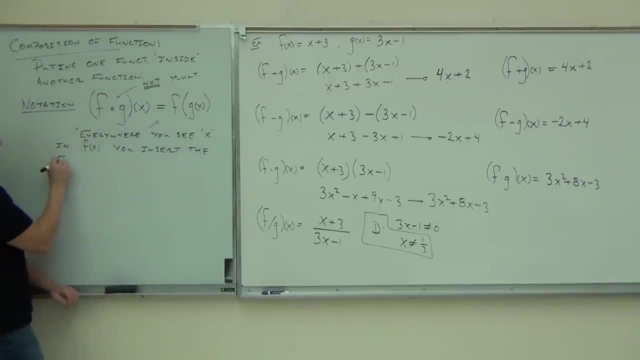 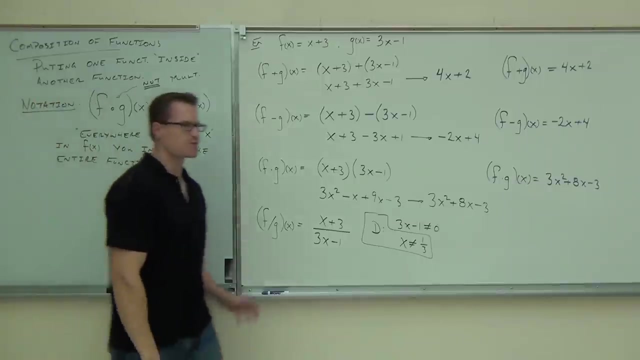 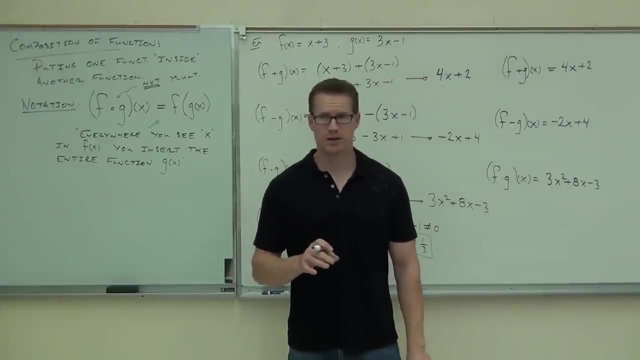 insert the entire function G of X. That's what that says in English. Everywhere you see the X in F of X. you're going to insert the entire function G of X. Now I have a nice way of doing this for you. Are you ready to see how to do this nicely? 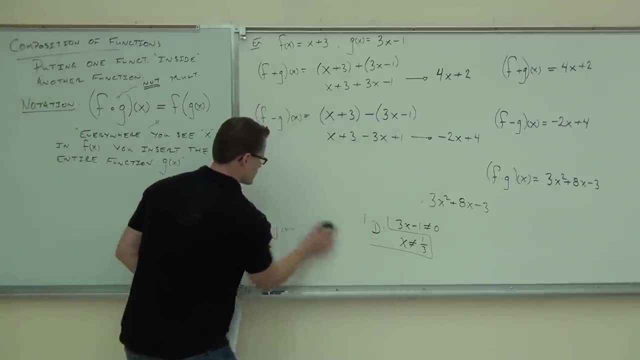 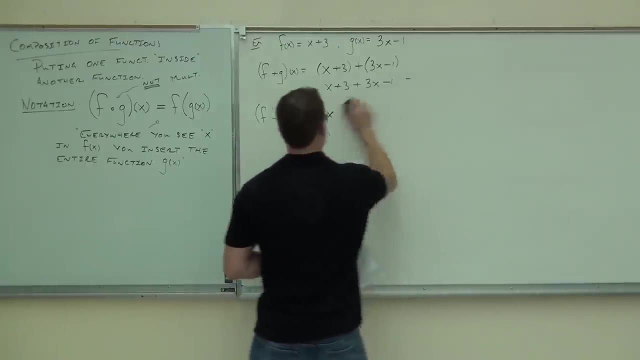 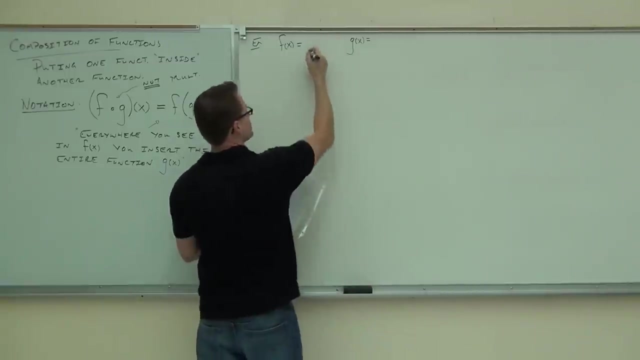 Alright, I'm going to erase all this. We're going to move on. I'm going to move over here because I want to make sure you see this nice and clearly show you all the work on it. Let's create two new functions, just so we really see how to do this. Here's X squared and G of X will make it 2X plus 1 works. 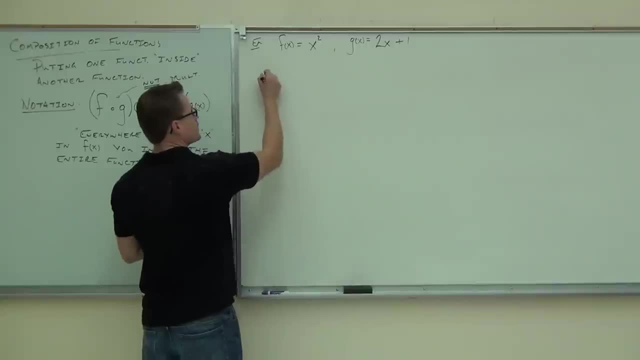 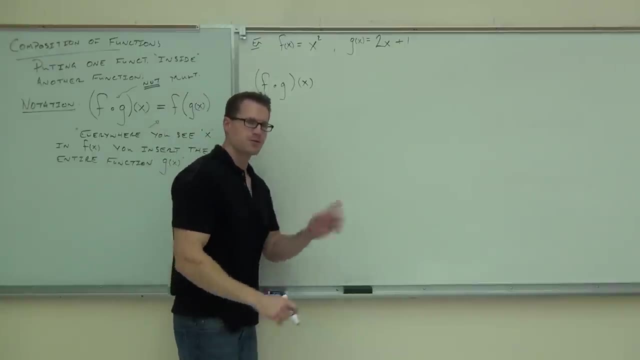 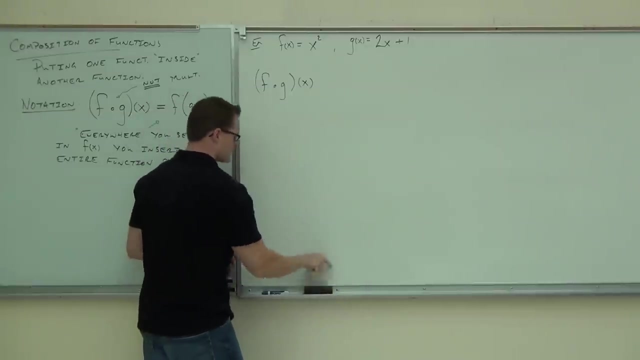 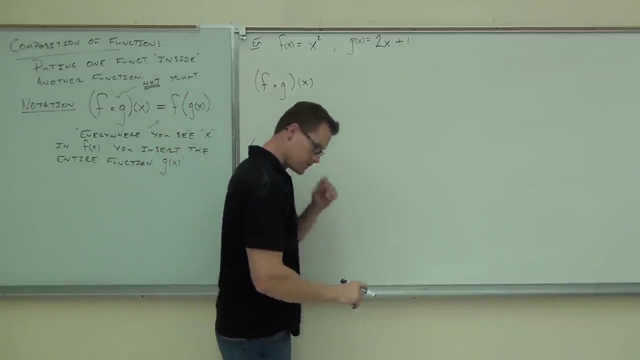 We're going to do several things. The first thing we're going to do is find F of G of X. After that we're going to find G of F of X and we're going to see if they're the same. Okay. 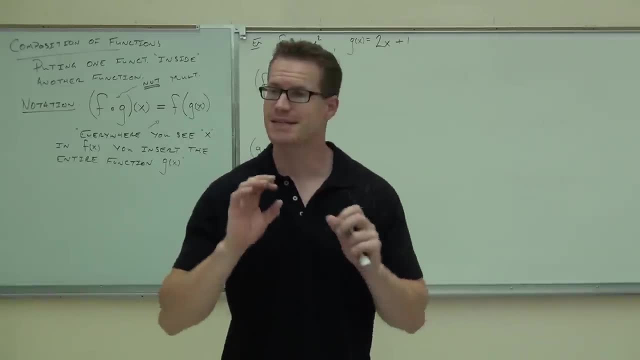 Trust me on it, Trust me on it, Trust me on this. If you follow these steps exactly like I show you, it's a piece of cake. If you don't, if you try to just kind of do it all in your head, it gets very confusing. 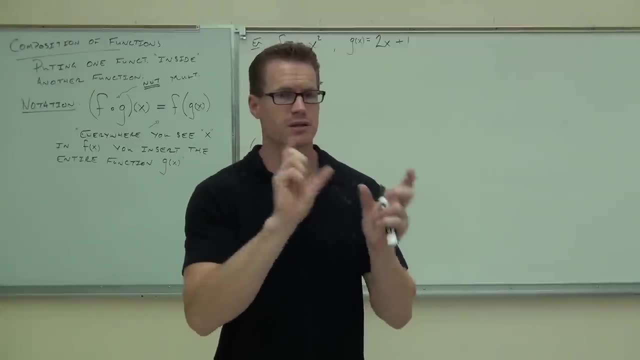 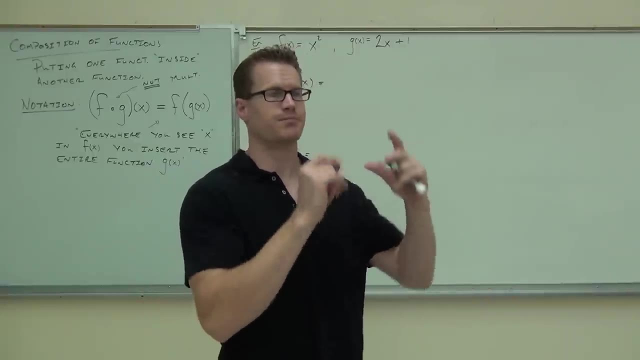 because you're alternating functions here. Okay, You're going to go between two different functions. You've got to have them in precisely the correct order, Otherwise you're going to get the wrong thing, Or you're going to get you're going to put the same function inside the same function. 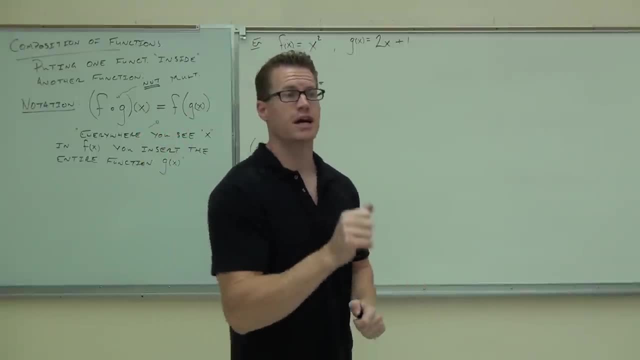 That doesn't make sense at all. We're going to take one function and put it inside the other function. Here's how you do this appropriately. First thing you need to know is that this order stays the same when you do this process right here. 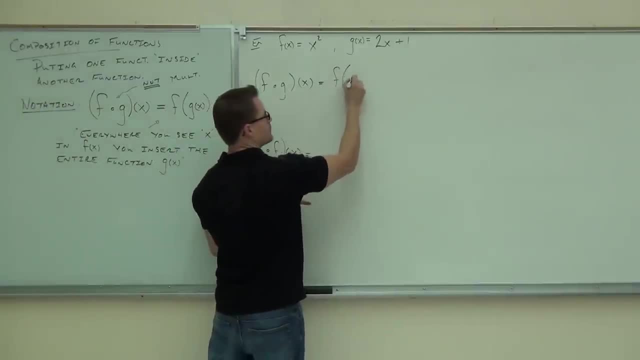 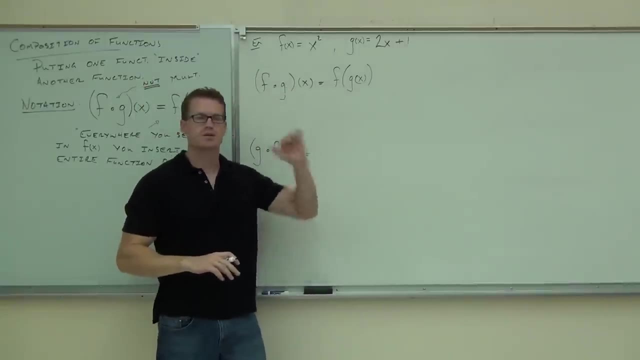 So F of G of X is F of G of X. So this is F of G of X. That was the definition of it. I already have that on the board over here. Are you okay with this one? Here's what you do now. 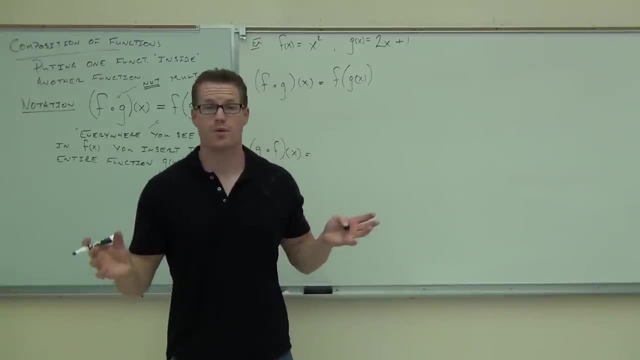 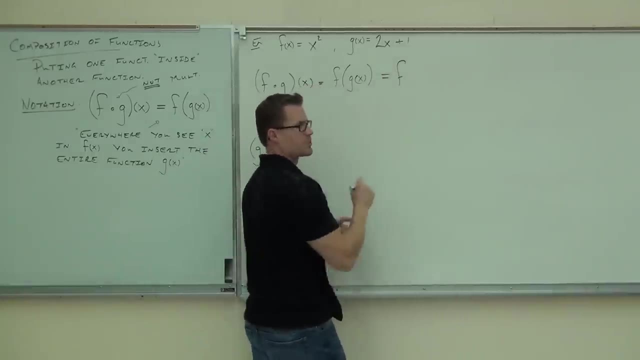 What you do is you work from the inside out, just like you normally would, in order of operations problem. Okay, So the next thing we're going to do, we're going to keep the F, because that's on the outside of my parentheses here. 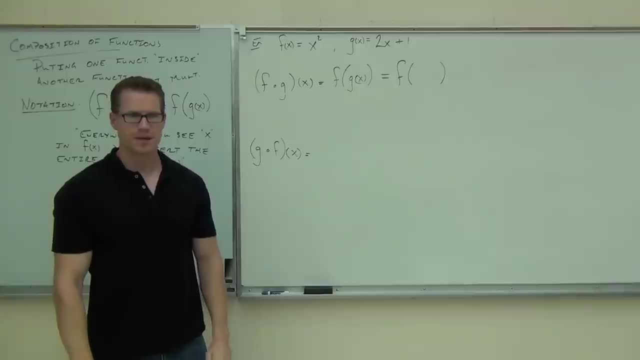 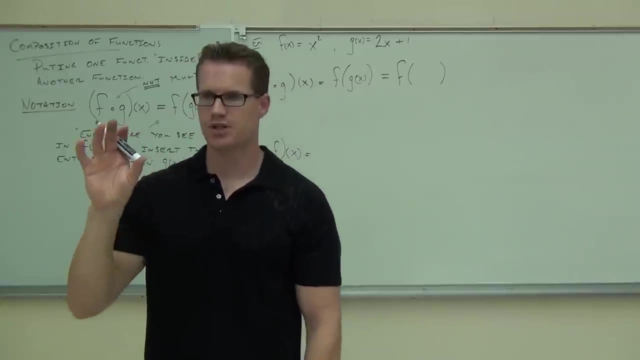 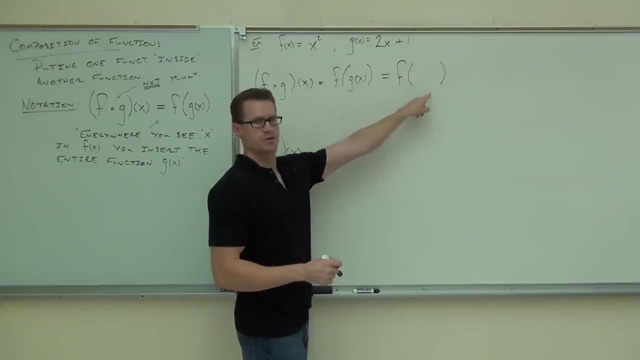 But on the inside of my parentheses, on the inside of my parentheses, I'm going to replace G of X with the actual function of G of X. So go look up top where G of X is, How much is G of X? So instead of having G of X, I could instead write two X plus one. 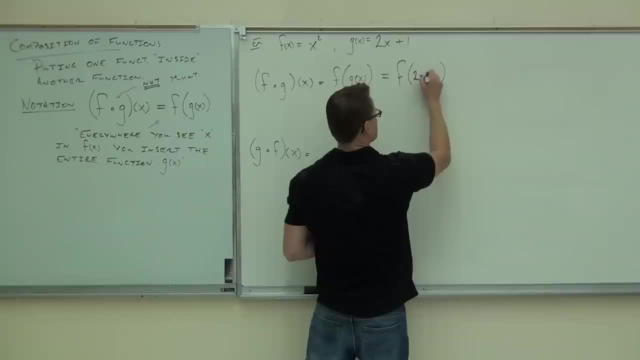 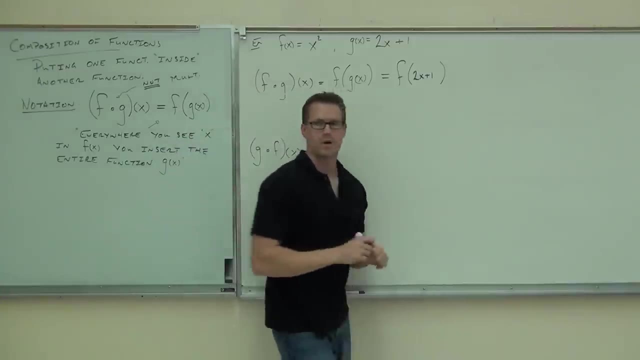 Are you with me? Write that. Are you sure you're okay with this step? I'm sure you're okay with this step. Okay, So F of G of X, F of G of X, F of. well, that's still G of X, right? 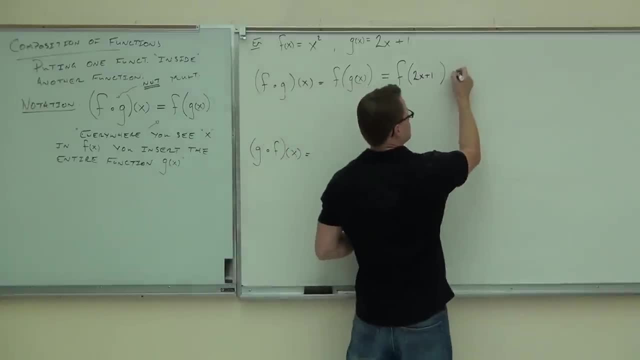 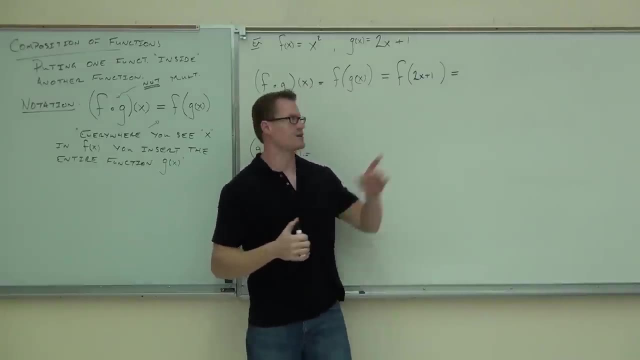 These all say exactly the same thing. Now, here is the key, the key to doing this: What's the only letter left on the board? X, Besides X, X. There's lots of letters on the board, actually Lots of writing. 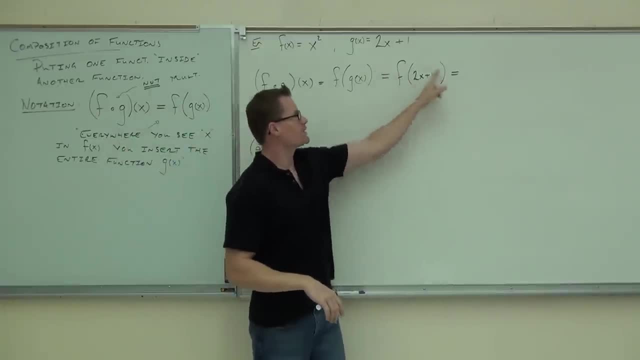 There's Y, Never mind Over here, the only letter that represents a function left on the board. what's that letter? X1.. I'm sorry, The letter. I want you to look at the function F. Okay, look at the function F. What is the function? 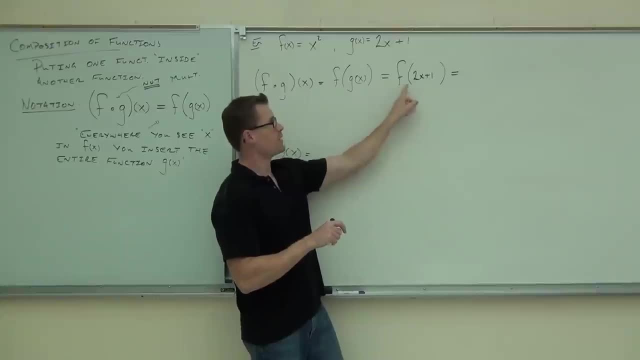 F, X squared. Okay, so this, this refers- we're going to ignore this for just a second, We're going to look right here. This refers to a function that's still left up there. yes, And it says X squared. 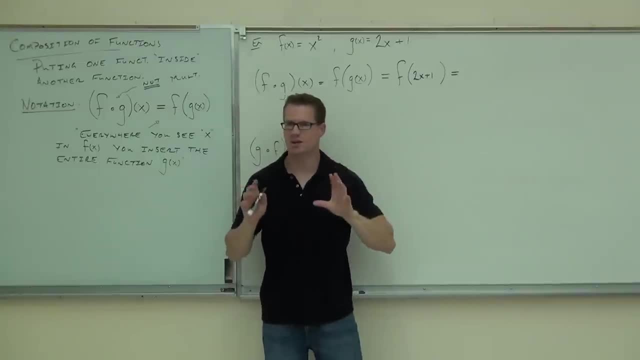 X squared You with me, X squared Now. you're going to say: say X squared, X squared, X squared Now. everywhere where you said the word X, you're now going to replace that word with the word parentheses. Okay, 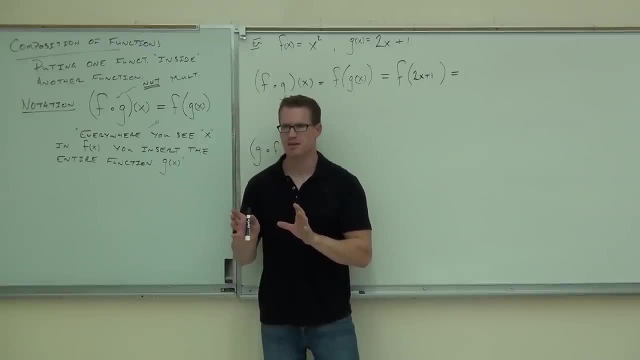 Trust me, Just trust me Now. you just said X squared, didn't you? Yeah, X squared, Now it's. I said X squared Instead of X. what word are you going to use? Parentheses? So now, finish that statement. 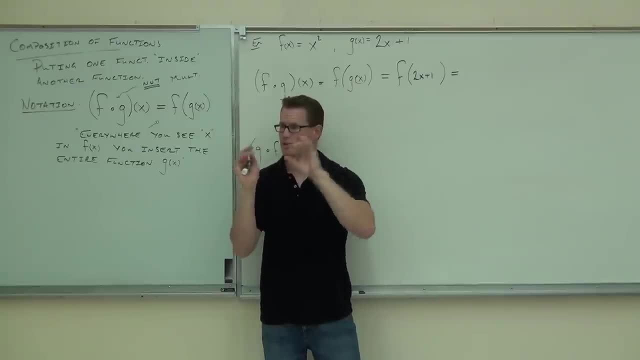 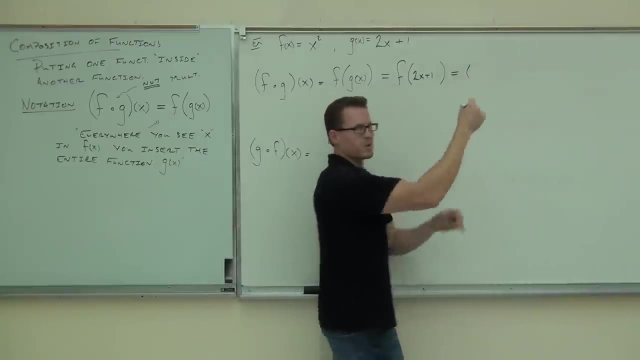 Parentheses squared. Parentheses squared. Don't forget the squared Instead of X squared, you're now going to have parentheses squared. Are you with me on that? Write that Write. don't write the word parentheses. Okay, Write parentheses squared. 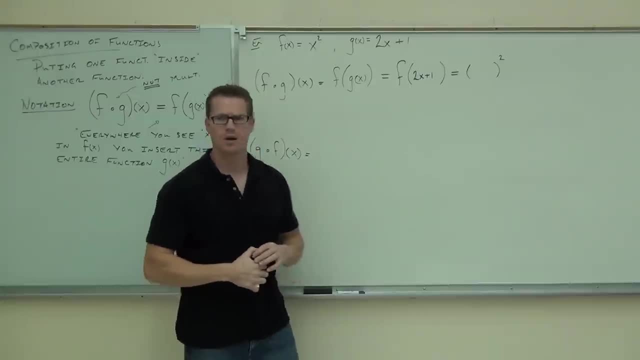 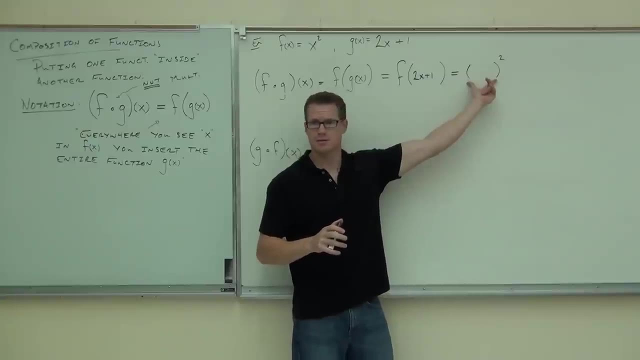 Okay, Are you all right with that? Now I need you to see that, essentially what we've done, this stands for your x. yes, In the function f right, This stands for your x, and we're still squaring it. 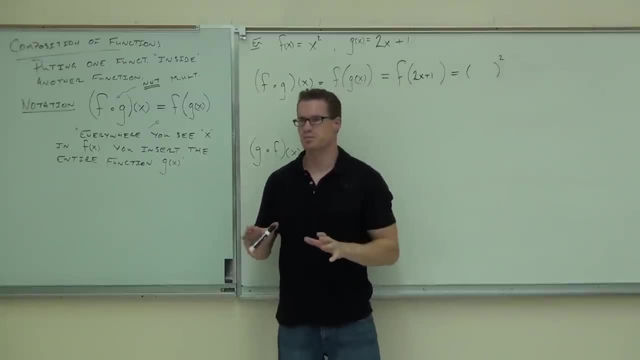 Do you follow? That is x squared. Here's what you do. That's the key point right there. If you can get that, you're essentially done. Okay, that's it Small thing, Okay. what was in this parenthesis now goes inside of this parenthesis. 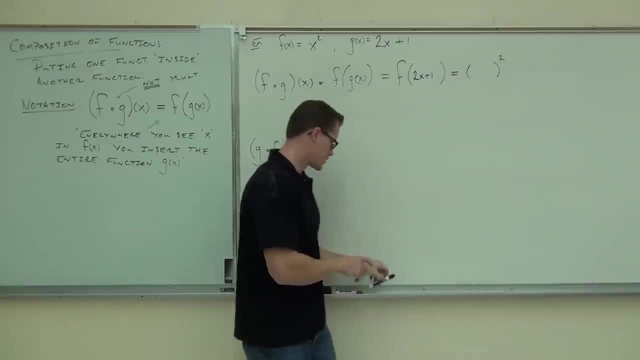 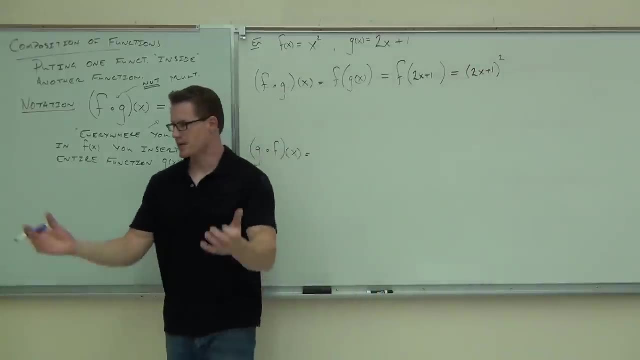 That's it. Just transfer it right over, Can you do that? So what's going to go inside that parenthesis? So x plus 1.. That's the composition of functions, That's f of g, of x. That's it. So there's no real x. 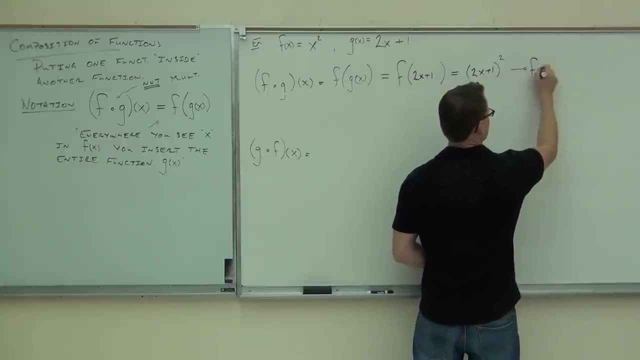 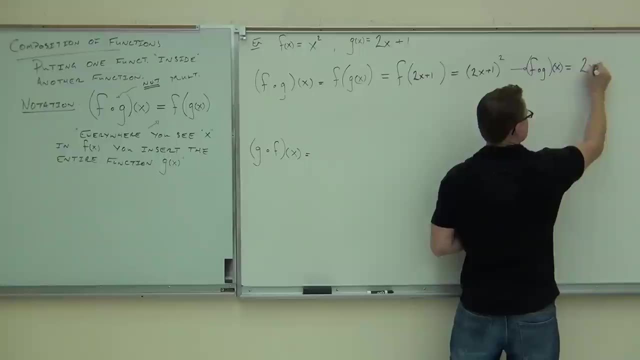 What do you mean? there's no, that's an x. Oh yeah, but the other one, the x, squared. you just used it as an imaginary. No, it's not imaginary. See, that's the cool thing about this is that what's happening is you're inserting the entire. 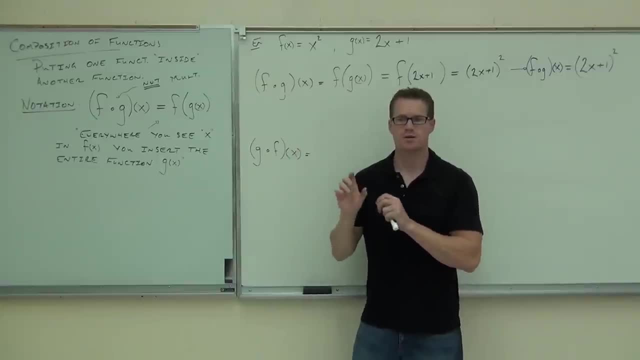 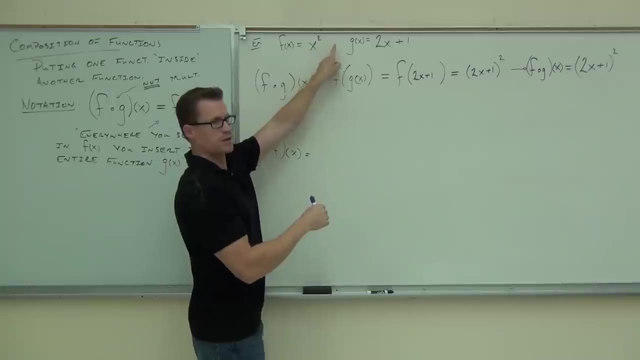 I gave you a simple example here, because you can really see it. You're inserting the entire function g of x into f of x. See look what happened. This was x squared right. This is 2x minus 1.. Take this, put it instead of x and you get that. 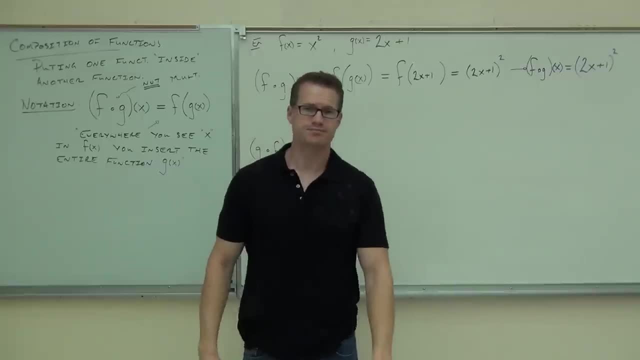 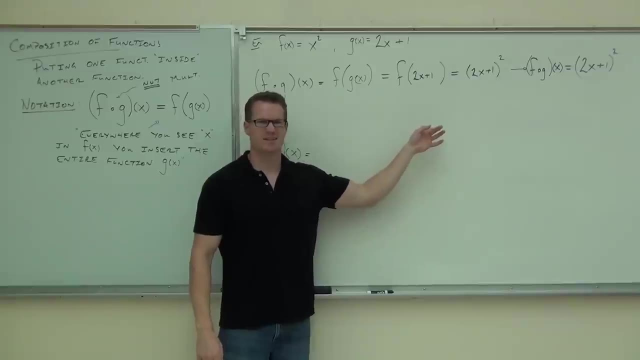 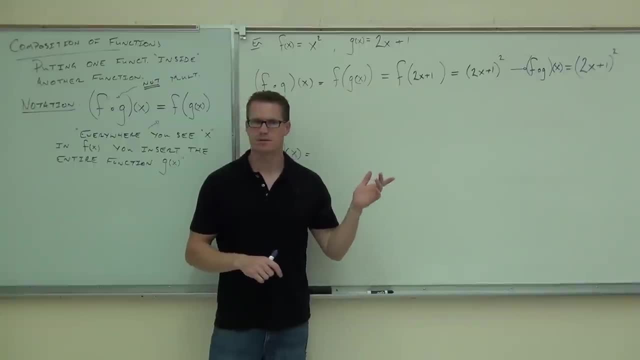 Yes, no, Yeah, Can you follow the process? Yeah, Good, This inserts one function into another function. So instead of x we now have the entire function g. So it's kind of hard to think of if you're just doing it off the cuff, right. 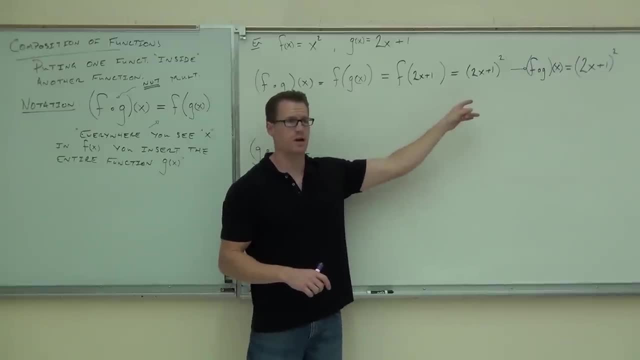 Like I don't even know. But if you follow the process you will get the right answer every time. What this does inherently is takes one function and puts it inside, So you'll have one function inside another for every single time. you have that variable. 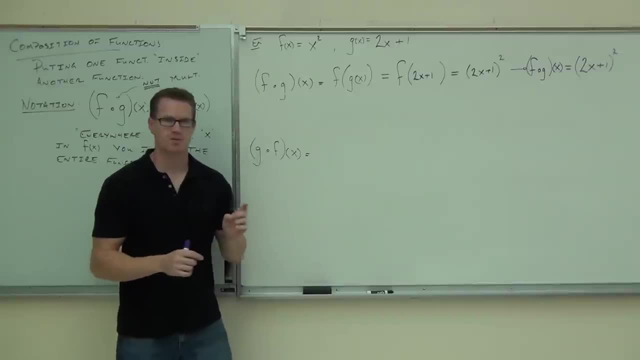 Let's go ahead and let's try that with g of f, of x, and see if it's the same thing. Let's see, Do you think it's going to be the same thing? No, We're taking one function and putting it inside the other function. 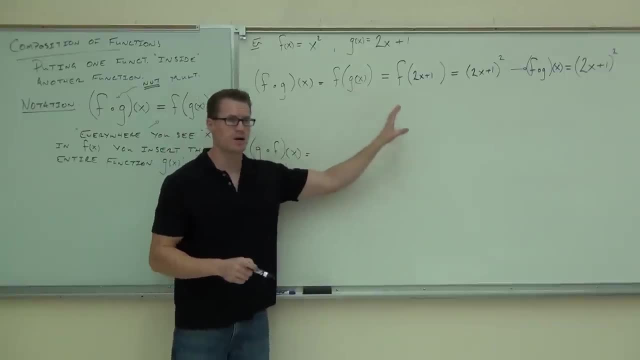 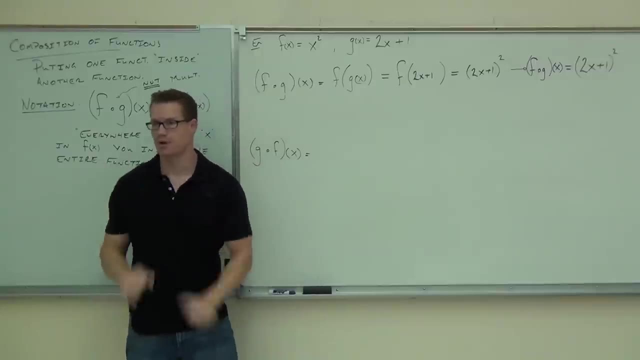 Let's see if that happens Now. this is an important example for you to follow. Even if you think you got this one down, just pay attention here. One thing happens on this particular example that you've got to make sure doesn't happen on your paper. 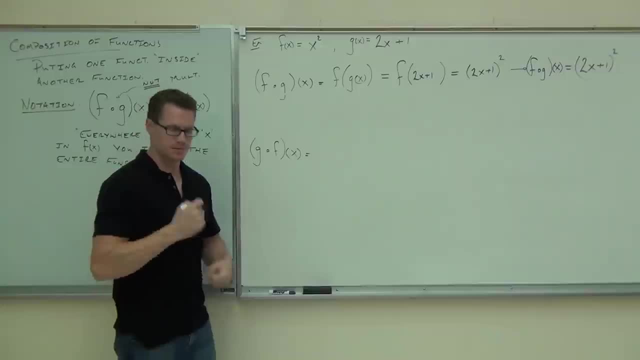 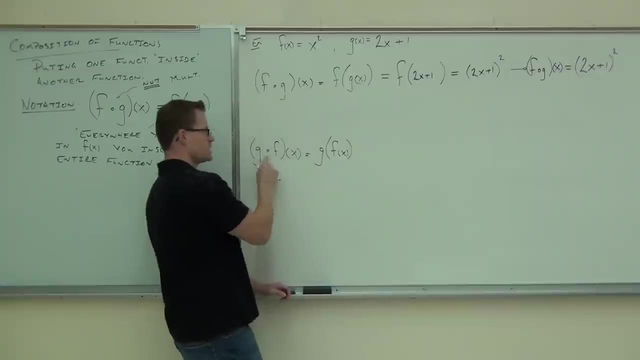 Firstly, the order has to be the same. So what am I going to write next? g of f of x, Sure, f of f of x. So g of f of x, g of f of x. Same thing Now again, just like order of operations. just like order of operations. 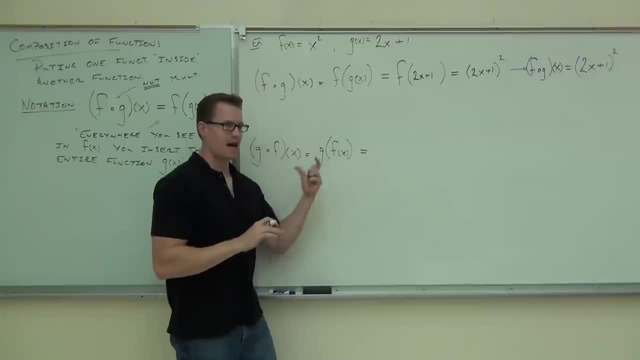 you're going to work from the inside out. So what letter am I still going to have over here? g- Good, I'm going to have a g Now, inside the parentheses. I'm working parentheses inside out here. instead of f of x, I'm going to have g. 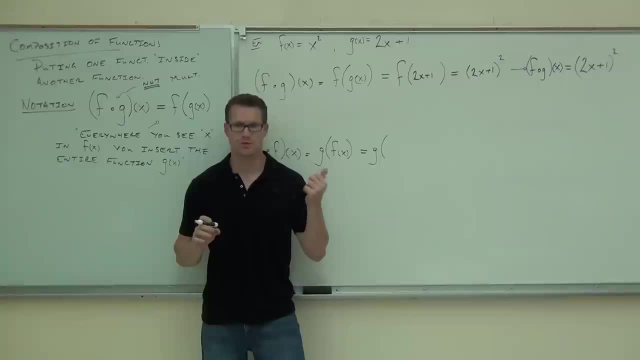 I want you to look back at the functions at the top. That's your reference guide. okay, That's where you refer back to. What is f of x, X squared? So instead of f of x, I can put X squared. 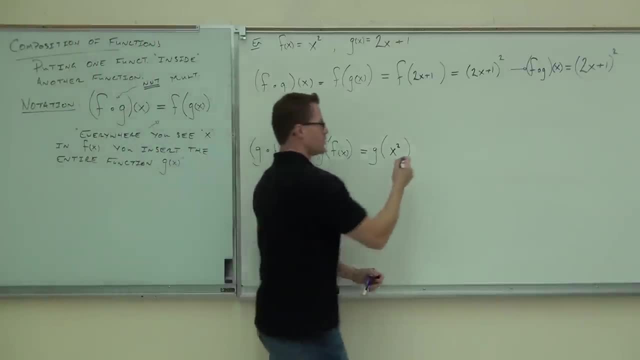 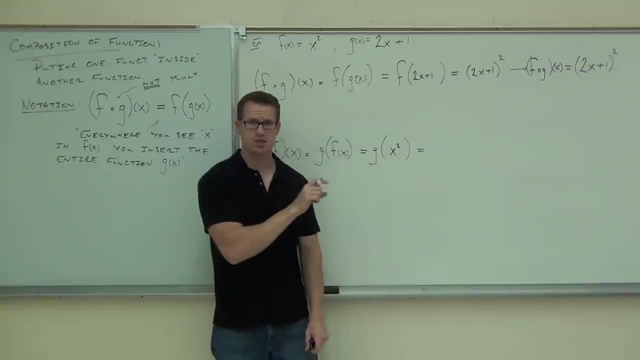 Raise your hand if you're okay. so far Good. What's the only letter left on the board that represents a function, G. So that says you're going to refer back to g. Can you see g? Read g to me: 2x plus 1.. 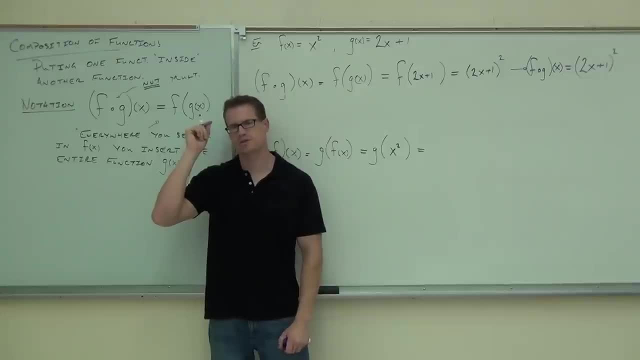 2x plus 1.. So you're going to 2x plus 1,, 2x plus 1,, 2x plus 1.. And then 2x plus 1.. Instead of x, what word are you going to use? 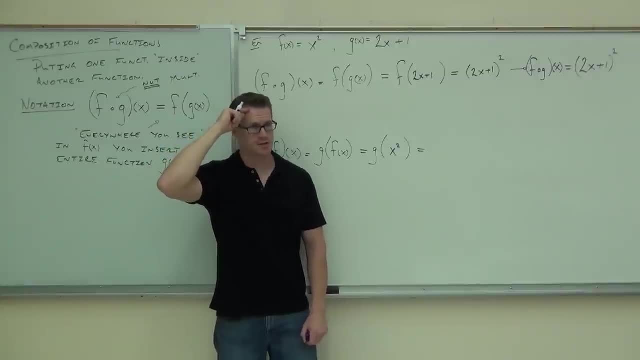 Parentheses. So say g, but instead of x, say the word parentheses. Say it out loud, Practice it. Parentheses plus 1.. Two parentheses- Some of you just stopped at two parentheses. Say the whole thing. Two parentheses plus 1.. 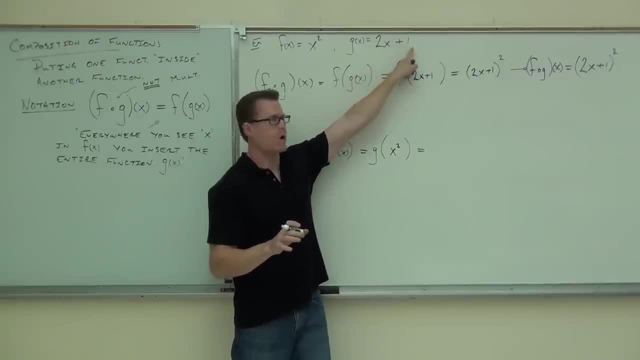 Two parentheses plus 1.. Are you with me? Uh-huh, Why are we going back to g? Well, it says g. That's the only letter we have left. Do you follow me on that, Yes or no? Yes? 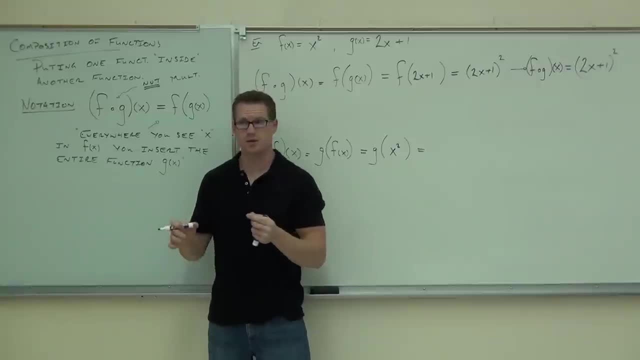 You sure? Yes, Uh-huh, This can be confusing if you're really not sticking with it. So if there's questions, man, you've got to ask, You've got to ask now, Because to me it makes perfect sense. 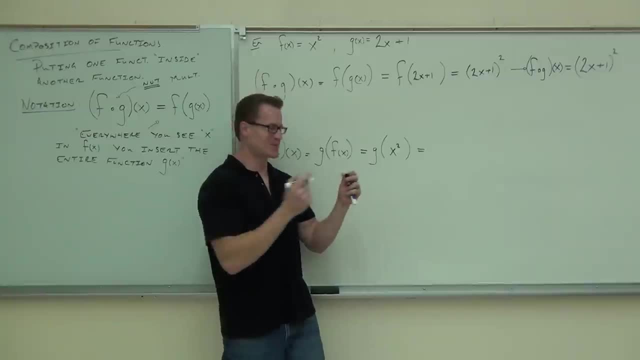 I've taught this class over 13 times. It makes absolute sense 17 times. I don't know It's a lot. So anyway, you look back at that letter. You say 2x plus 1. But instead of x you're going to say parentheses. 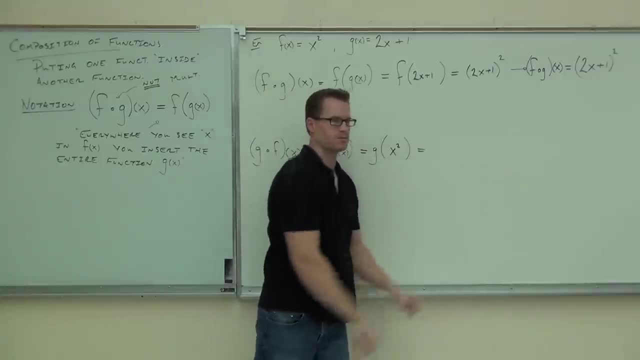 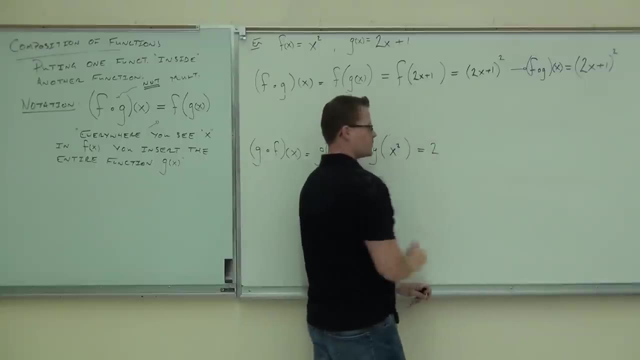 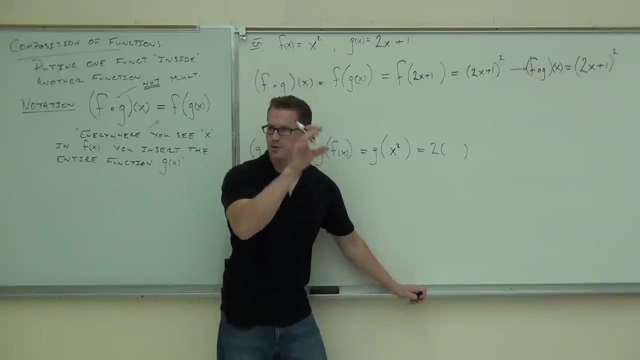 Two parentheses plus 1.. Write that on your paper now. Okay. So 2, what's next Parentheses? What's next Plus 1.? Notice how the plus 1 is going after the parentheses. Do you see that? 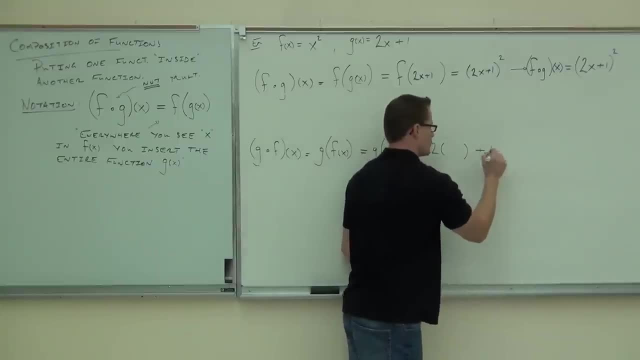 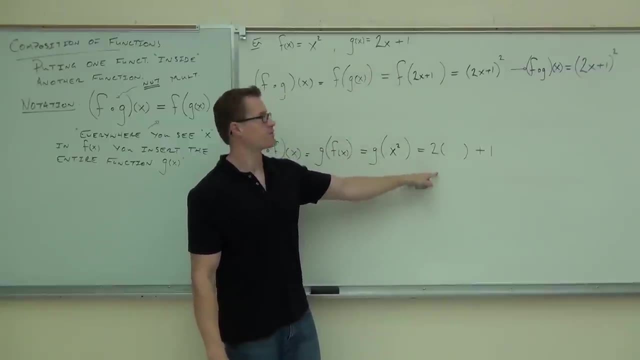 It's not within it, It's after it. Does this look like that function? Do you see the similarity? Uh-huh. What's the only difference between this and this? Arrangements? Yeah, that's it. Instead of the x, you have parentheses. 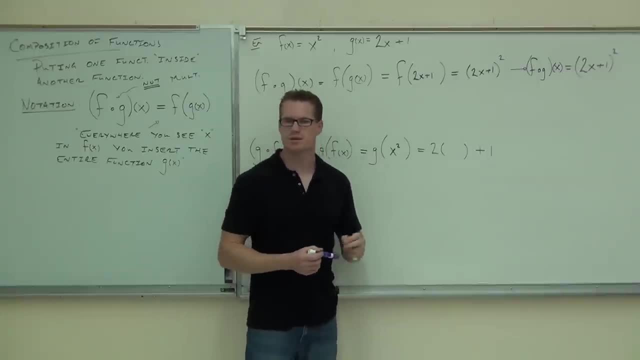 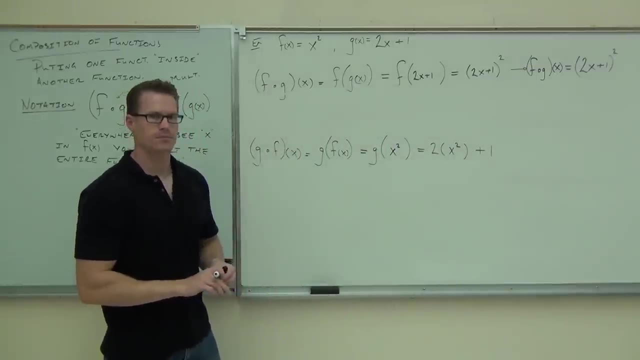 You're still okay. What goes inside the parentheses, That's it, You're done. How come you never need to simplify them? Well, you could distribute that out if you wanted to. You get 4x squared plus 4x plus 1.. 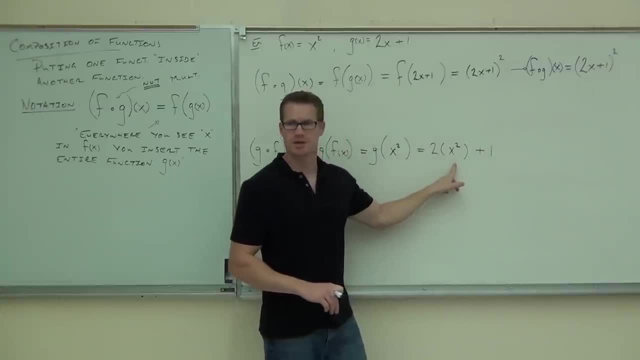 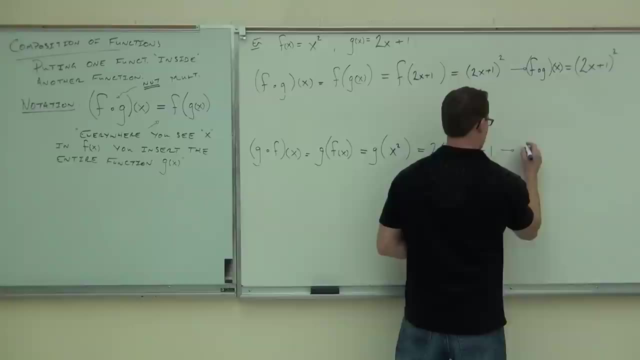 You could do that Here. we're going to drop those parentheses, because these parentheses really aren't doing anything. You're going to get 2x squared plus 1.. Do you see it? So this says okay, g of f of x. 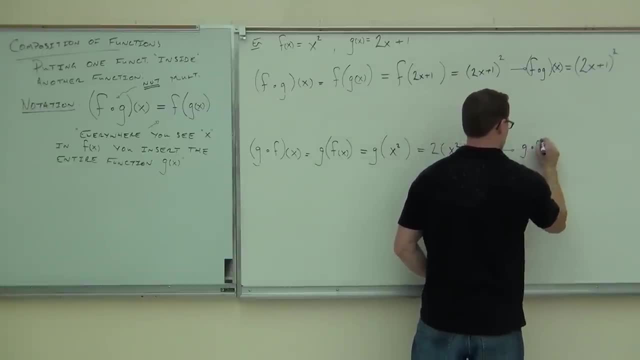 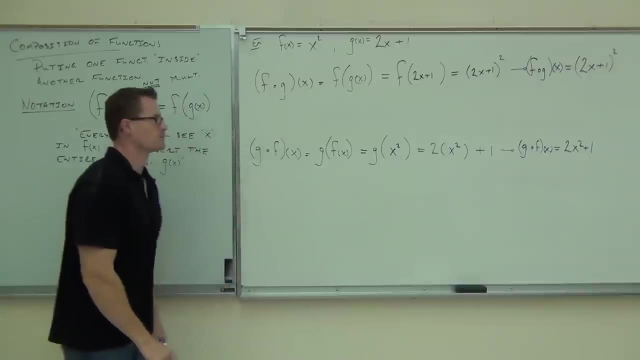 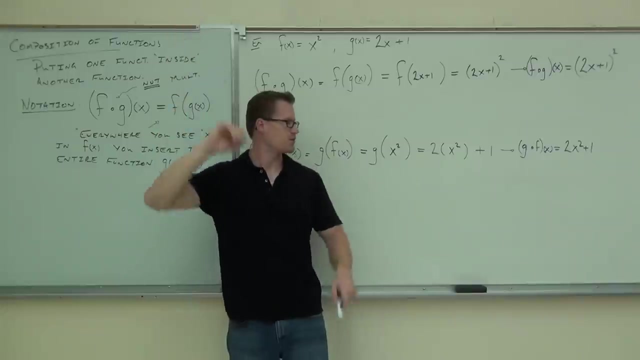 2x squared plus 1 equals 2x squared plus 1.. Would you please raise your hand if you're okay with this so far? Yes, Is that it for the left-hand side? Are you okay with that? All right, 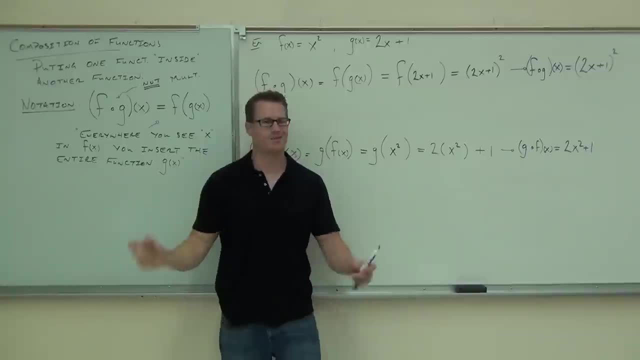 So is f of g of x and g of f of x the same thing? No, No, definitely not, Definitely, definitely not. Now there's one more thing the book's going to ask you, and sometimes they put this in the incorrect order. 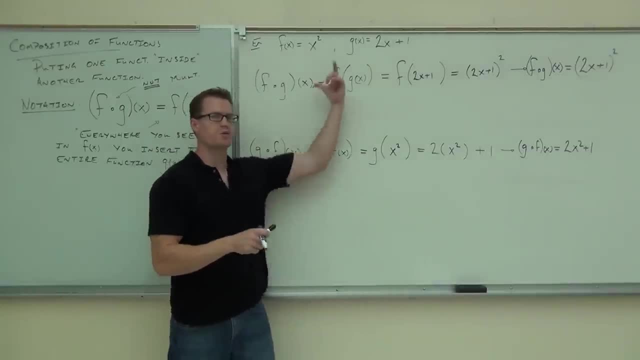 Sometimes they have you do it. They have you do the part I'm about to show you. before you do this part, Let me give you a big hint: If you're going to do these compositions, do the one with the x's first and get this expression. 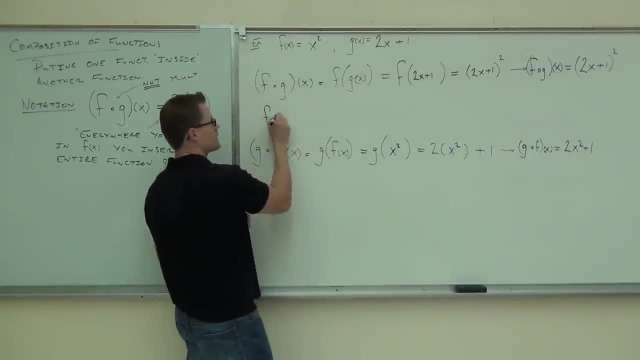 because the next thing they're going to have you do is do this: Find f of g of 3 and find g of f of 3.. Even if they ask you for this one first, do this one first. You with me on that. 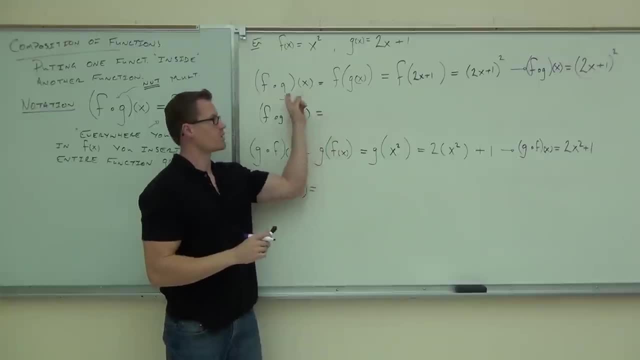 Don't try to do this one first. It's hard to do. It's harder You're going to want to find out your expression before you try to plug in a number. Otherwise you're trying to do two or three things at once. 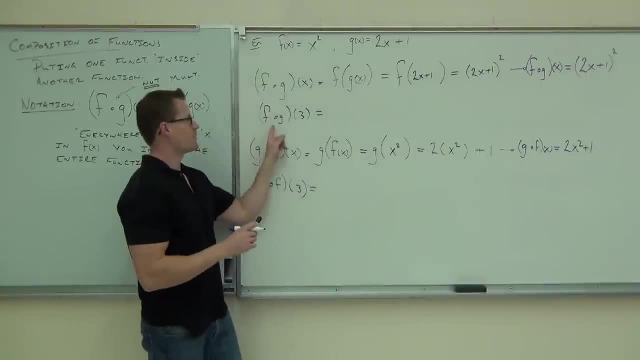 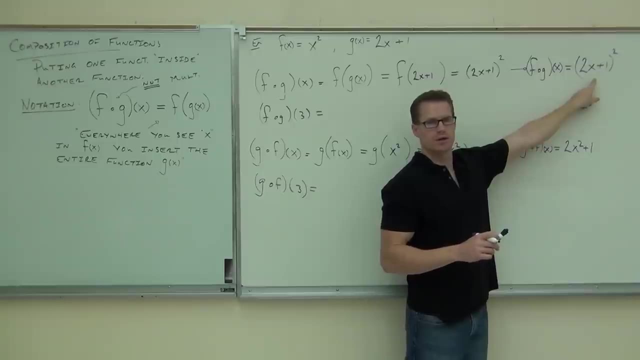 You okay with that one. So what does it mean to do? f of g of 3? It says: go back to f of g, Go all the way to the very end where you found it, and what number are you going to plug in? 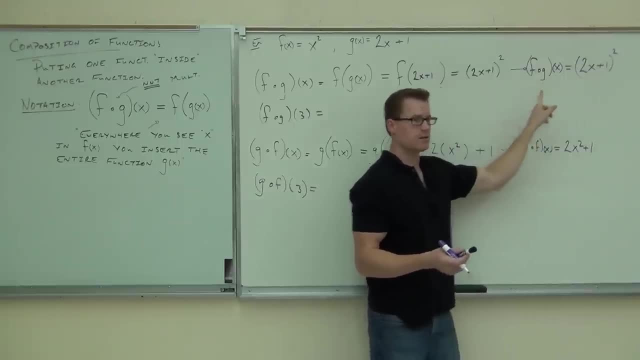 Three. Just plug in 3 to that. This is f of g right f of g of whatever number you want. This is f of g of. take whatever number you want, make it a 3. You're going to have 2 times 3.5.. 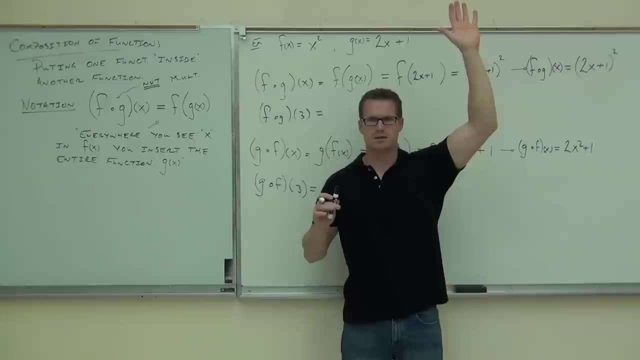 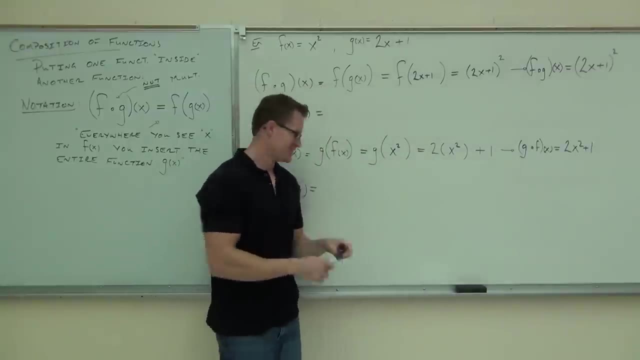 Plus 1 squared. How many of you can follow that idea? Did I just blow your minds? It's like a mine grenade. Now this says: go back to the function you just found, f of g. Identify that function. Go to the very end. 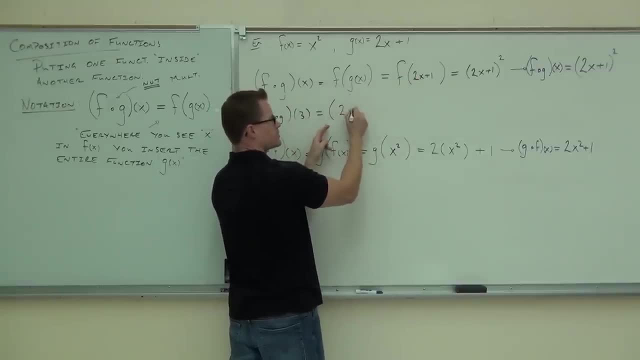 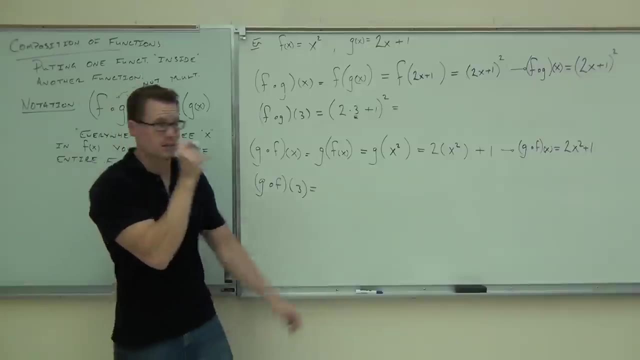 Say: okay, this was 2x, so instead of 2x I'm going to have 2 times 3 plus 1 squared. I'm just plugging in 3.. That's all I'm doing. Plugging in 3 to my function. 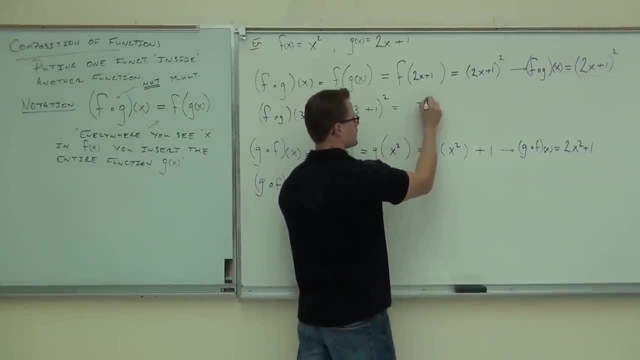 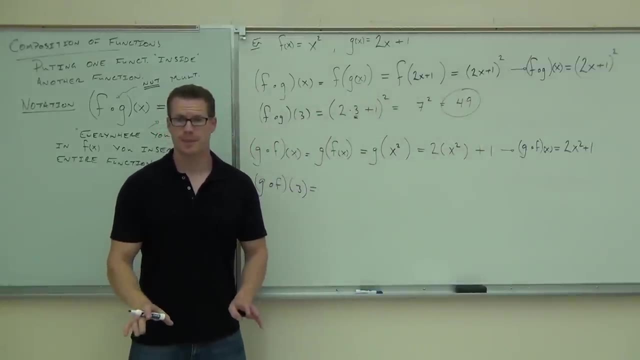 Okay, That's going to be 7 squared or 49.. Oh, so that's just only after. you would have that original problem After Got it. Okay, After That's what I'm saying, You do this first. 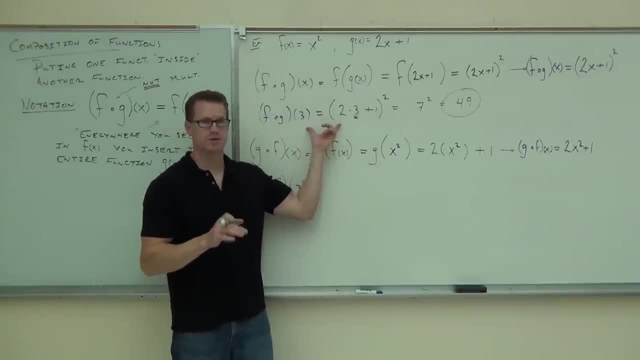 Even if the problem on the homework asks you for this, you need to do this first. You got it. Do that first. Dude, that wasn't going to be just f and g or they're going to use different letters. They could use different letters. 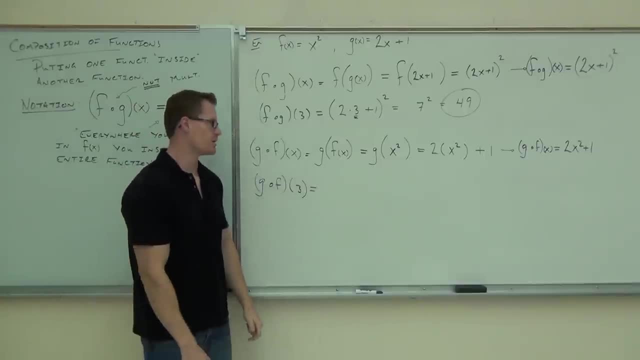 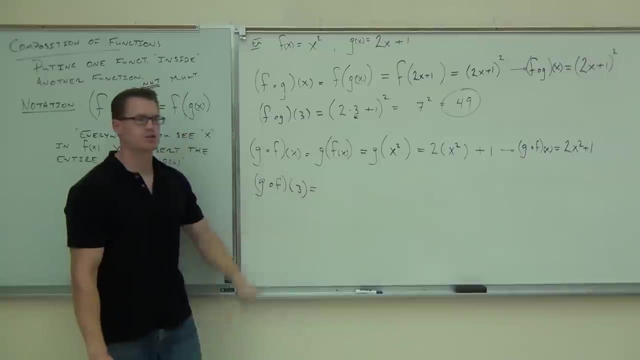 They could have h and j or whatever. It doesn't really matter, But it's going to refer back to 2.. These functions will be given to you, okay, And they're going to be different on your problems. What I want you to do right now is find g of f of 3.. 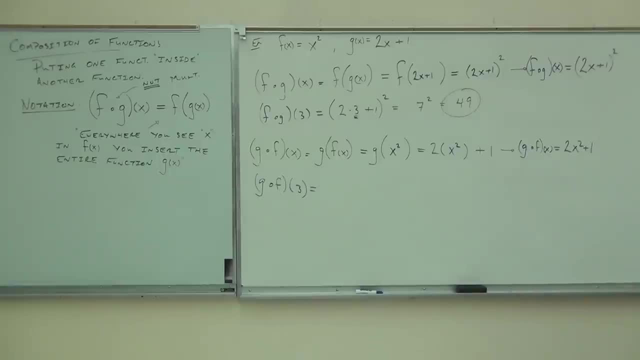 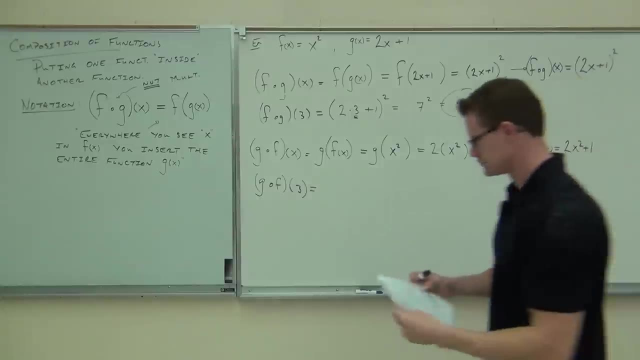 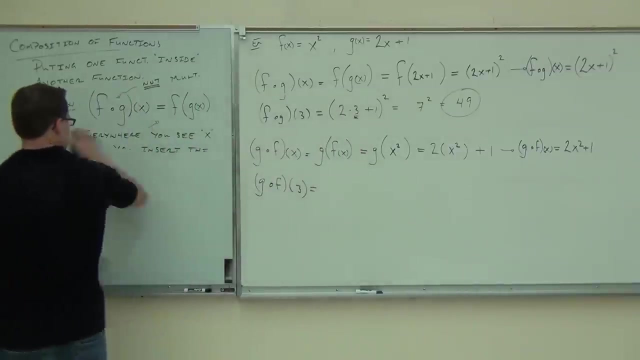 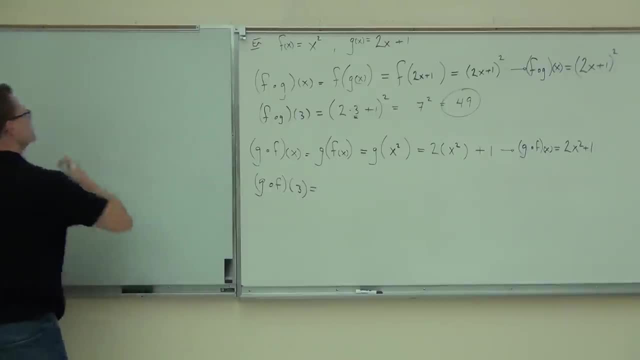 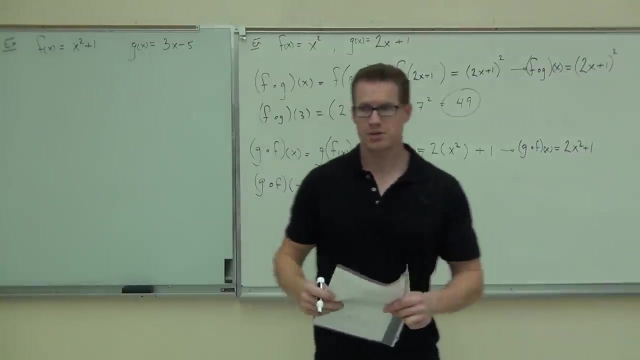 It's 2.. b squared is 9 times 3 is 18,. 19 plus 1 is 3. 5 is 18.. If you want to get a jump start, if you've already done that, I want you to find. 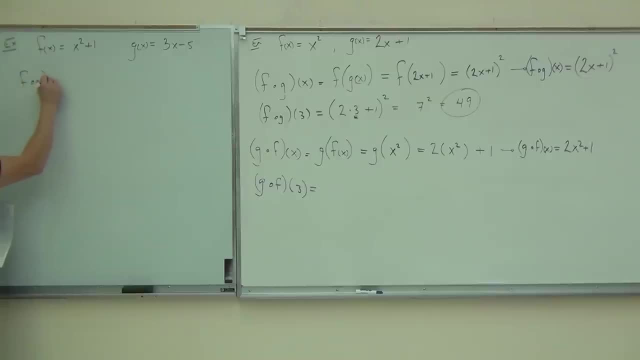 f of g of x. I want you to find g of f of x. After you do those two things, remember this comes first, always. I want you to find f of g of: oh, let's see here, let's do four. 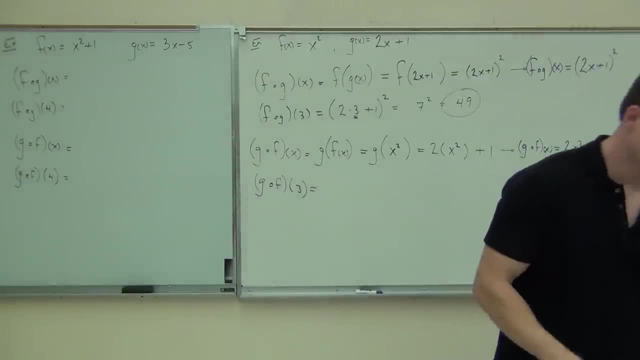 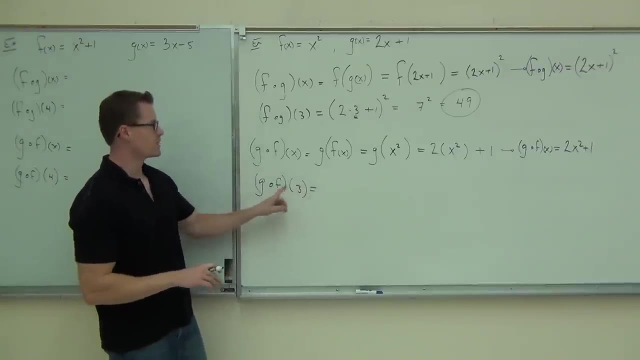 And g of f of four. Okay, before you start, y'all should be done with this one. Let's go ahead and do this. g of f of three says you're gonna go back up to g of f of x. You're gonna look at the very end. 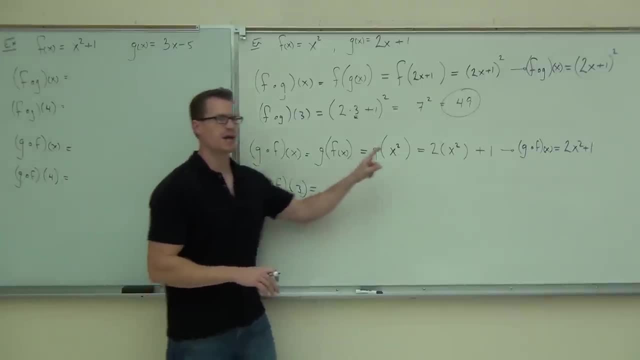 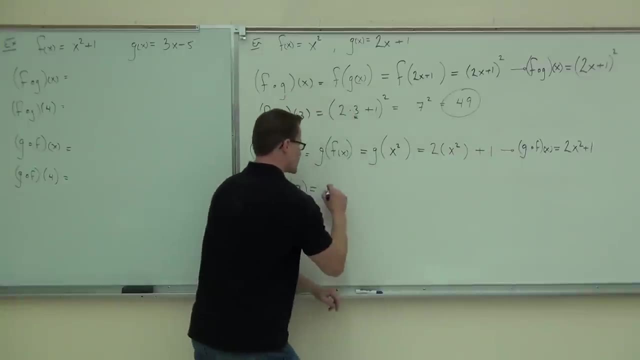 to the expression that you got at the end. That's two x squared plus one. What number are you plugging in Three? Just plug in three. That means two times three squared. That's where that three's going is into that expression. 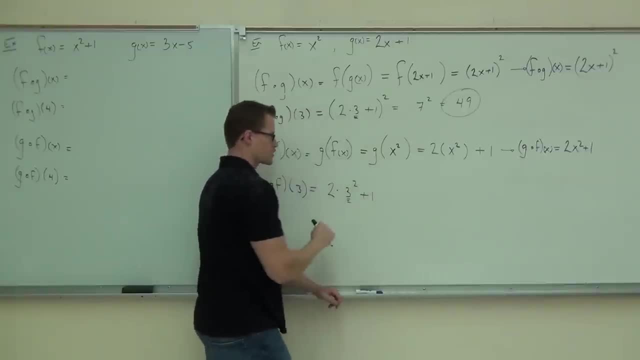 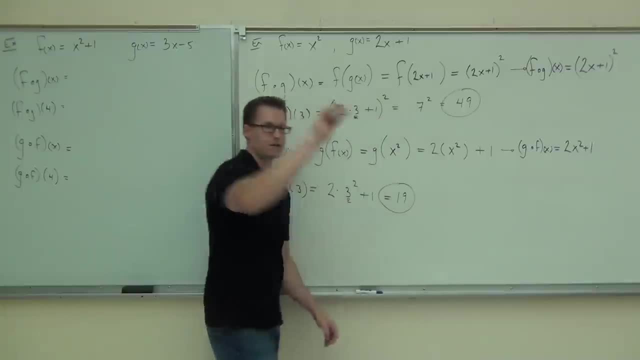 Nineteen, Nineteen, Nineteen, Good, good. So on this problem which I'm gonna have you do right now, I'll give you about a minute to do it, Maybe two minutes. Which ones are you gonna do first? 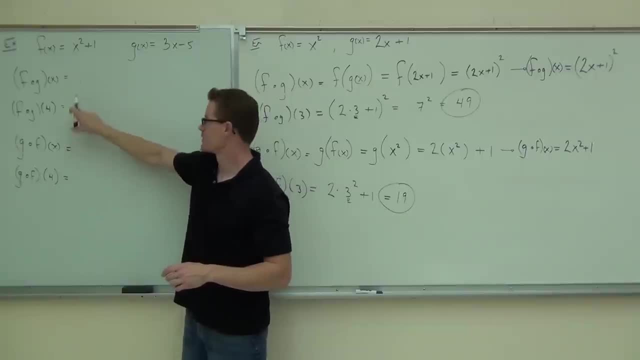 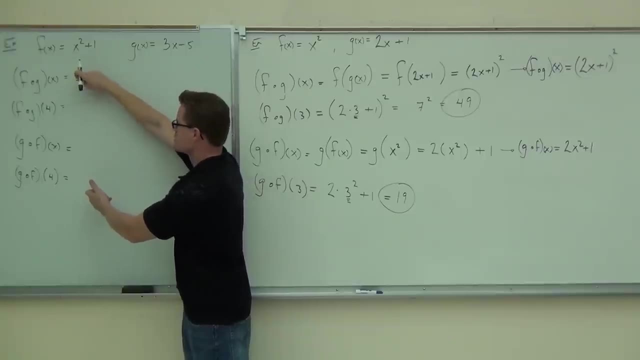 The first and second one, or the first and third one, First and third. Well, you're not gonna do these ones first, are you? That's not gonna work. You could do the first two first if you wanted to, but make sure you do this one before this one. 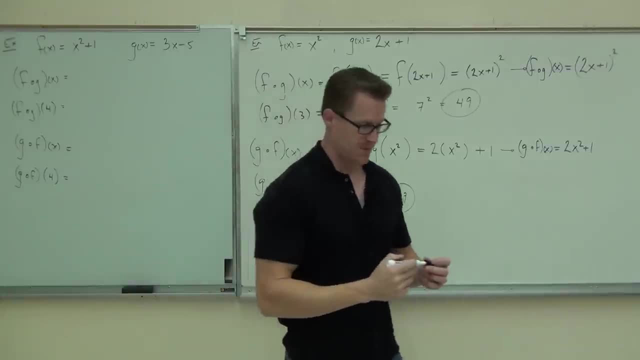 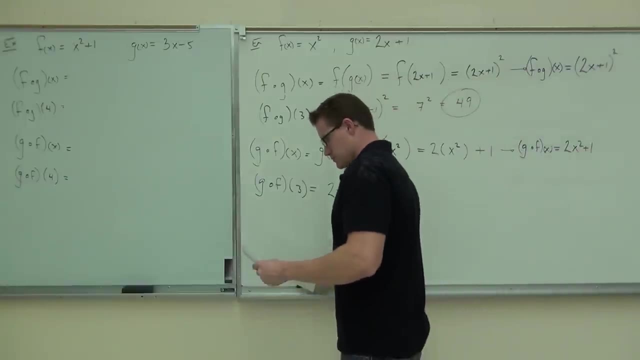 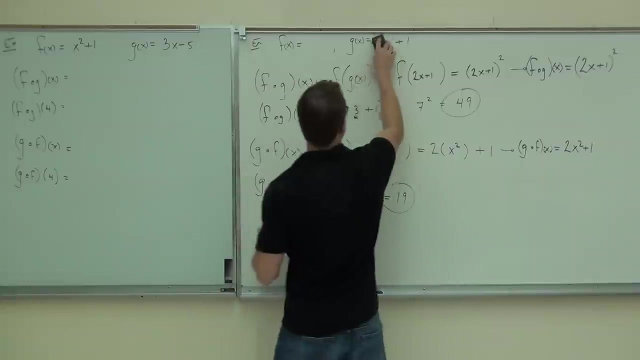 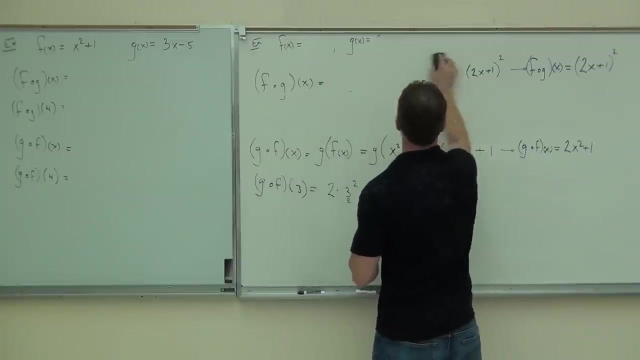 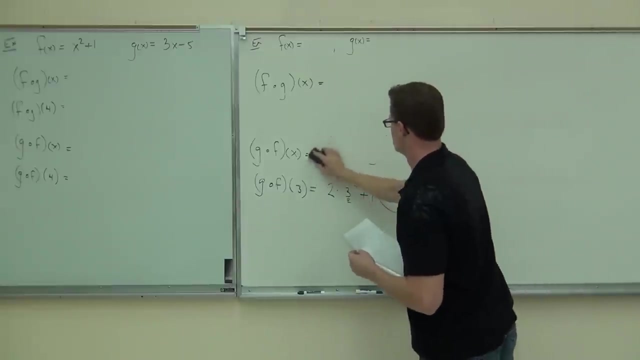 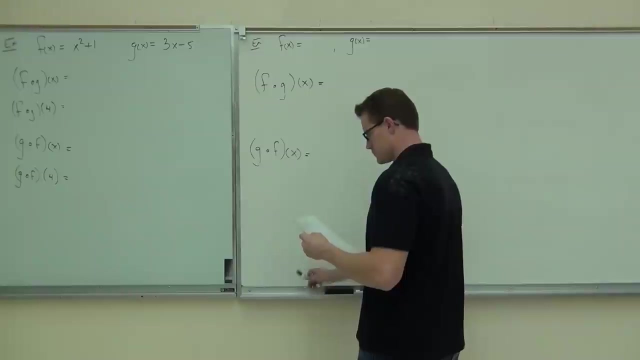 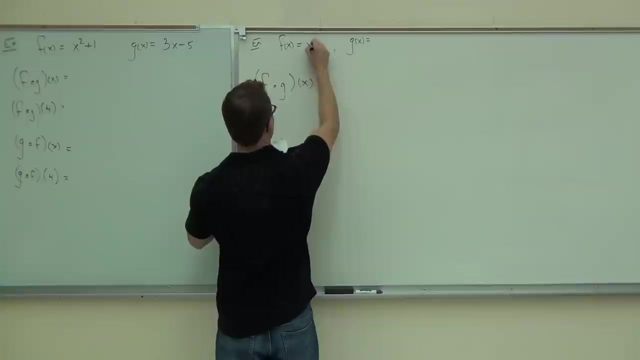 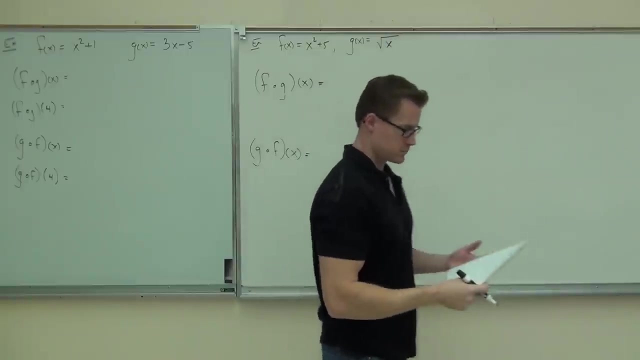 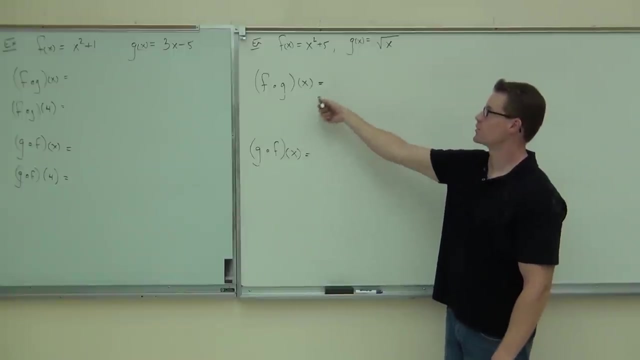 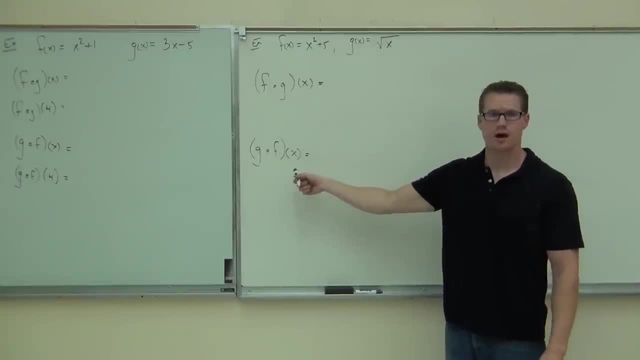 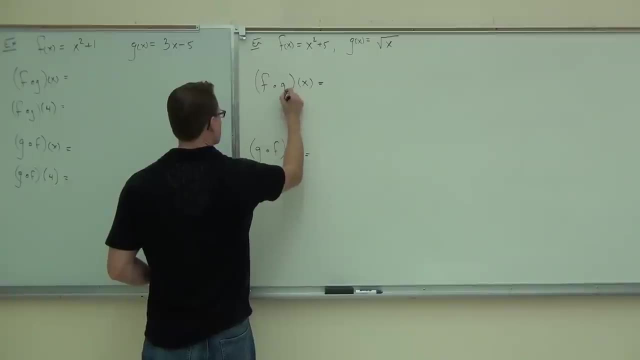 We're gonna do f of g of x and g of f of x together in just a moment. I don't want any. no, you don't plug it in numbers. I don't want any numbers. I'll be walking around. If you need help, let me know. 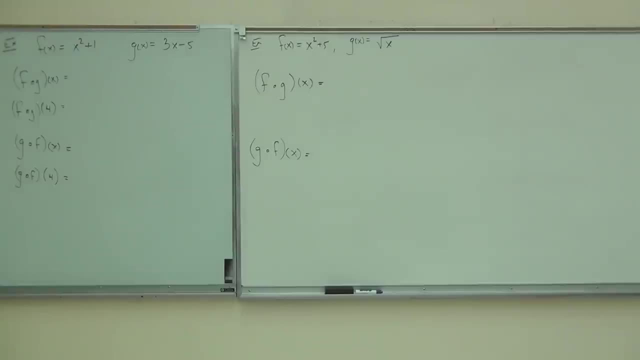 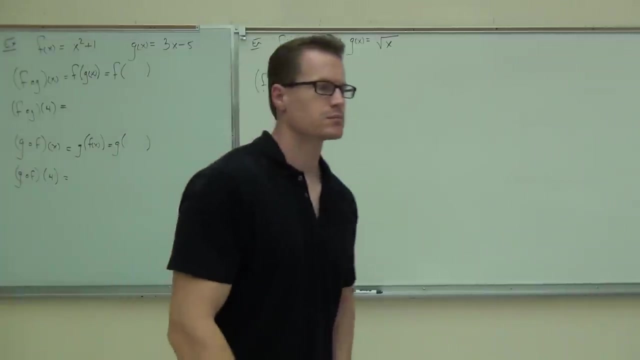 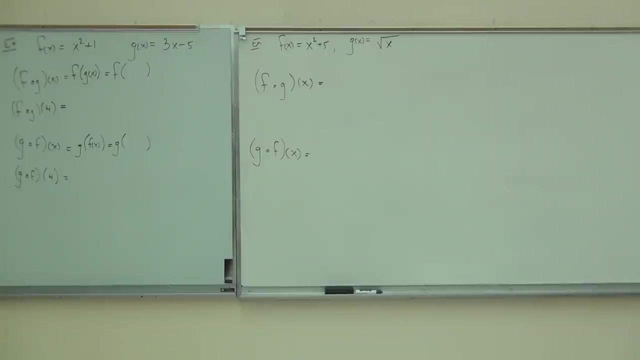 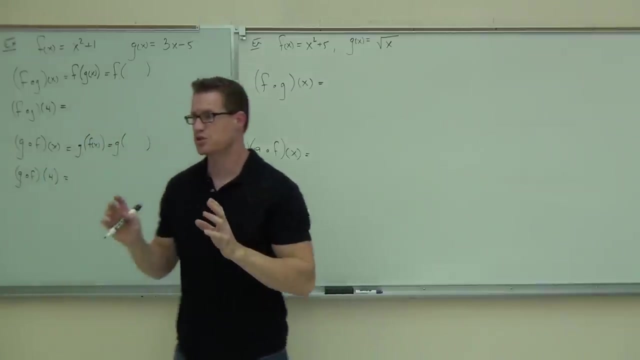 It's kind of an important concept for you moving on. All right, let's start again. Thank you, Thank you. Okay, I'm going to make sure that you got these things right before you do these things. Of course, these are the items that you need to do first, the compositions, with just the 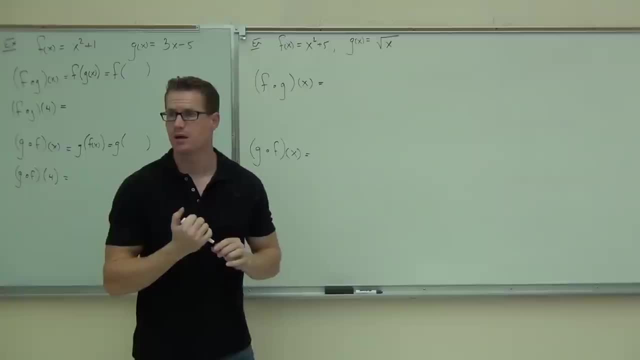 x variable. That way you can do it, That way you can plug in the number later and it's way easier. Are you with me on that? So let's go ahead and see if you got this done correctly. So can you all tell me what goes inside this particular parenthesis? 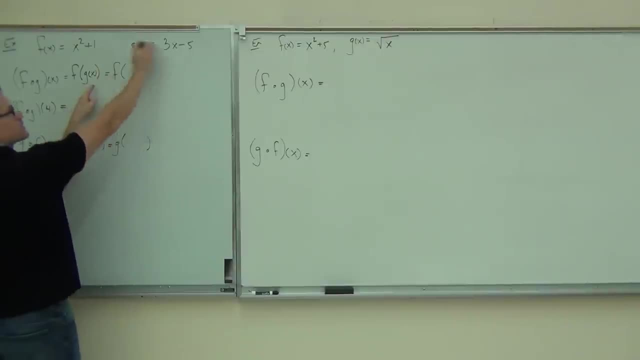 3x minus 5.. Good, That's referring back to g of x, 3x minus 5.. The only letter left on our problem is f. So you're looking back at f. You're reading that in your head or reading it aloud. 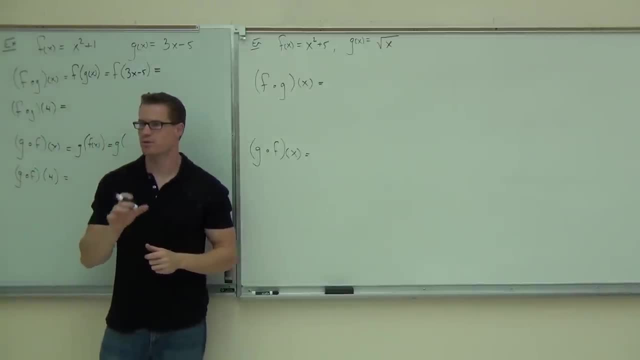 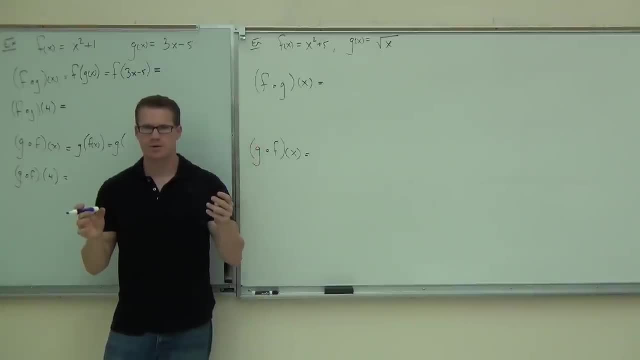 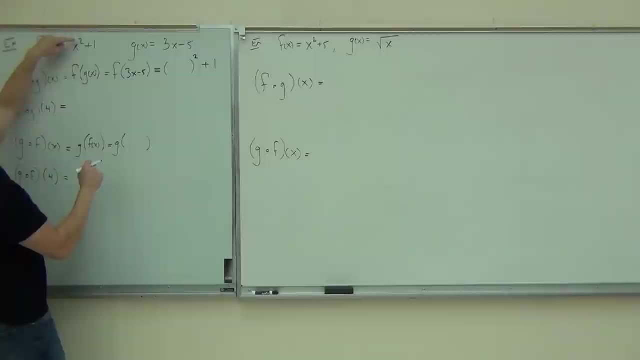 Did you write parenthesis squared plus 1?? Yes, I see where that's coming from: Parenthesis squared, parenthesis squared plus 1.. Why am I going to f? Why am I going there? Because you've got to write the f function out. 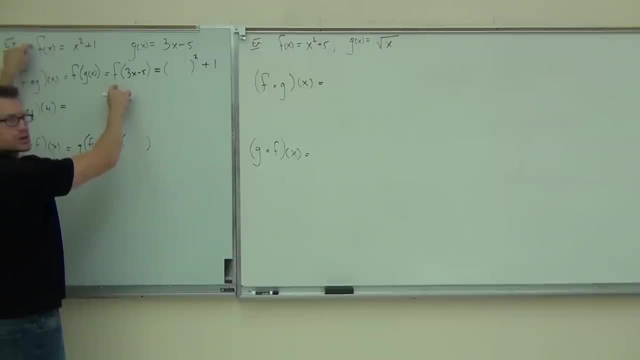 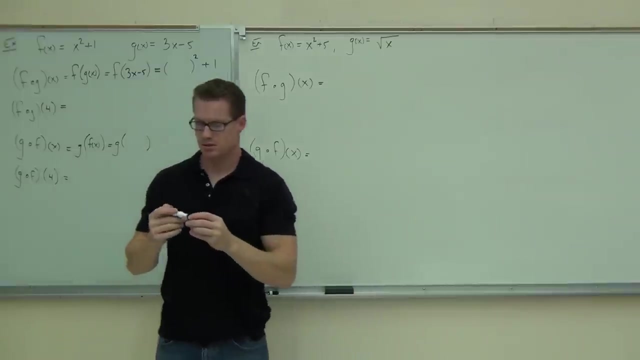 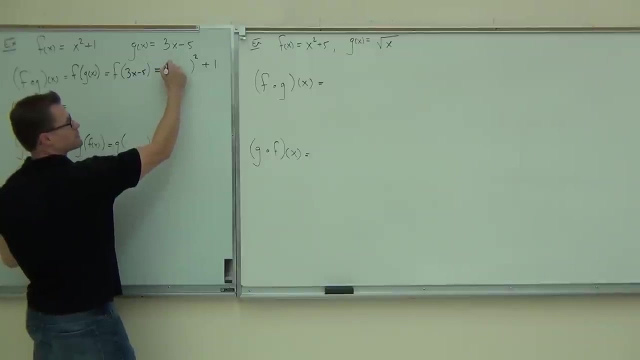 Because it says f. Yeah, It says f, We're looking at those two things. So you're looking here. f says parenthesis squared plus 1.. I've written that out. What goes inside that parenthesis? What was it? Whatever's in this parenthesis goes in, whatever parenthesis you have left. 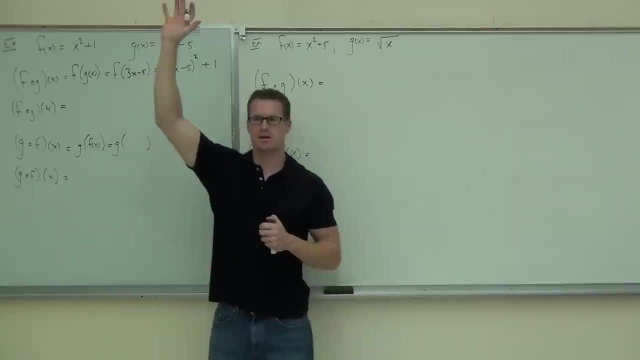 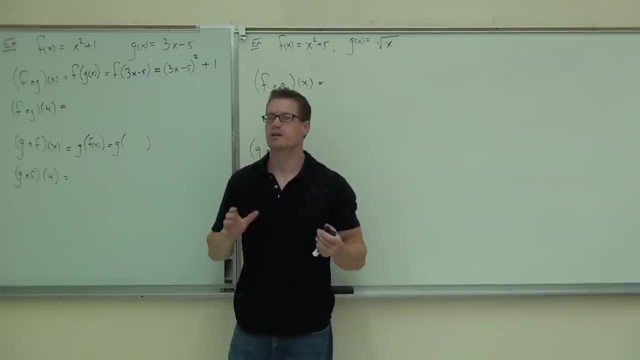 I want to see how many people got that one right. If you didn't raise your hand, you didn't get it right. right, Okay, that's fine. If you didn't, where did you make a mistake? If it's plugging in the wrong function here, you need to really watch that. 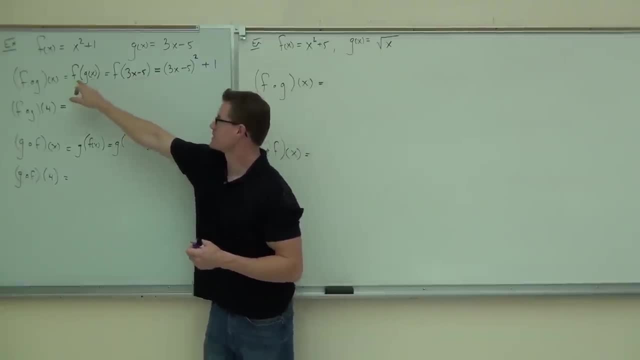 Okay, You need to look here and get that function. I mean, this is f of g of x. This should be f of g of x. It's the same exact thing. You just got to refer back to the correct function and put it here. 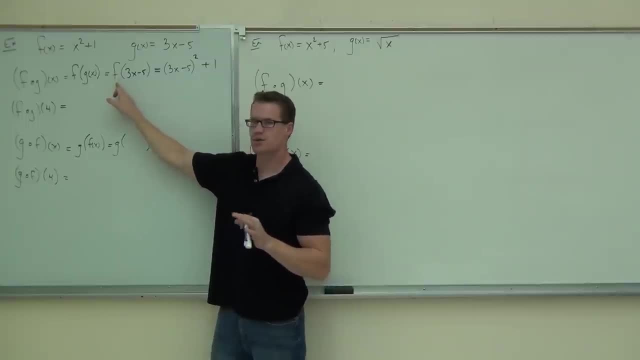 The letter that's remaining. that's telling you what to write out next. So you should be using. typically, you'll be using both functions somewhere. If you use the same function twice, you've done it wrong. You should be using both these things. 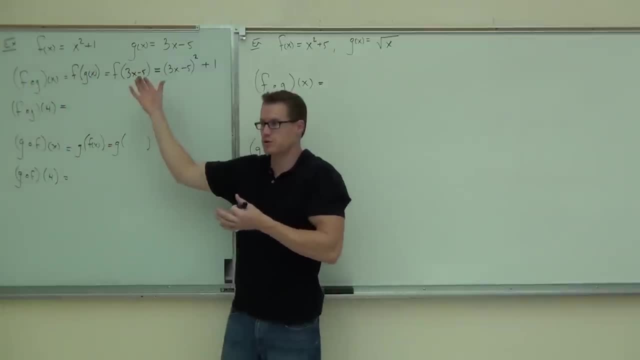 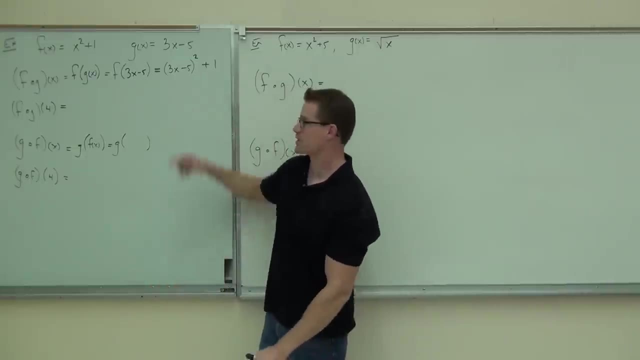 If it's asking for two different functions, of course you're going to be using both functions there. Now you can choose to distribute that if you want to, and combine like terms or leave it. I really don't care, I prefer to see that one. 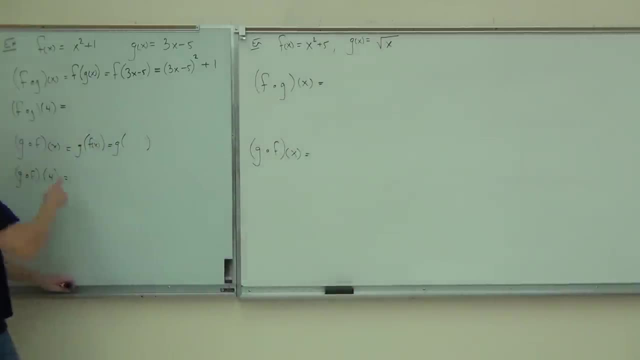 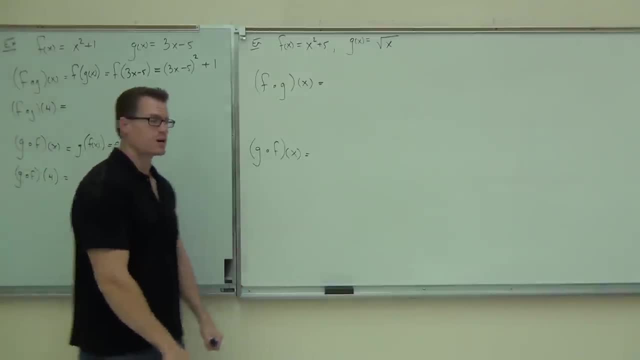 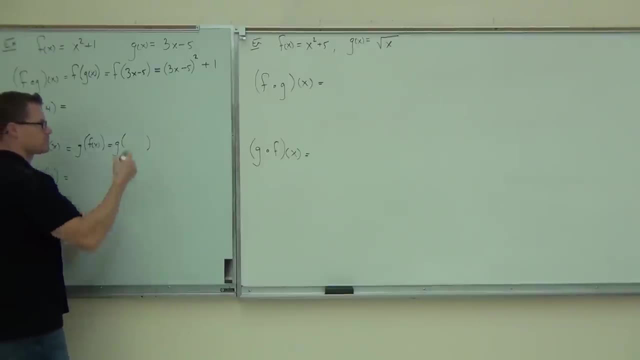 I don't know Now, how about g of f, of x? Let's go ahead and practice this one. Can you all tell me, what function should I be looking at for this one? What is it? x squared and then just x squared. 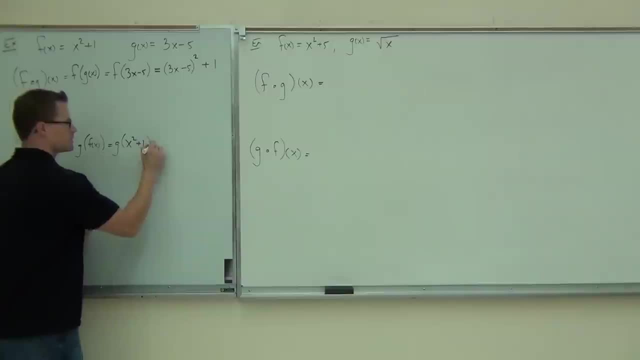 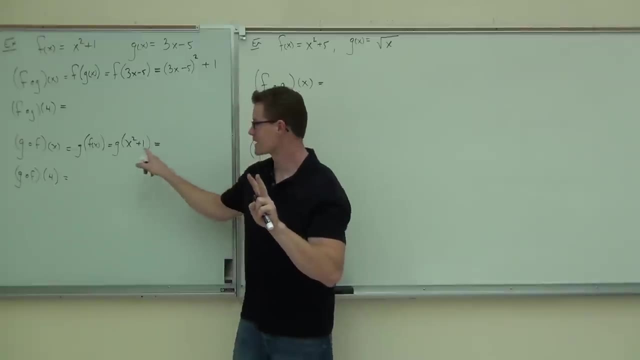 I'll try this one. I'll try this one. Okay, Good Equals. Are you okay with that step? Yep, That was the second most important step. The most important step is the next one. The second most important step. you should have g of that function. 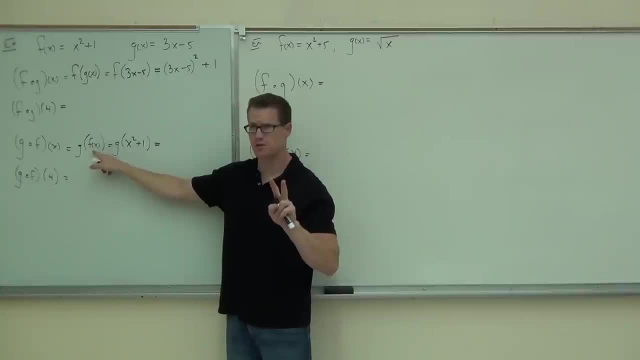 That function is x squared plus 1 in this case. So x squared plus 1 goes right here. Take a moment to look at the board. Are you okay with it? honestly Okay, Good, Now, what function are you supposed to look at? 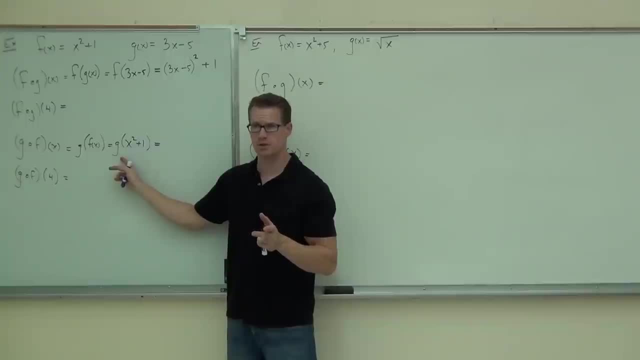 G, G- That's the only letter left that represents a function. What does g say? 3x minus 5.. 3x minus 5.. Good, Now, that's supposed to be 3.. Parentheses minus 5.. 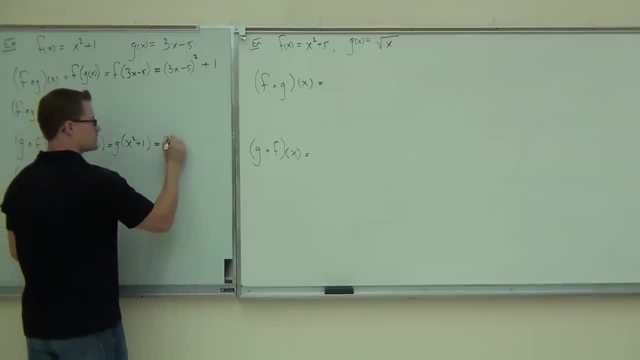 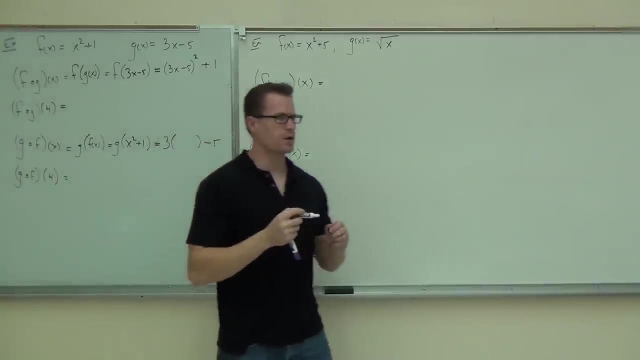 That's exactly what you write: Three parentheses minus 5.. Are you okay with that? Are you okay with that step- That's the most important one- is looking at the correct function and writing it appropriately. So this says you're looking at g. It's the only letter left. 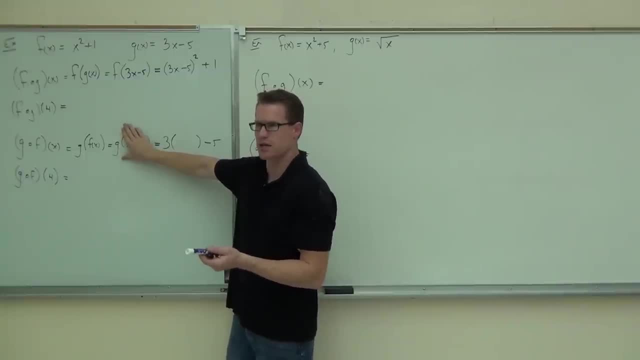 This is this you're going to ignore for just a second. Just ignore that for a second. Look back at that function. That says g, three parentheses minus 5.. We wrote that out. Now you just got to translate this parentheses into this parentheses. 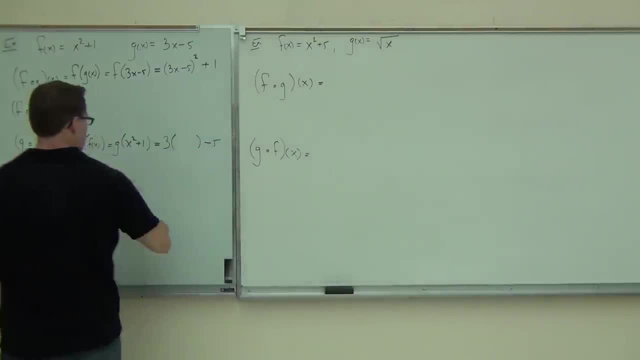 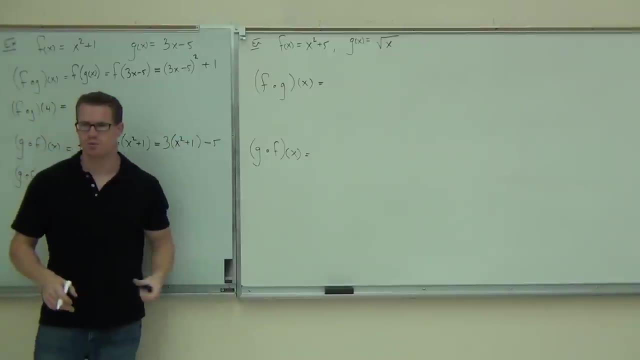 Just replace it. What goes in there Excerpt. Now you can probably distribute that one a little bit easier than that one, right? So go ahead and do that if you want to. Otherwise you can leave it, but it's probably going to be a little bit easier. 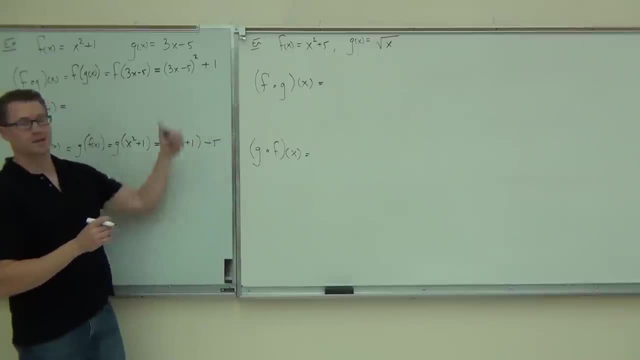 to plug a number into this next thing I'm going to write than this one Here. it really doesn't matter. So we're going to do 3x squared plus 3 minus 5.. You see where that's coming from, I hope. 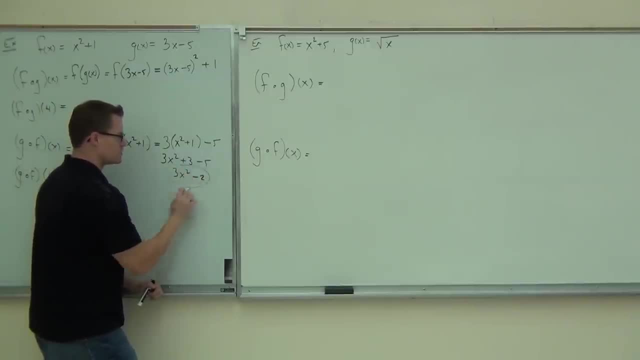 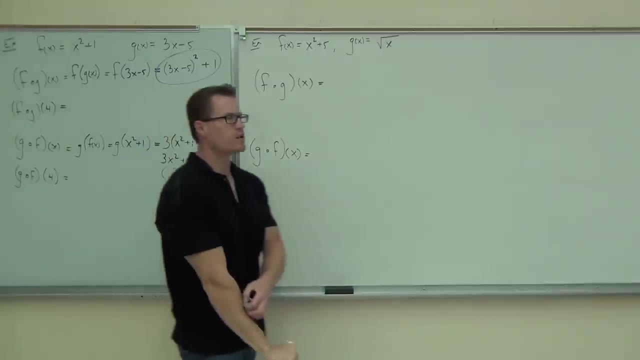 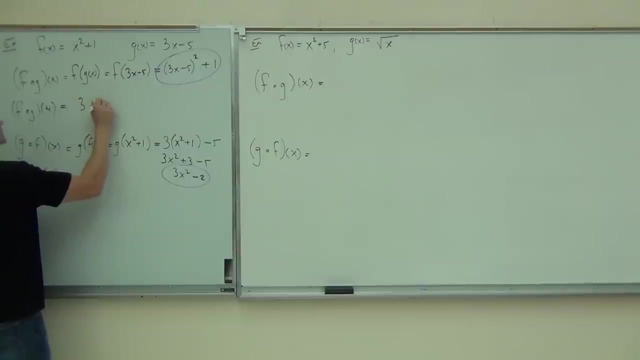 That's 3x squared minus 2.. Now, what's the 4? have you do? What's this one mean? Plug it into? Plug it into this one. No, this is the one that says f of g. Now just take that. plug into 4, so we're going to get 3 times 4 minus 5 all squared. 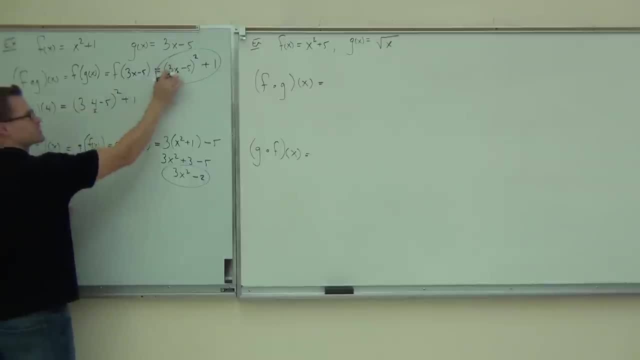 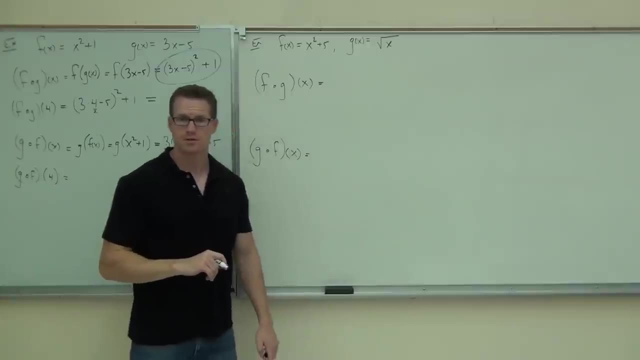 and then plus 1.. We're just taking that value of 4 and inserting it into the function that you just figured out. How much is that all going to be, please? Seven, Seven, No, it's 49. 49?. 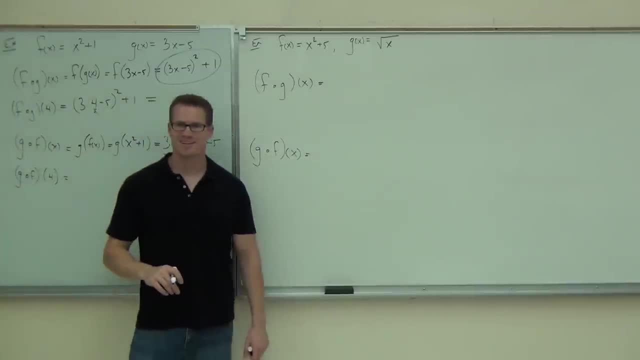 50.. 50.. 50?? It ends up being 50.. 49 plus 1 is 50.. Sorry, It's okay, It's all. good, It's early, It's the only one. 12 minus 5 is 7.. 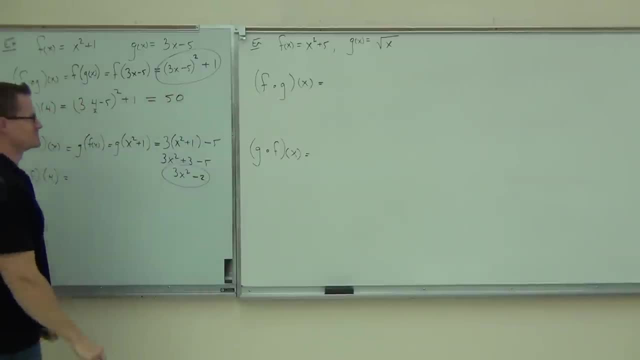 40. Okay, 50. Cool, Did you get 50? Yeah. Next one says: take that 4, insert it into this function. That's 3.. Either way, it's going to work out correct for you, okay, whatever form you leave in. 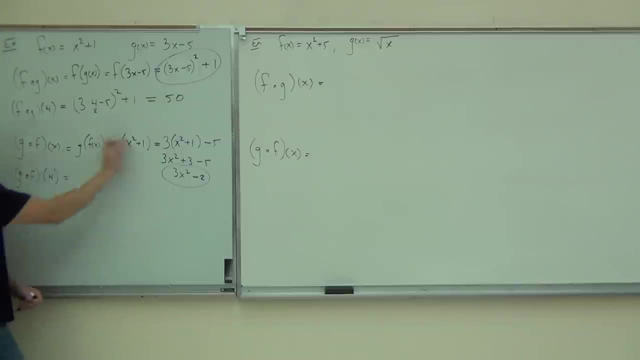 3 times 4, squared minus 2,, how much do you get out of that? 46.. 46.. That's the idea. Can you handle the idea? Yeah, We're going to try a couple more. really, really quick. 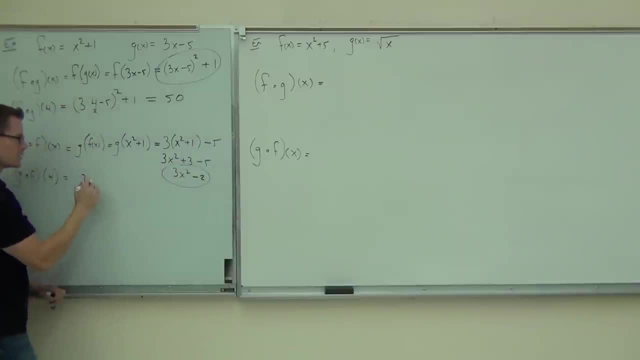 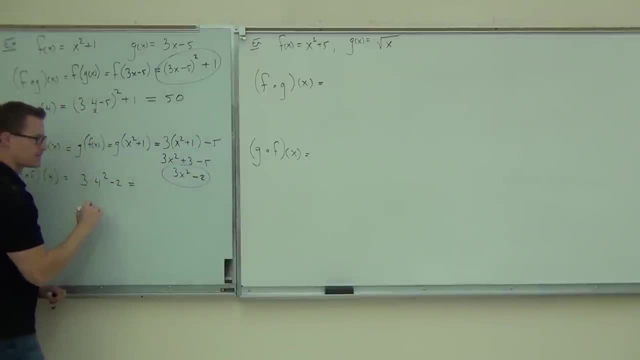 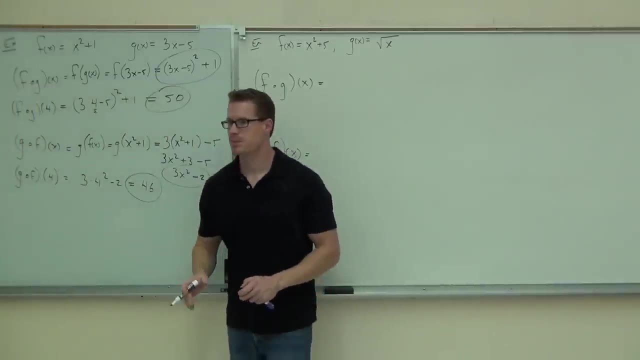 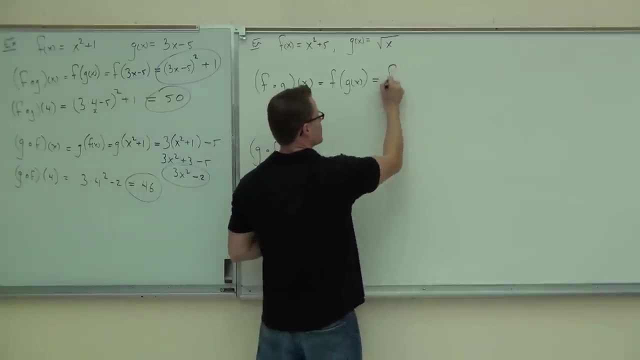 So you see a couple different scenarios here. If we want f of g of x in this case again, I'm going to move kind of quick on these examples- We already covered the main issues. We're going to have f of inside the parentheses will be: 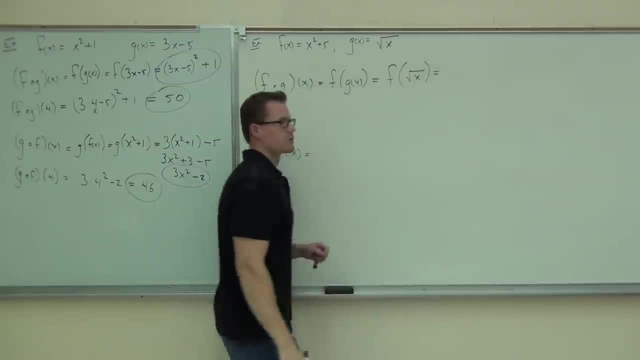 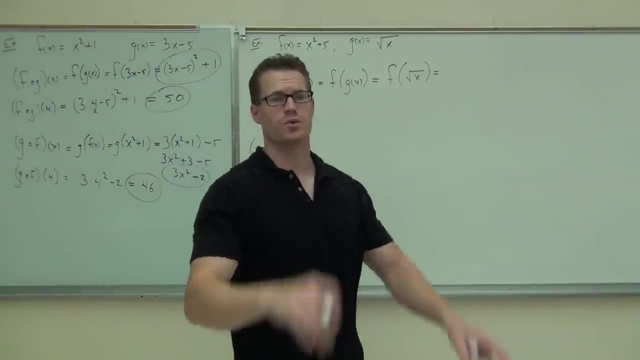 Squared by 3.. Good, We look back at the original function F. F says X squared plus 5.. You see that. So, instead of X squared plus 5, folks, what are you going to put? Come on, say it out. 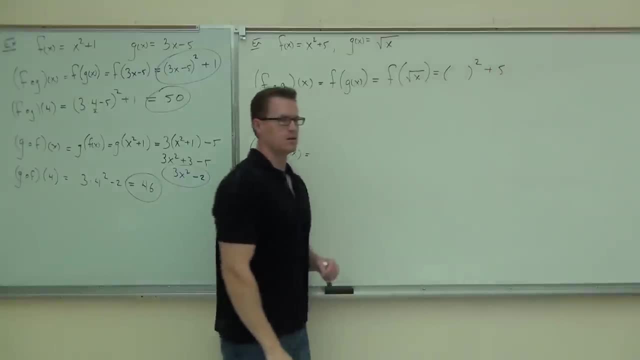 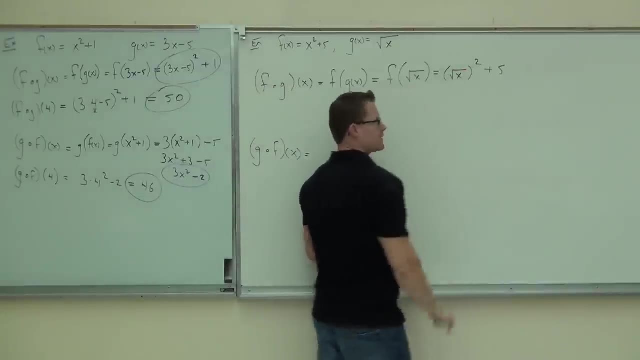 Parentheses squared. Okay, good, I like it. Are you okay with that? Look back at that F. What goes inside that parentheses? Now here's something interesting that can happen when you compose functions. Firstly, how many people feel okay getting that far? 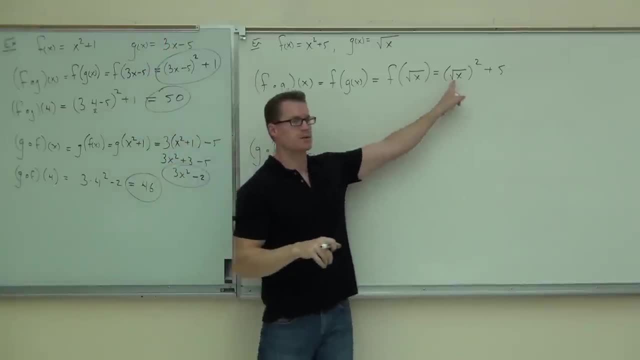 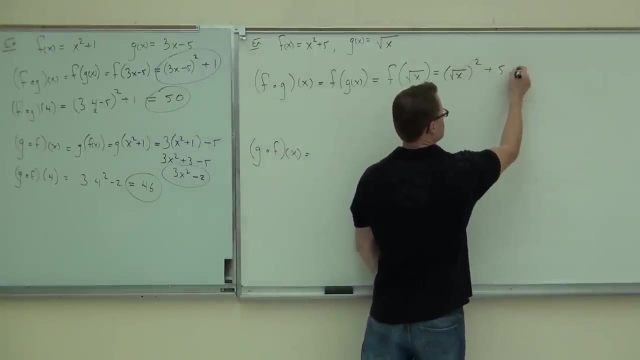 I went fast, but we should be able to handle that. What happens? That's interesting, isn't it? Sometimes, when you compose functions, that can happen Square over square root. that's going to give you X plus 5.. That's your composition, just X plus 5.. 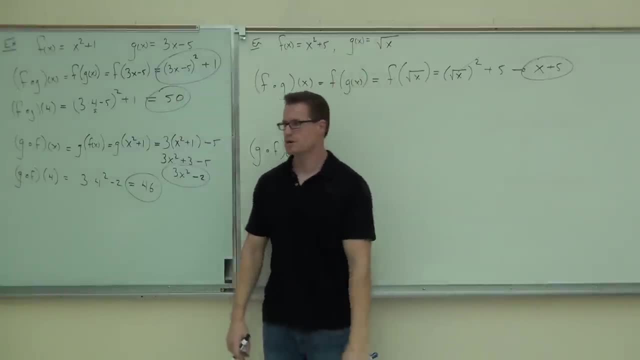 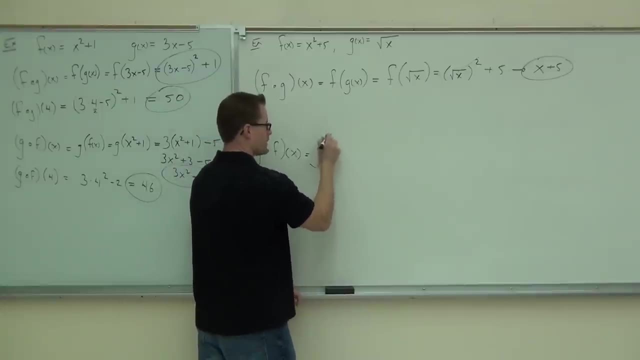 So all this stuff reduces down, when you compose it, X plus 5.. Kind of neat. Let's do it the other way, see if it works out the same. Here we're going to have G of F of X. Of course that's going to be G of what's inside the parentheses. 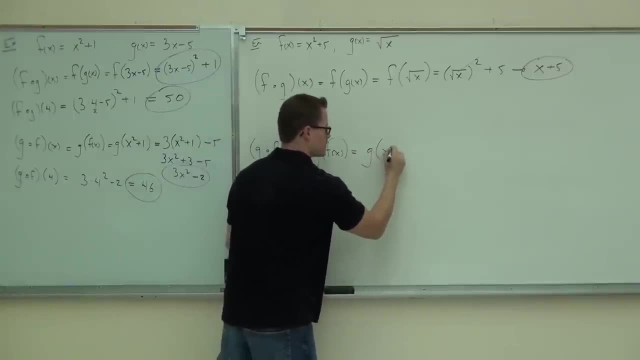 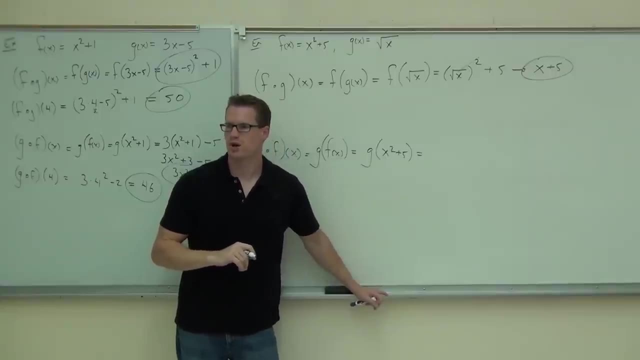 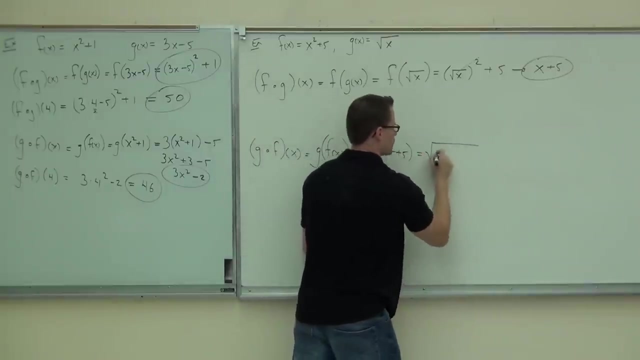 In this case, everybody. what's going to go in here, please? Okay, the only letter left on the board is G. What's G? So? square root of Square, root of Square, root of parentheses. Square root of parentheses. 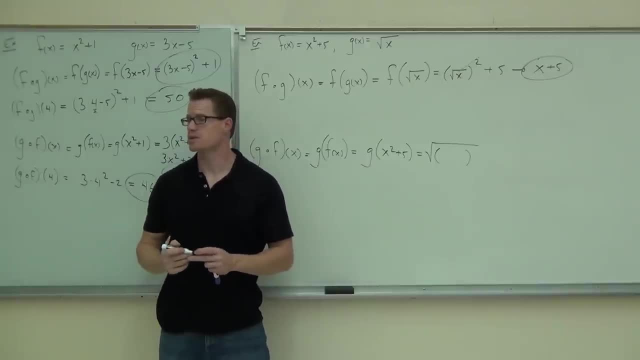 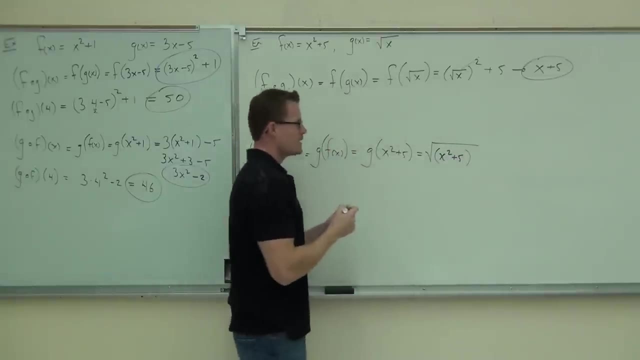 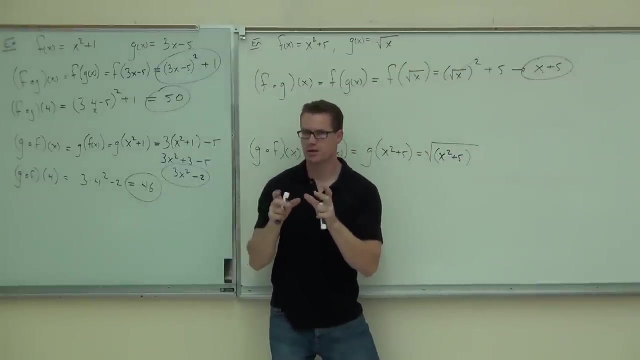 Instead of X, you put a parentheses. What goes in that parentheses? X squared plus 5.. Now this parentheses really doesn't do anything but group this expression together and let you know that the entire thing is underneath that parentheses. Do you see that the entire thing is under that parentheses? 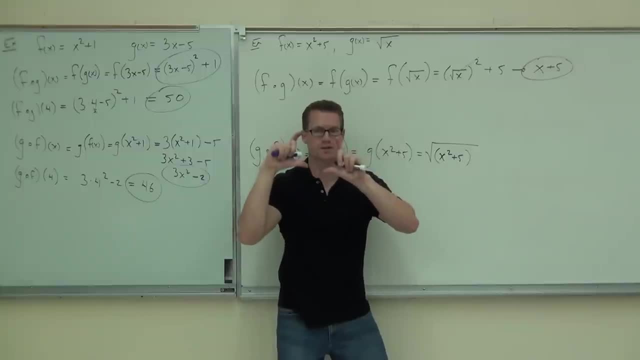 That's why I had you do it this way. so you see that. so you don't put square root of X squared and then plus 5. at the very end We have those parentheses. they're meaningful in your problem, but then at the very end it's not really doing much. 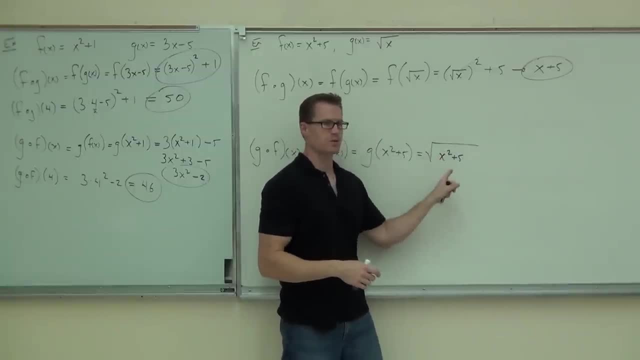 You have the square root of X squared plus 5.. Can you simplify this square and the square root? You can't bring up the X. No, You can't bring up the X because it's combined with that plus. You're done. 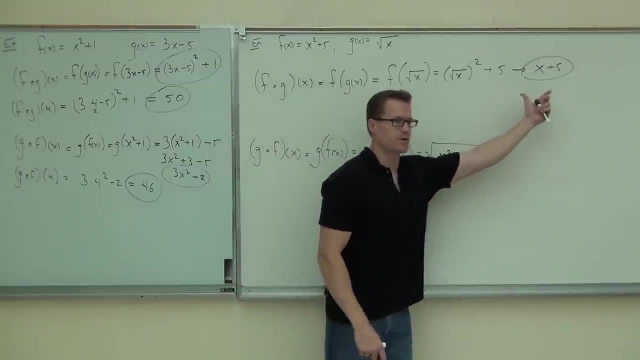 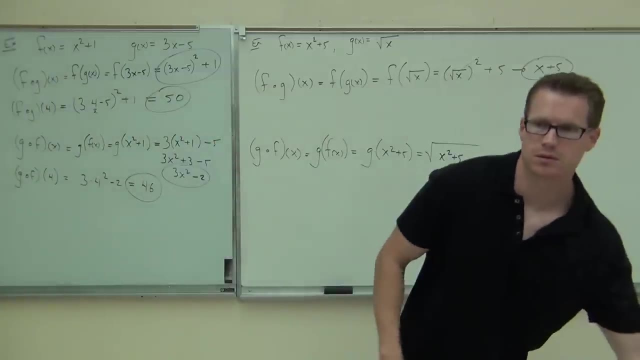 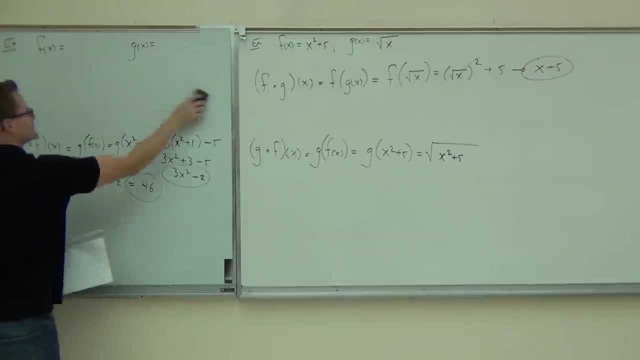 That's all you can do there. So it looks a lot different than that one, a lot different. You ready to try one more example and then we'll call it good, Sure, Okay, How many of us is ready? Awesome, Here we go. 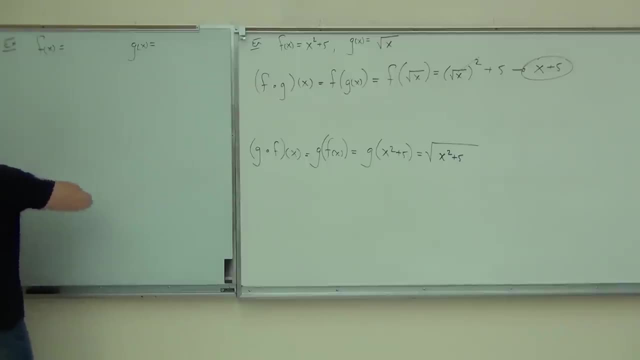 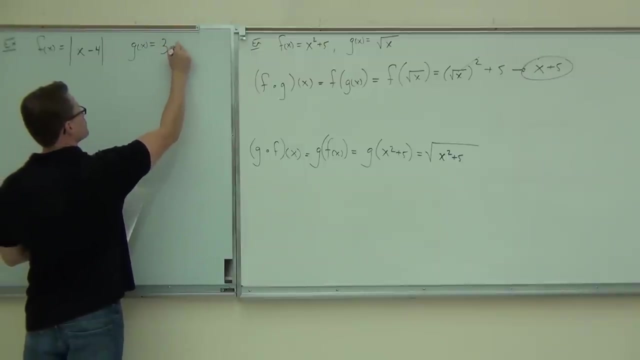 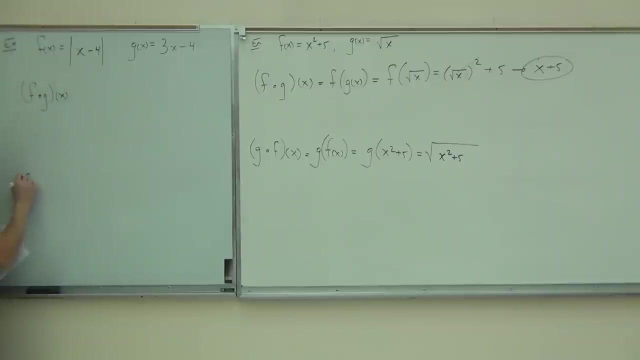 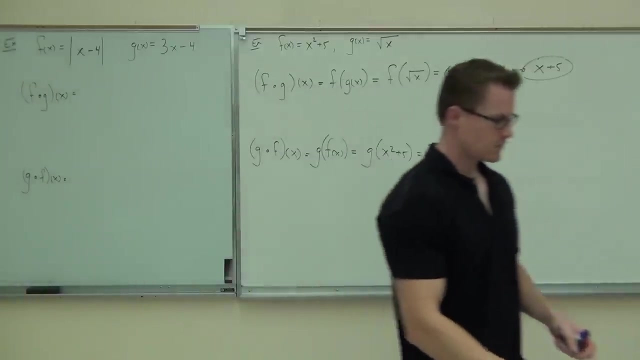 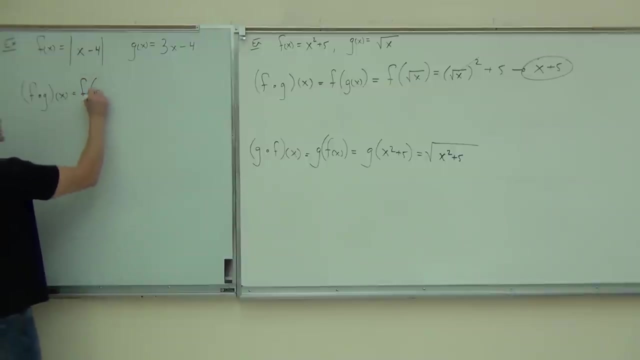 Yeah, F of G of X, G of F of X. So here we are, Here we go. f of g of x written the same exact way. it's said the same exact way: f of. can you please tell me what's going to go inside of my parentheses? 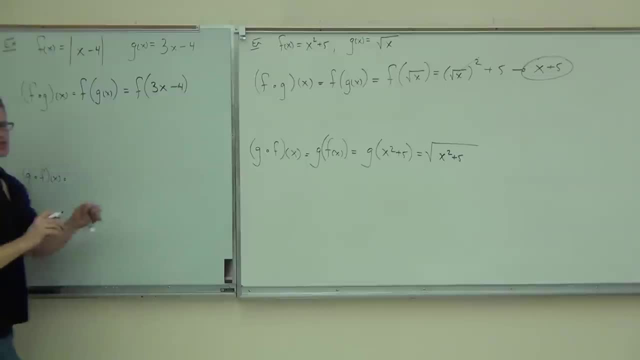 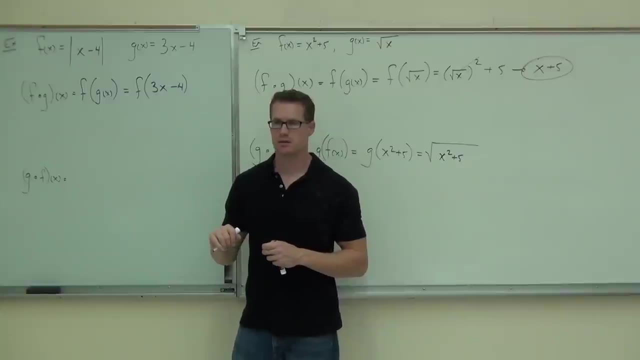 Good. What function do I look back at now? What's the only letter left? So read f to me. The absolute value of x minus x minus 4 is inside the absolute value, right. So read that to me using our parentheses: we're going to have absolute value. what's going to go in there? 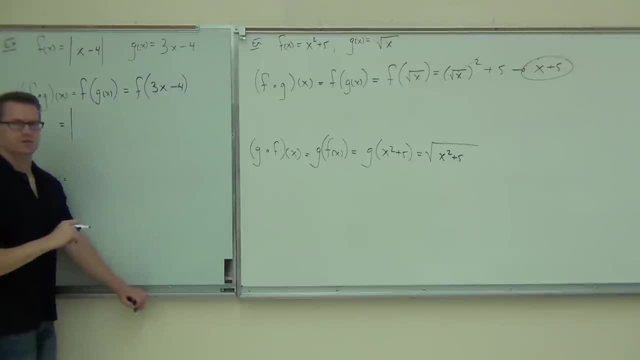 x minus 4.. x minus 4, great. x minus 4, instead of x, you use what Parentheses? Parentheses minus 4.. You, okay with that step. That's the big one, right? That's the big step. you see where it's coming from. 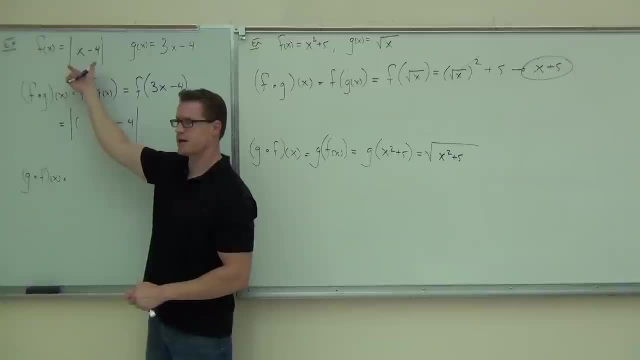 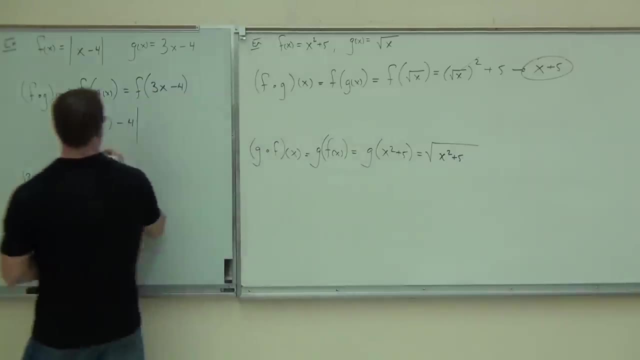 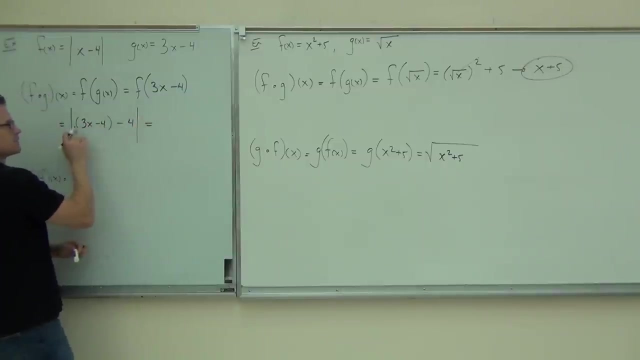 It says f. go back to f. read it in your head: Absolute value of parentheses minus 4, that's what we have. What goes inside there, What have you put there? Now notice, we can do something with this: 3x minus 4 minus 4, that's absolute value of 3x minus 8.. 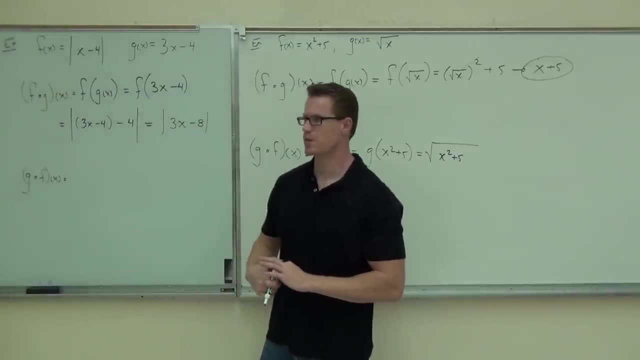 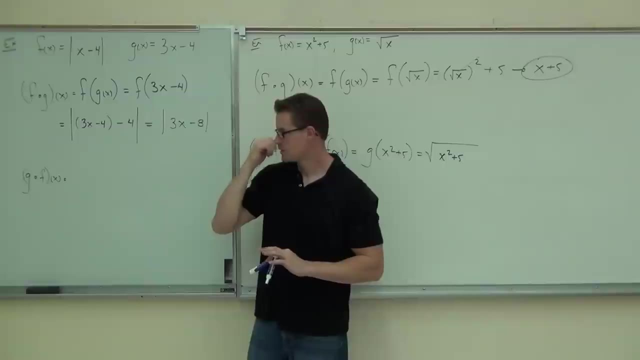 You can't do anything past that, but you're done with that, Done with that problem. See where the minus 4 minus 4, that's giving you that minus 8.. Ready for the last one? Okay, why don't you participate on this thing? 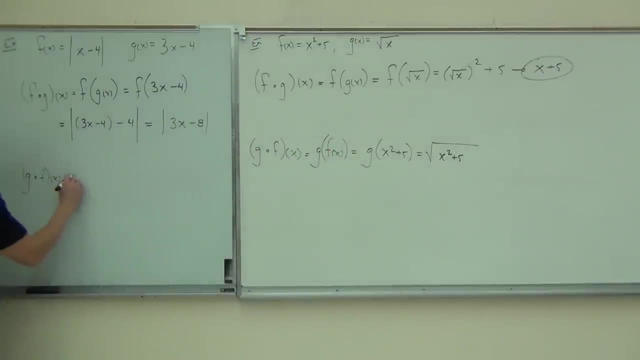 I want you with it. I want you with it. So first thing we write is g of f of x. for sure, What letter remains? the f of the g g? Okay, left hand side of the room. it gets me quiet today. 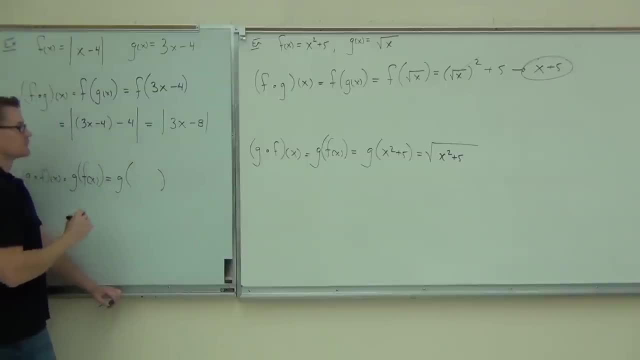 What goes inside my parentheses right here: 3x minus 4.. Be careful. Absolute value of x minus 4.. Why is it different? Why is it different than this one? We're using a different function. We're using a different function, that's right. 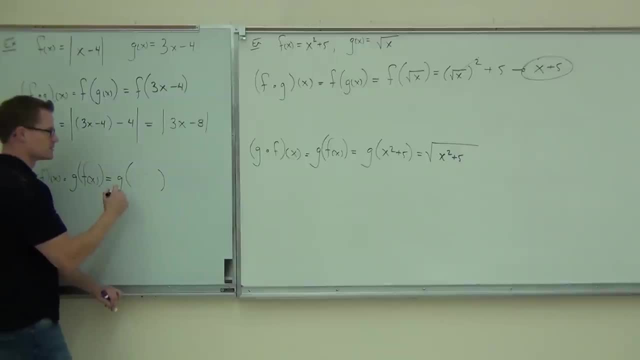 So in this case I'm looking at f of x. What's f of x say Absolute value of x minus 4.. So that's going to go inside of that. Is it easy to get tripped up on these? Yes, 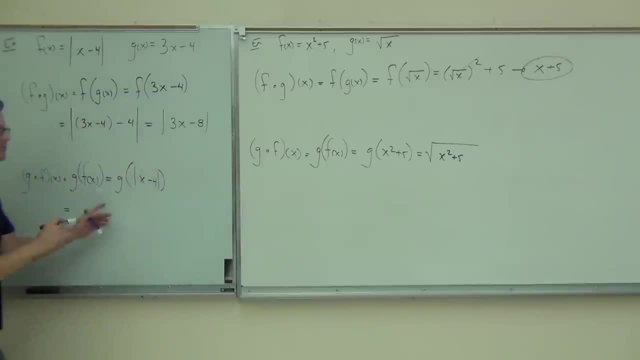 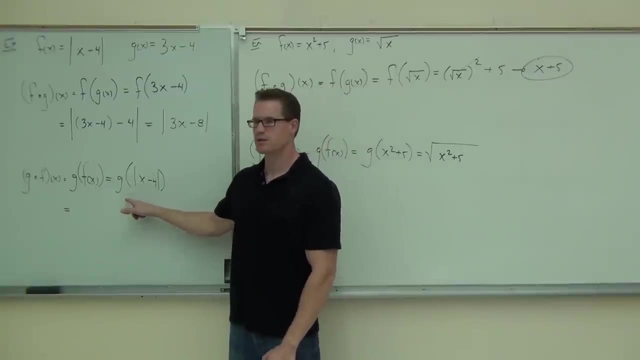 You've got to really be focused on what you're doing here. Now, what function am I looking at? 3x minus 4.. 3x minus 4.. Good, Why? What letter do I have left g? So you read g. 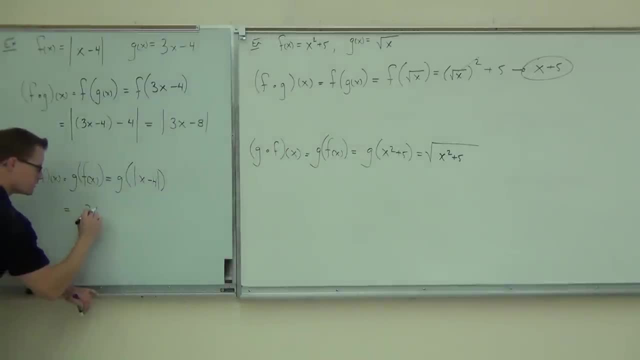 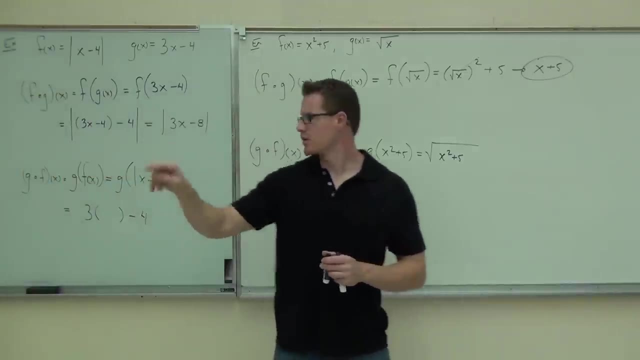 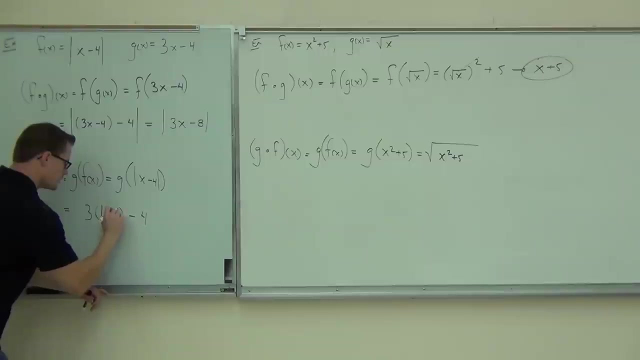 3x minus 4 or 3.. Read it to me: 3, what now? 3x minus 4.. Cool, Can you tell me someone on the right hand side of the room what goes inside this parentheses? Absolute value of x minus 4..